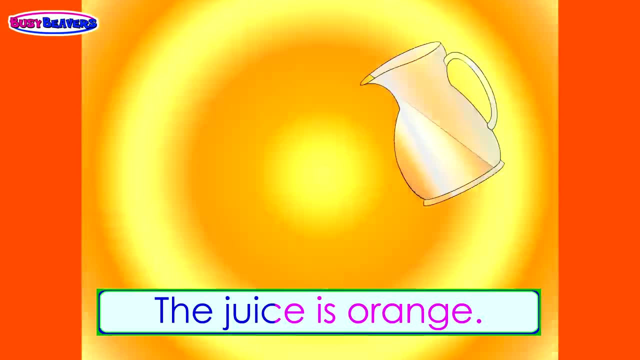 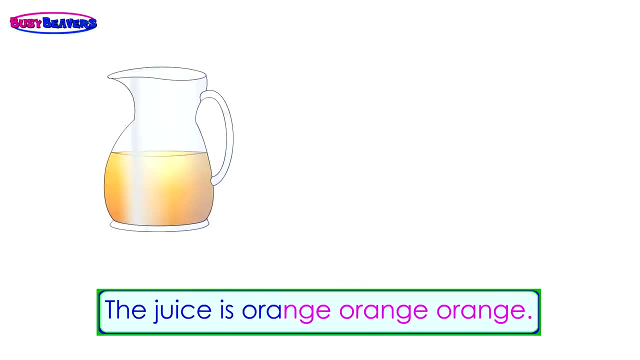 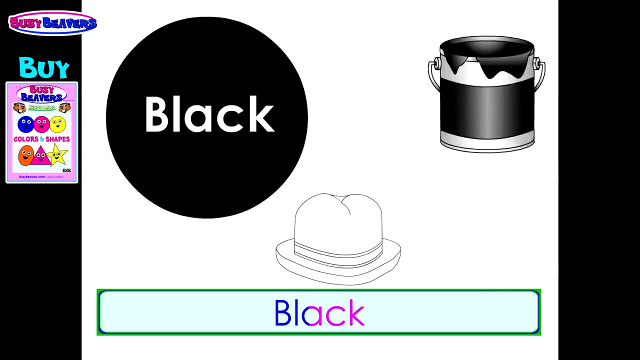 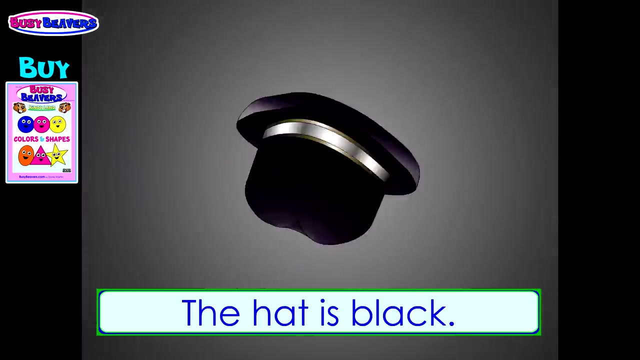 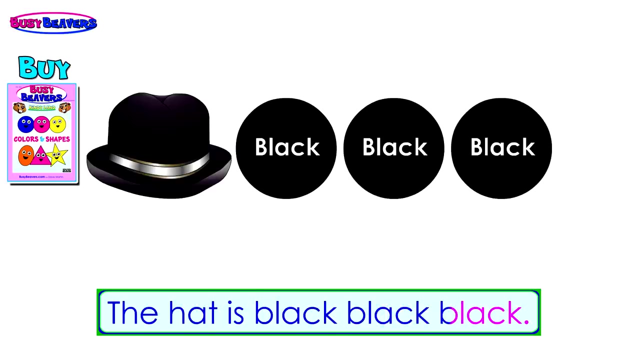 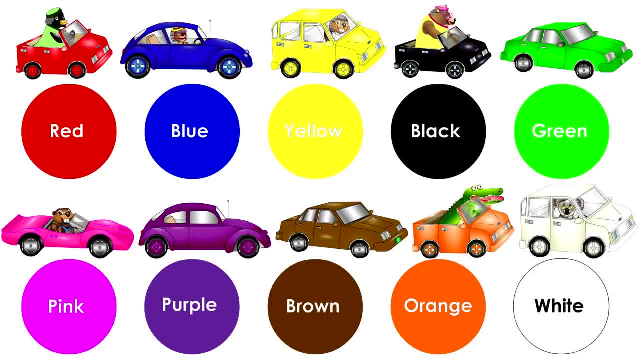 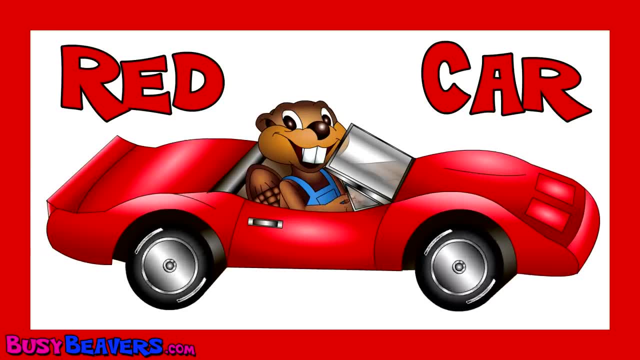 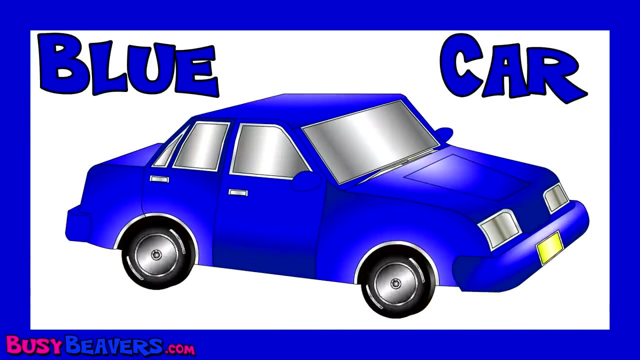 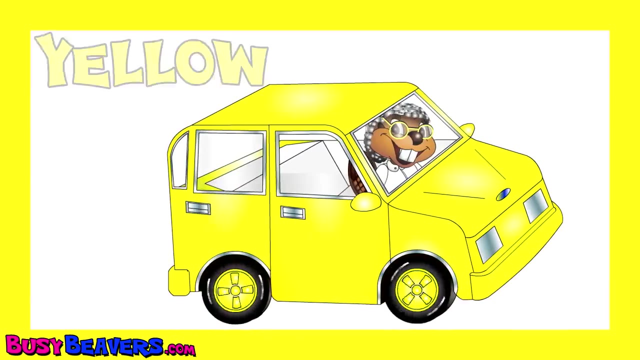 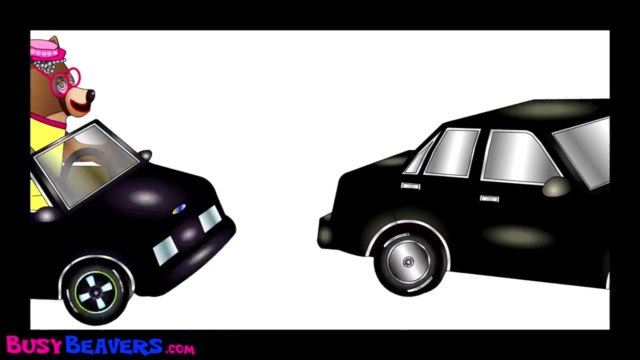 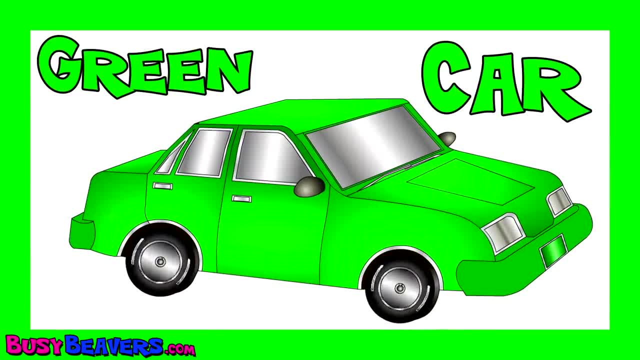 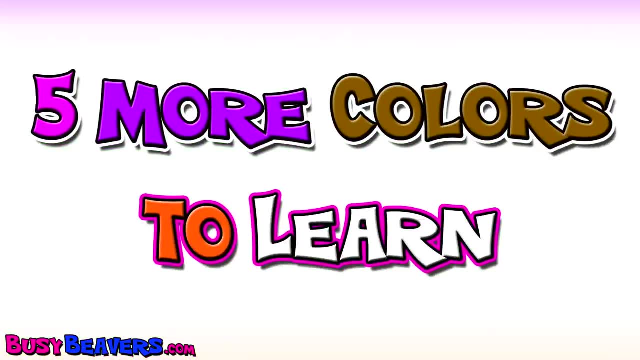 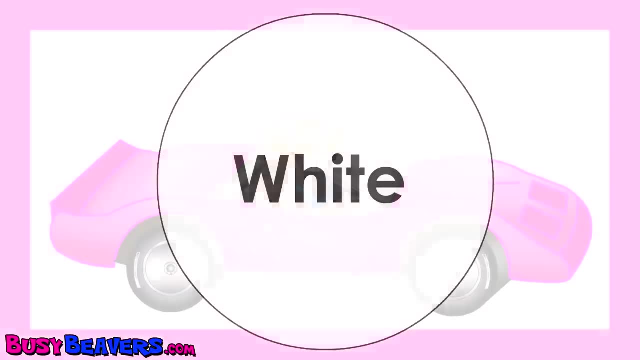 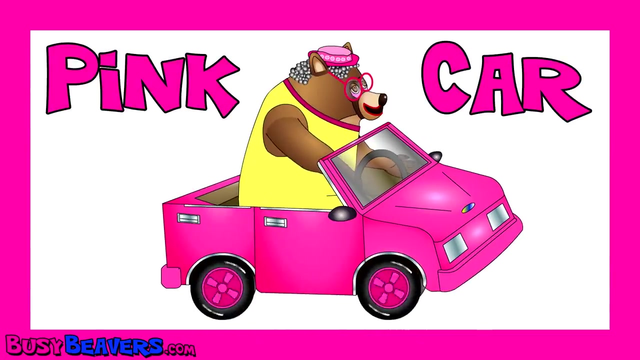 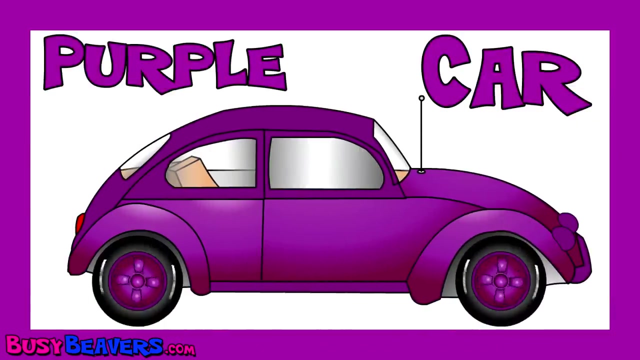 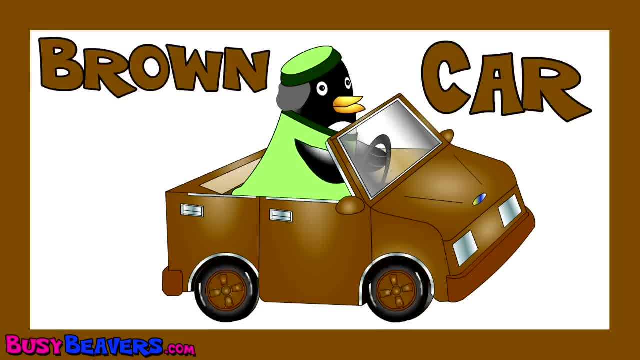 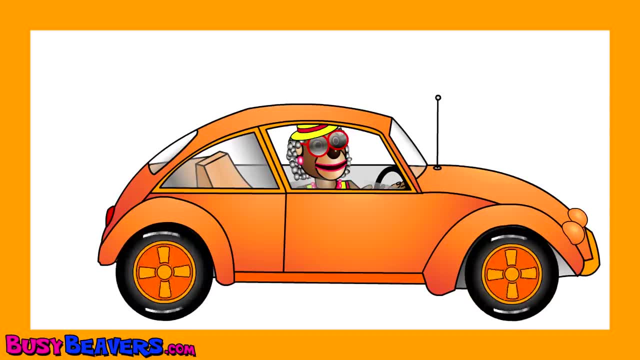 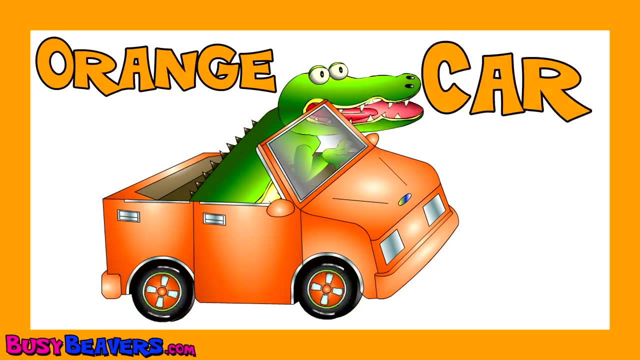 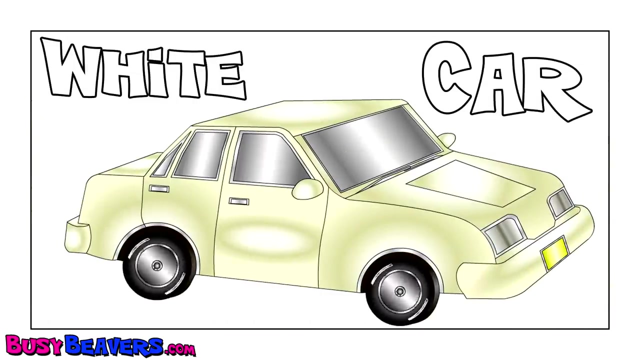 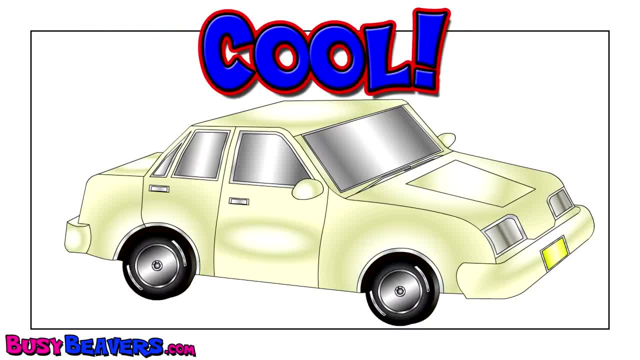 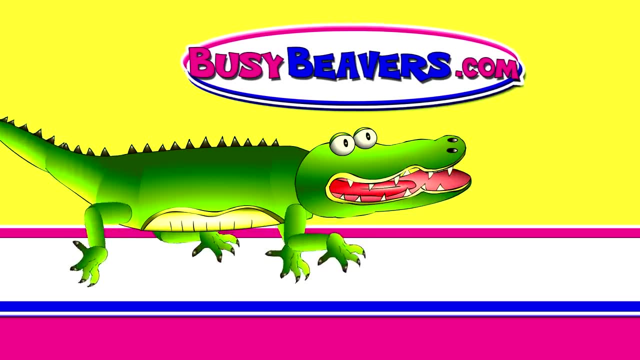 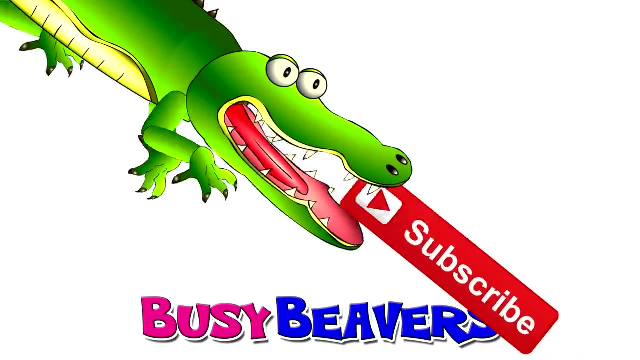 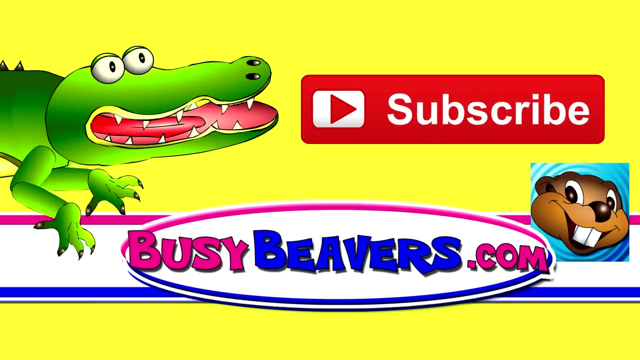 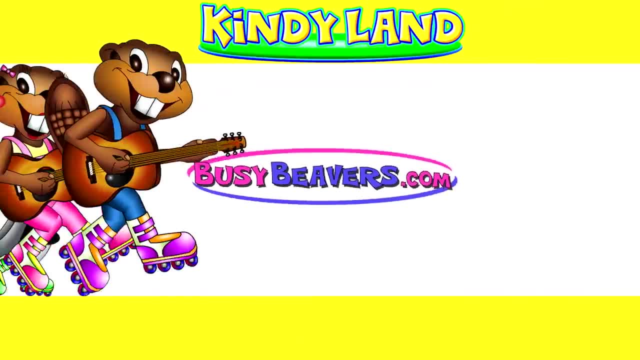 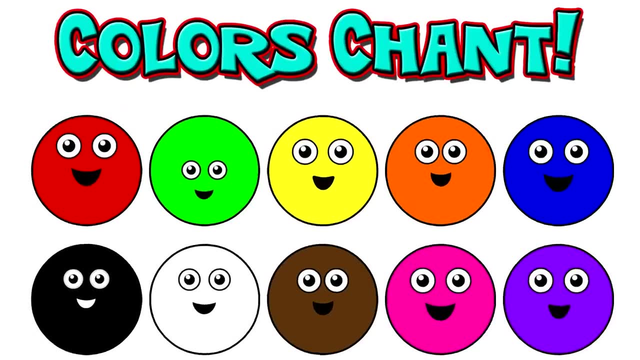 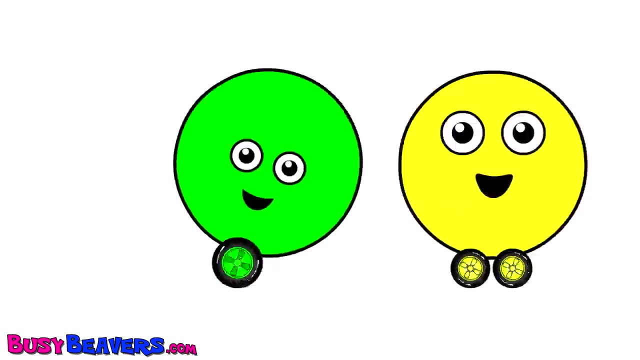 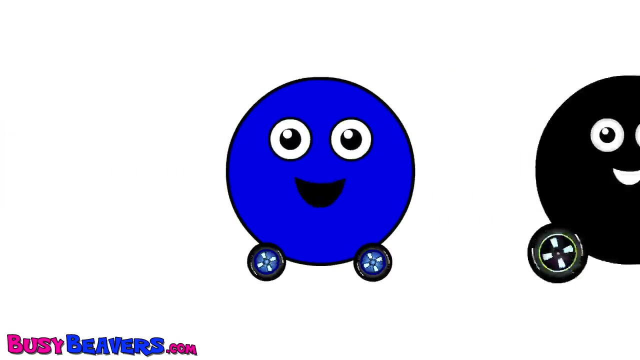 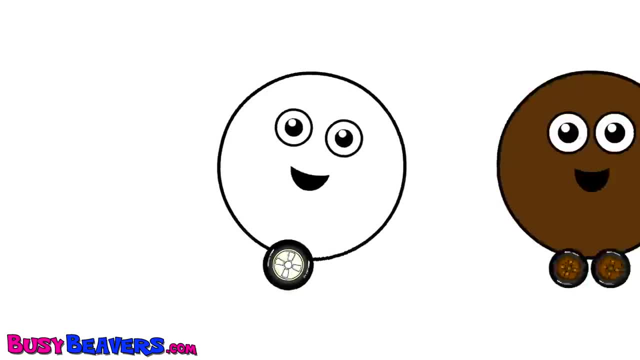 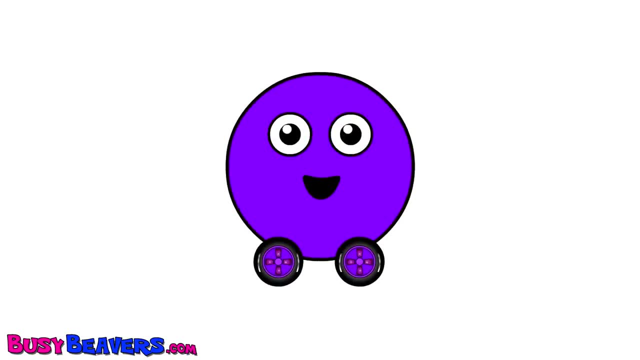 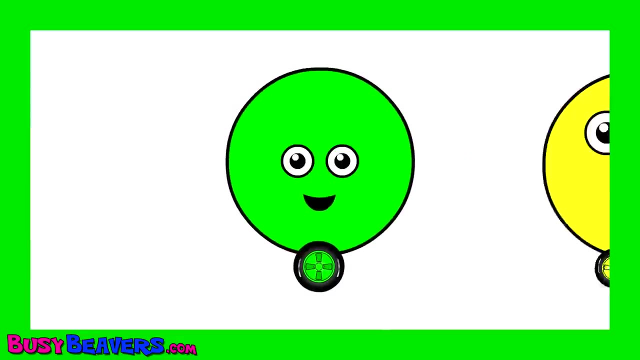 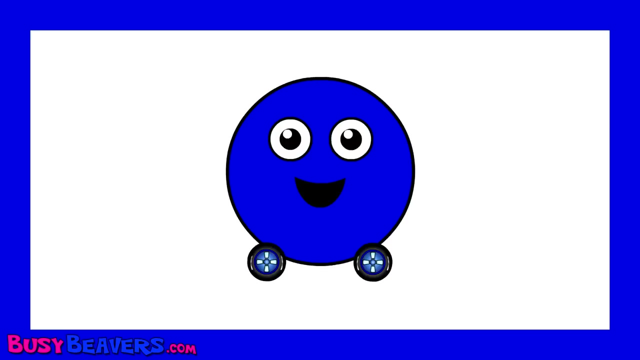 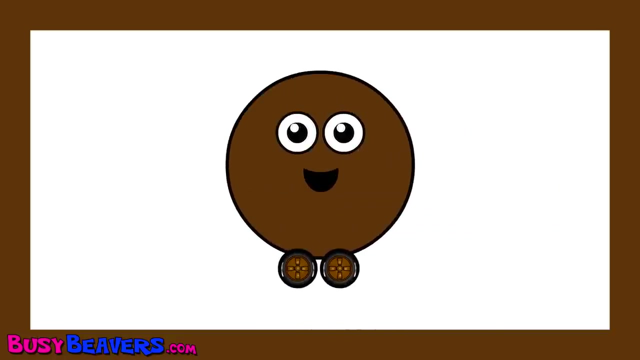 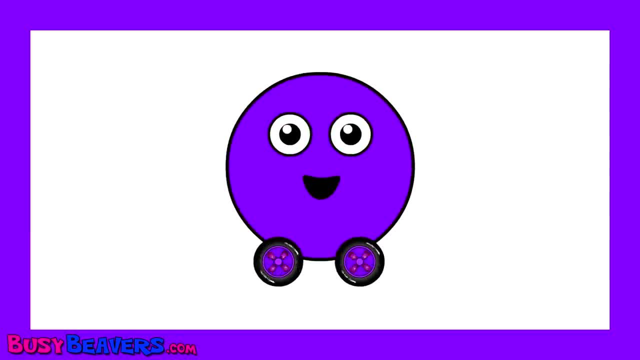 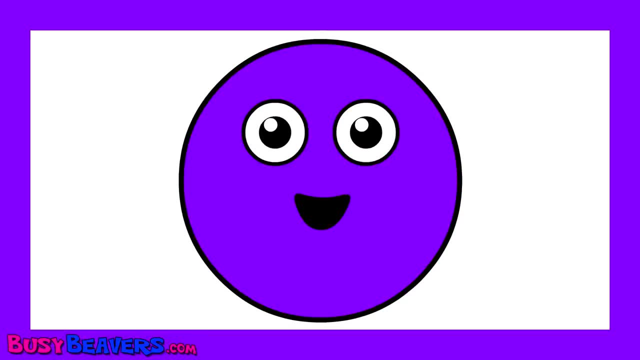 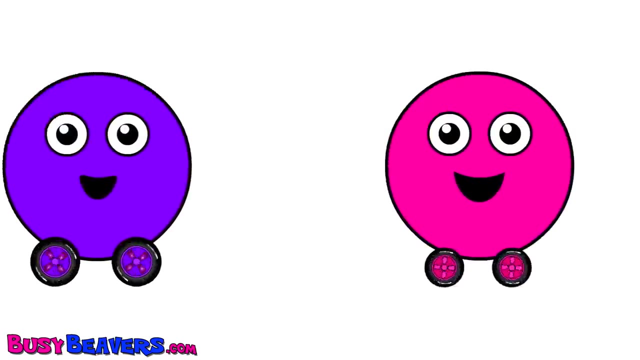 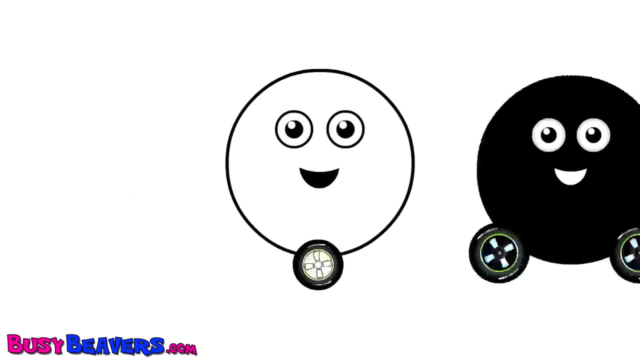 Pink, purple, purple, red, green, yellow, orange, blue, black, white, brown, pink, purple. Now let's try it backwards: Purple, purple, pink, pink, brown, brown, white, white, black, black, blue, blue. 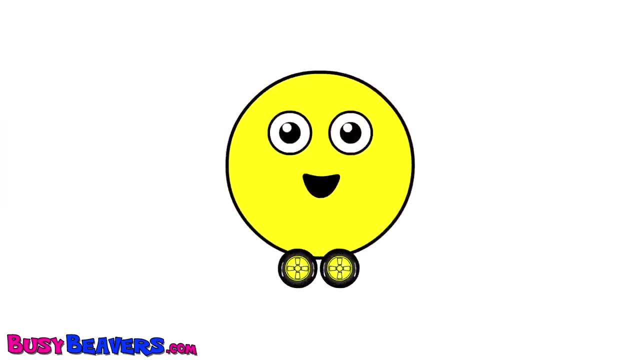 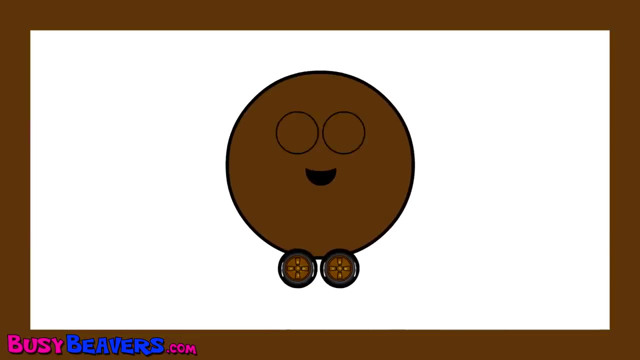 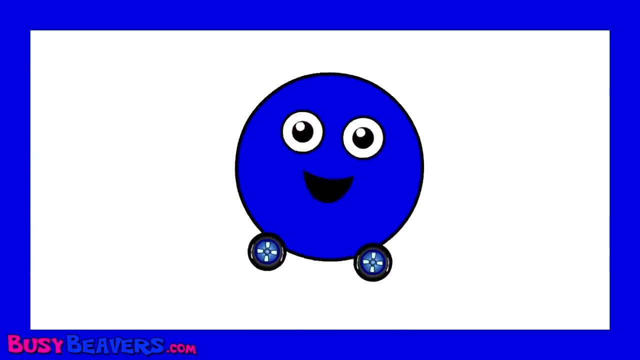 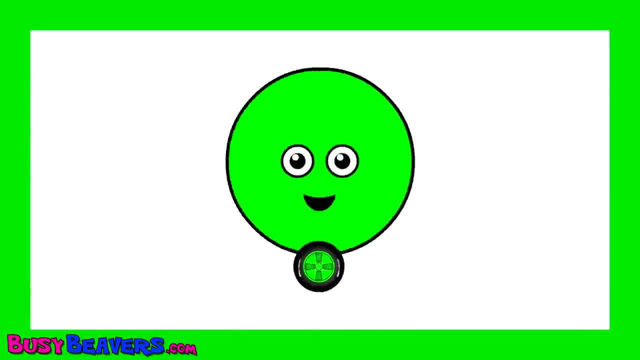 Orange, orange, yellow, yellow, green, green, red, red. One more time: Purple, purple, pink, pink, brown, brown, white, white, black, black, blue, blue, orange, orange, yellow, Yellow, yellow, green, green, red, red. 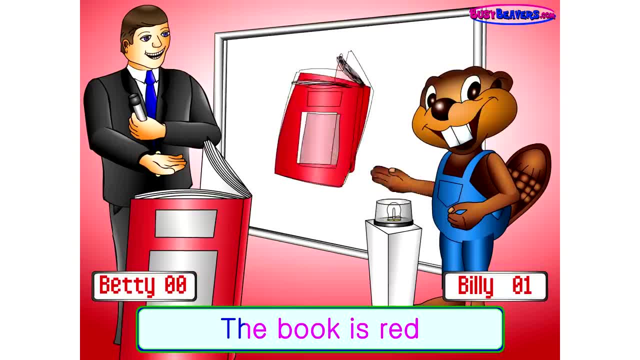 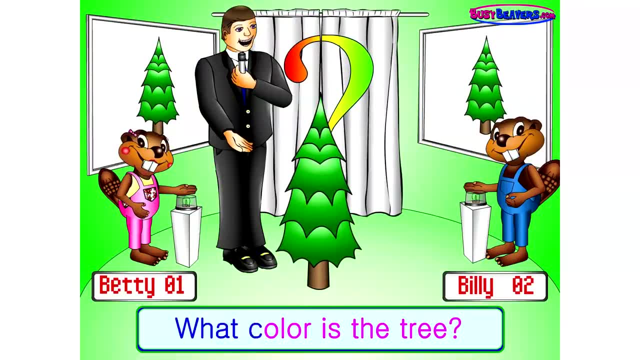 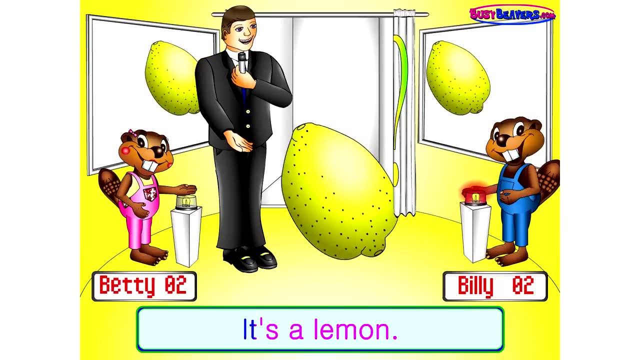 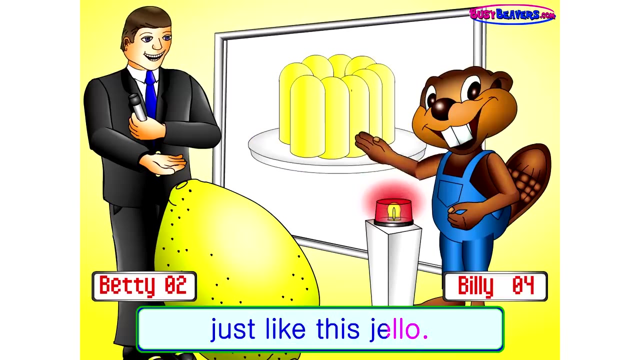 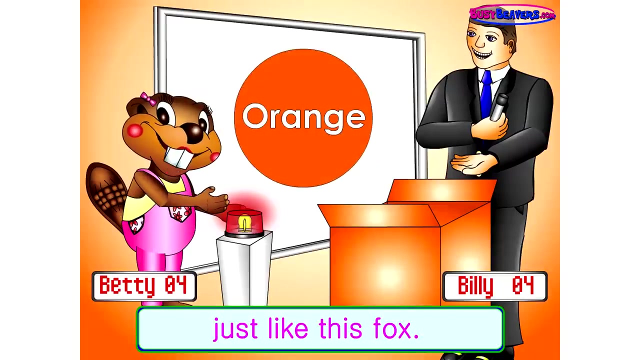 What's this? It's a bug. What color is the book? A bug is red, just like this bed. What's this? It's a tree. What color is the tree? The tree is green. you see, I see What's this? It's a lemon. What color is the lemon? The lemon is yellow, just like this jello. What's this? It's a box. What color is the box? The box is orange, just like this fox. 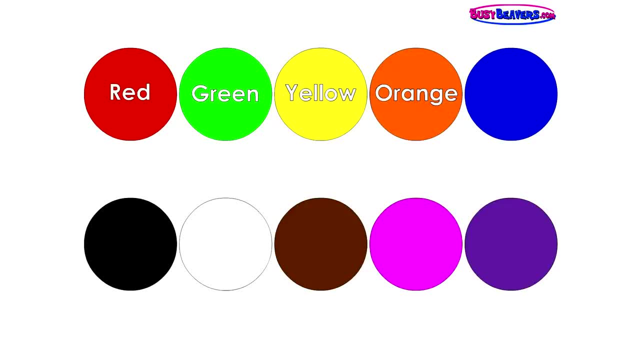 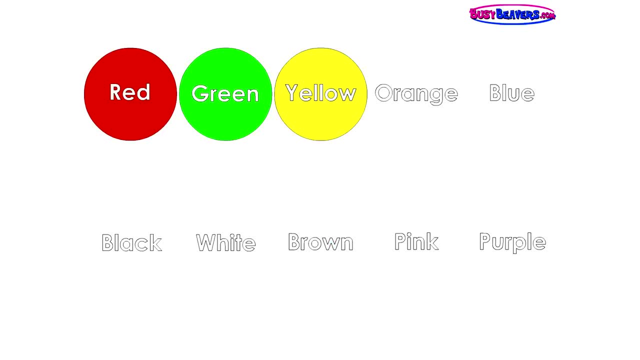 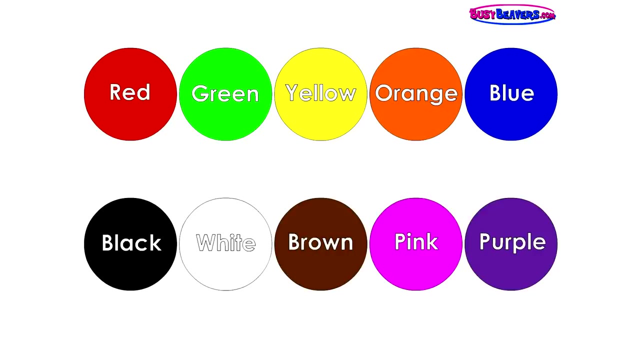 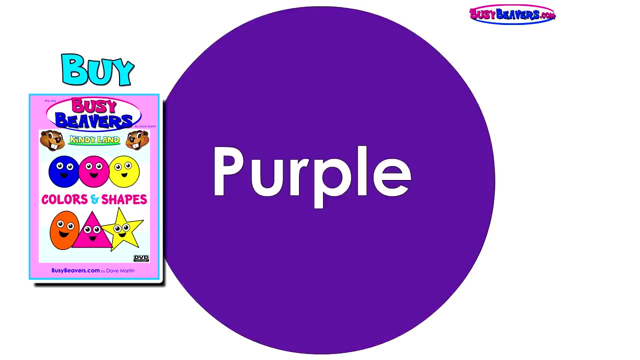 Red, green, yellow, orange, blue, Black, white, brown, pink, purple too. Red, green, yellow, orange, blue, Black, white, brown, pink, purple too. What's this? It's a pen. What color is the pen? 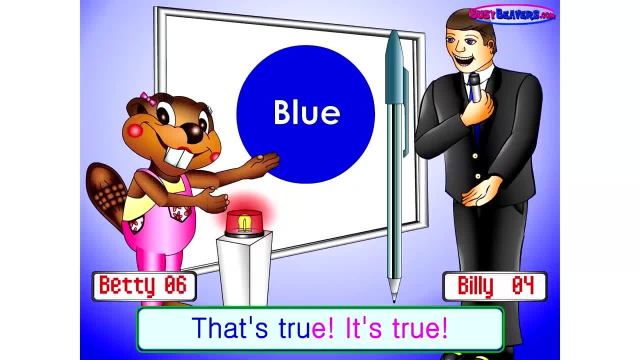 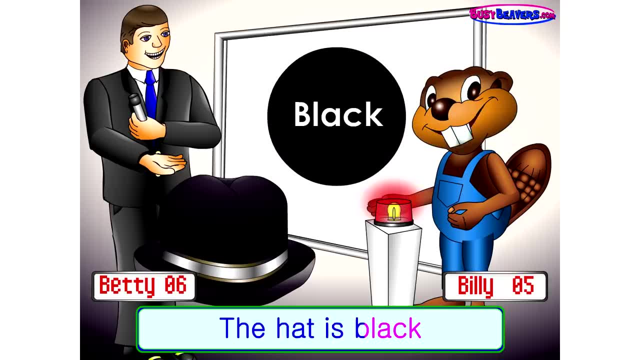 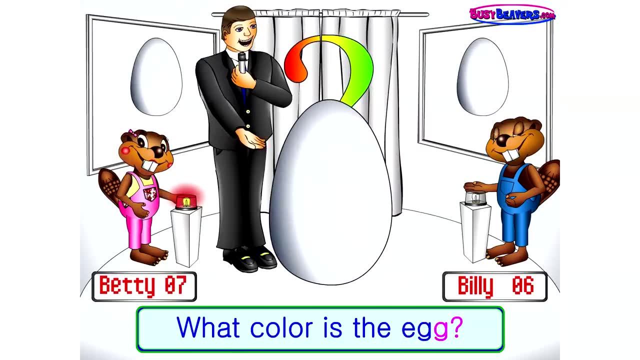 The pen is blue. That's true. It's true. What's this? It's a hat. What color is the hat? The hat is black, just like this cat. What's this? It's an egg. What color is the egg? The egg is white. 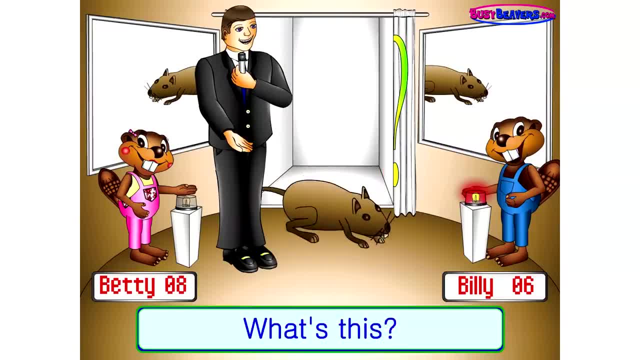 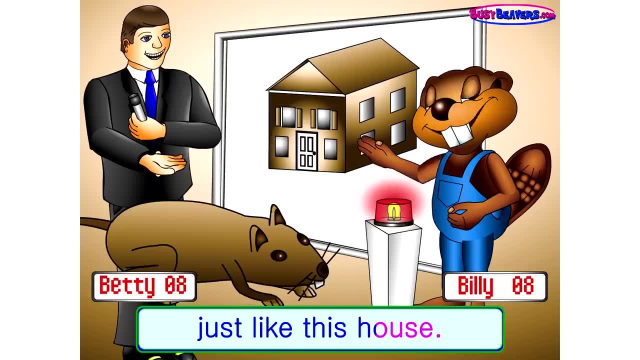 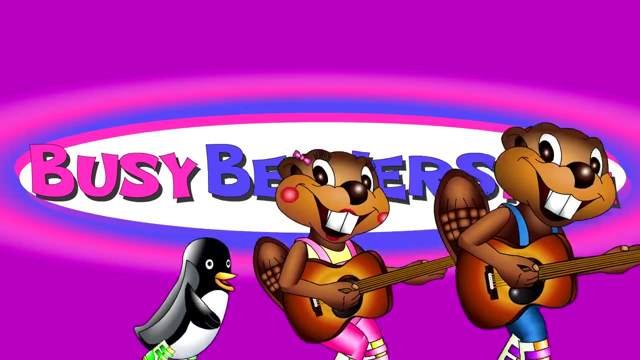 That's right, I'm right. What's this? It's a mouse. What color is the mouse? The mouse is brown, just like this. Red, green, yellow, orange, blue, Black, white, brown, pink, purple too. 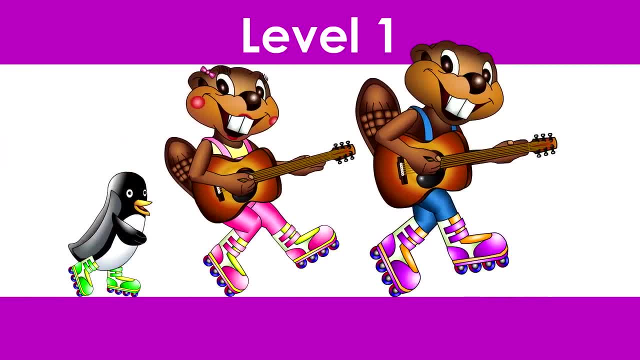 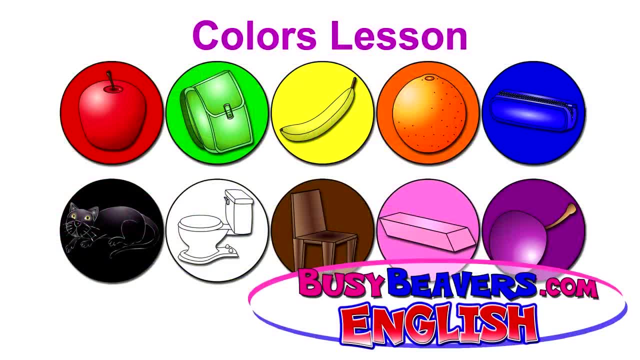 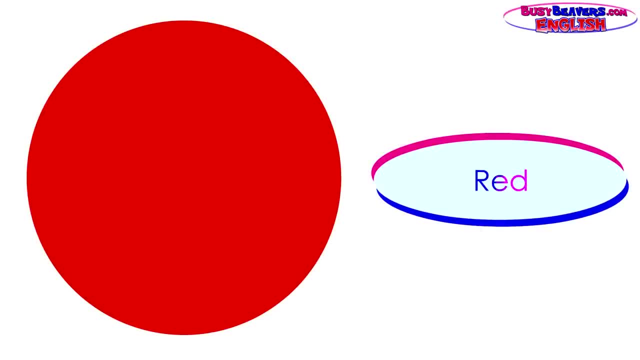 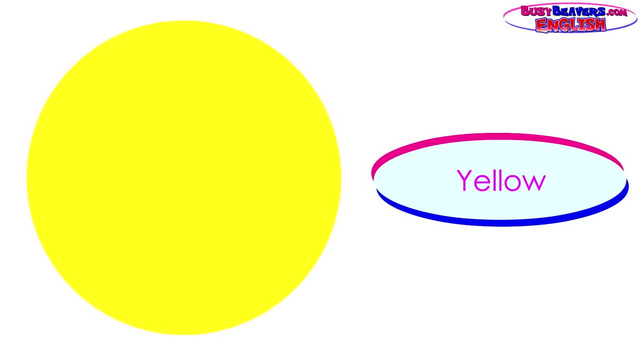 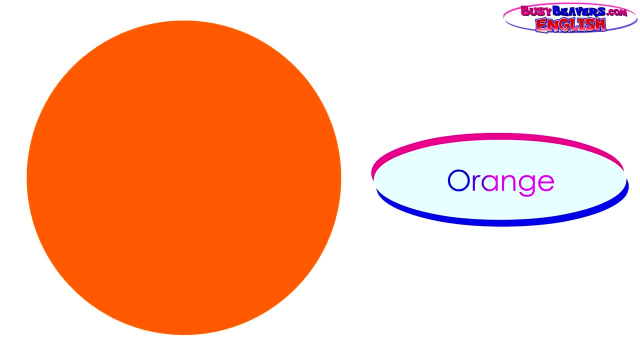 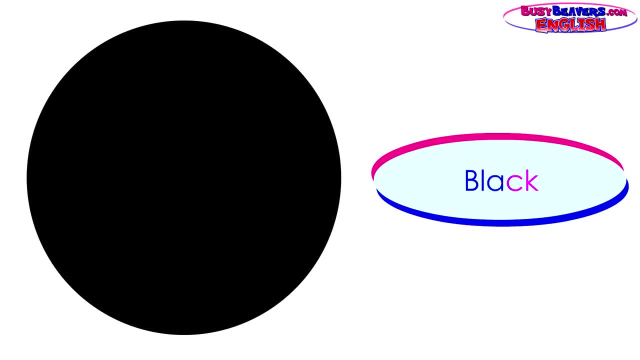 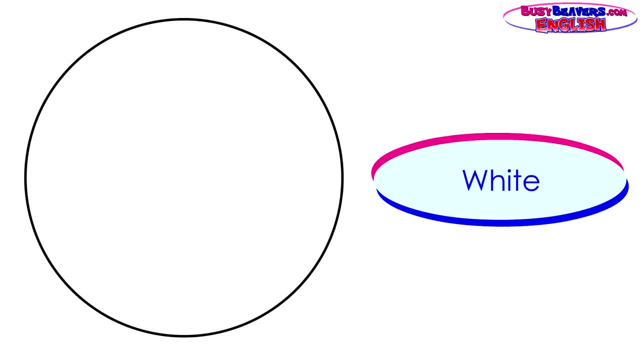 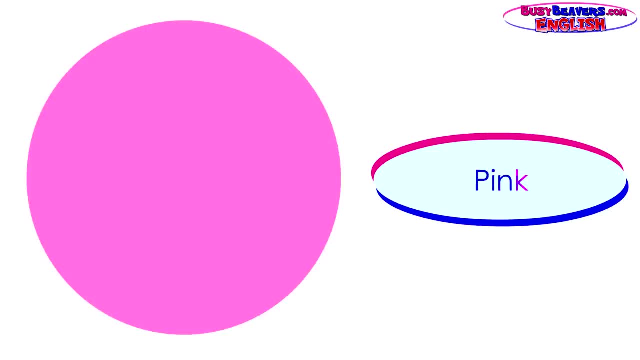 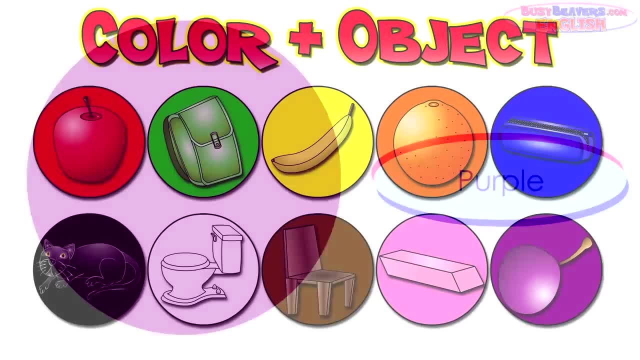 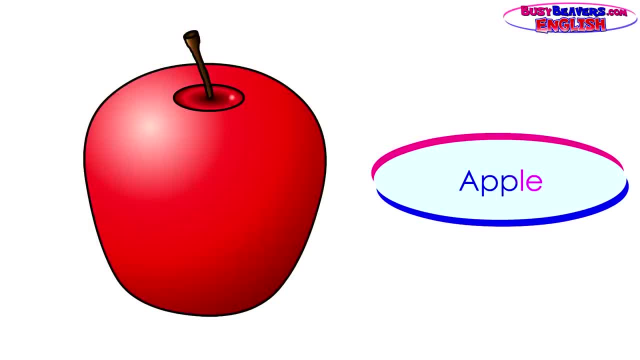 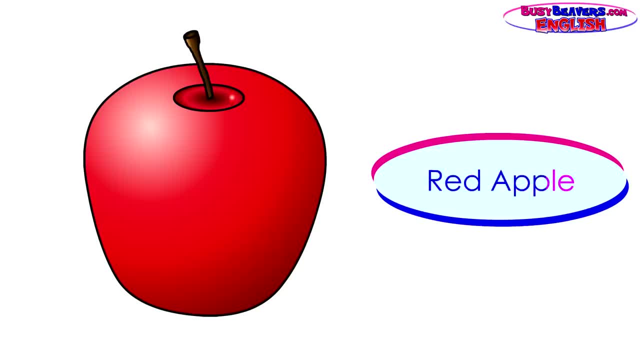 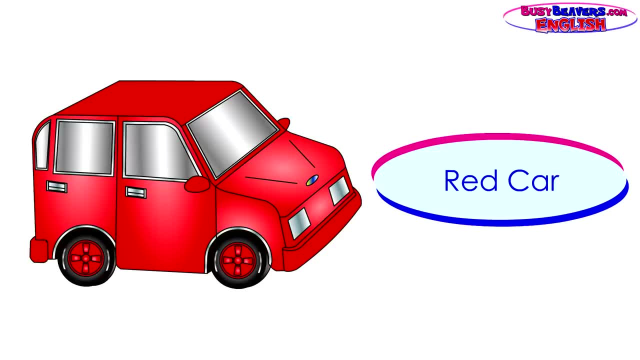 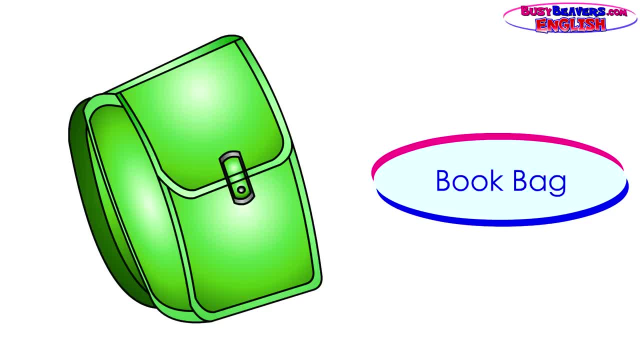 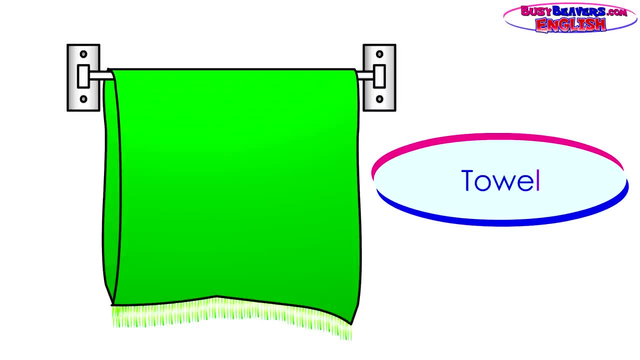 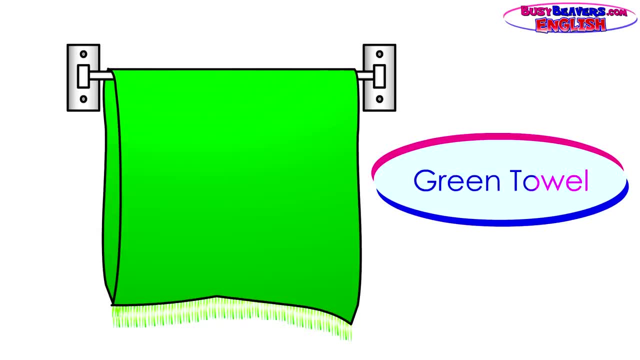 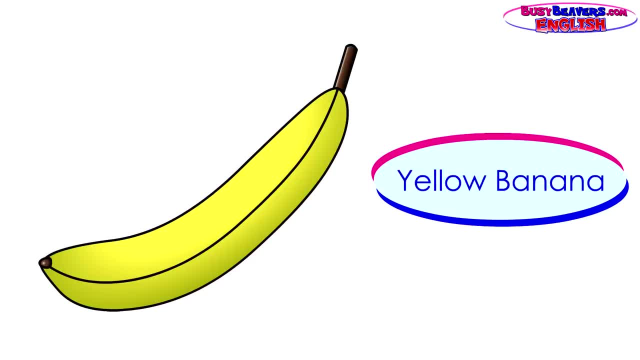 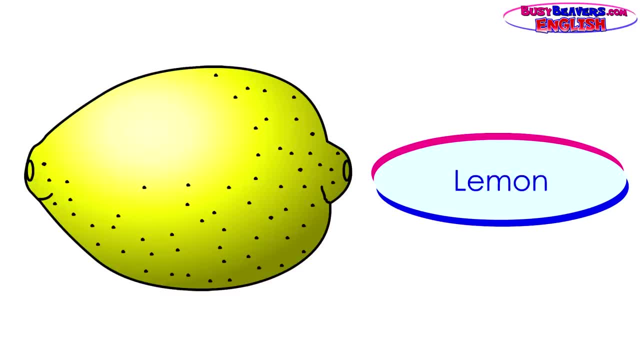 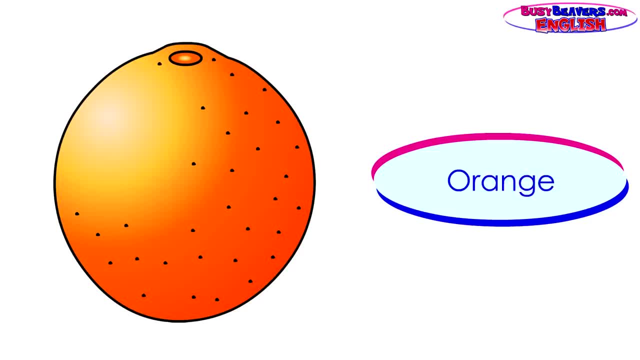 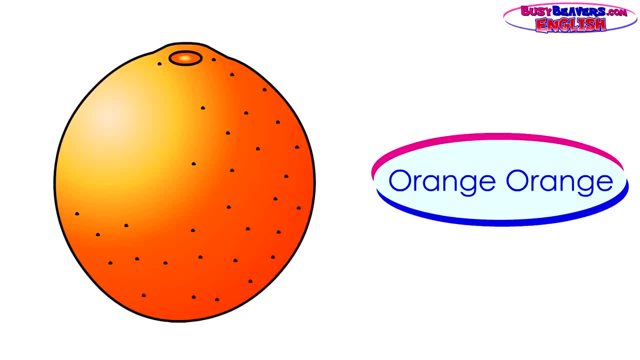 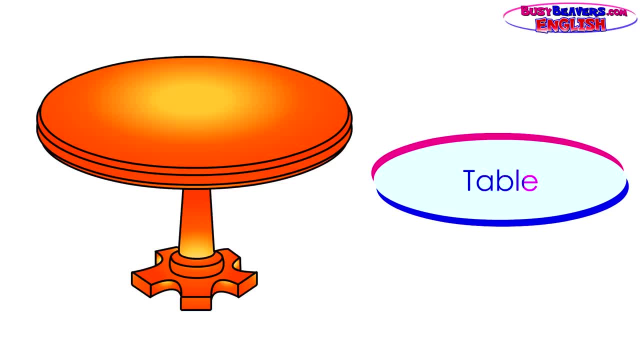 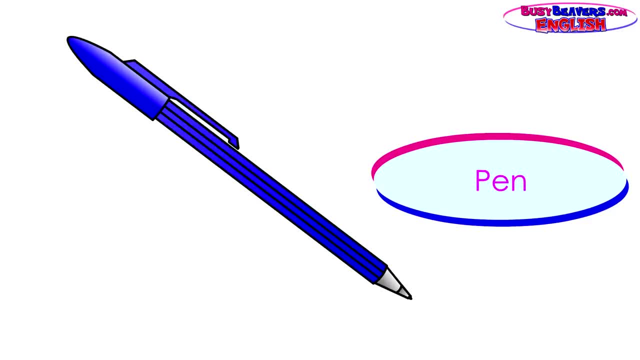 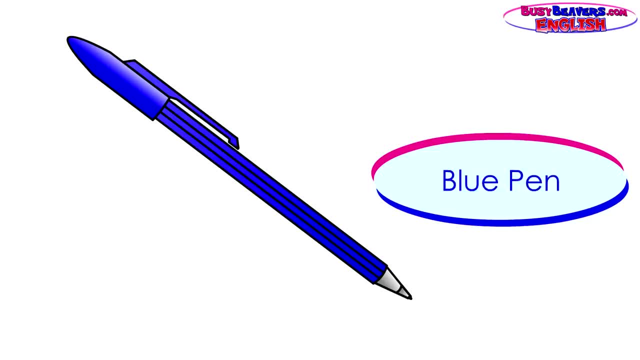 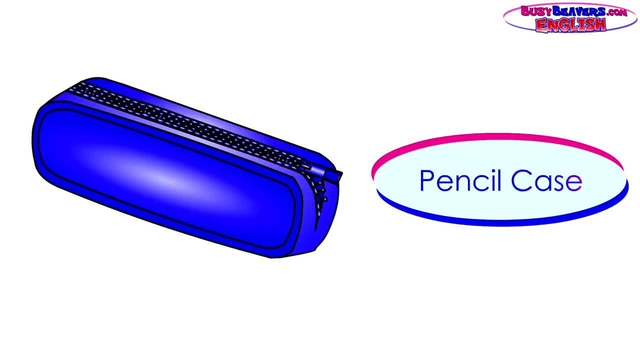 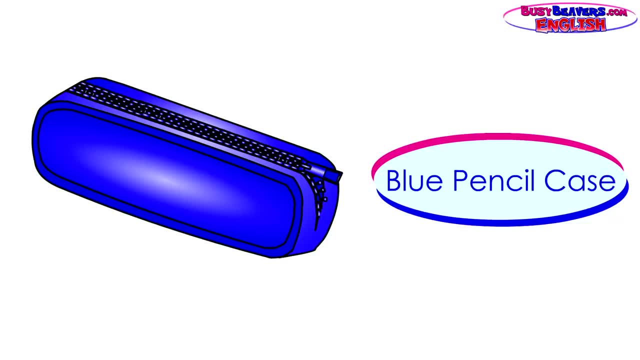 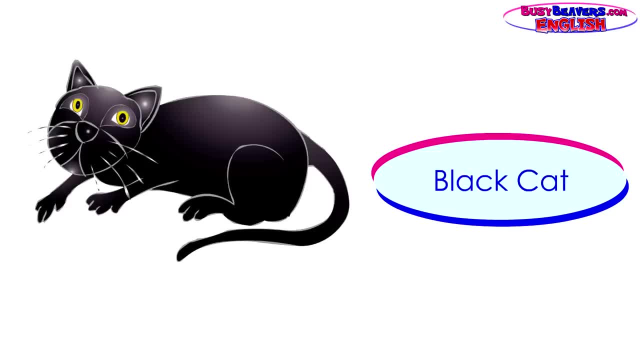 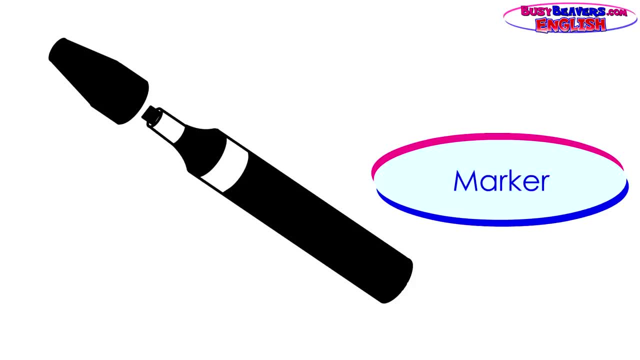 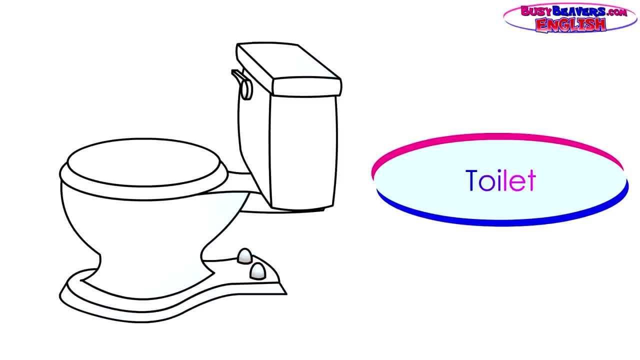 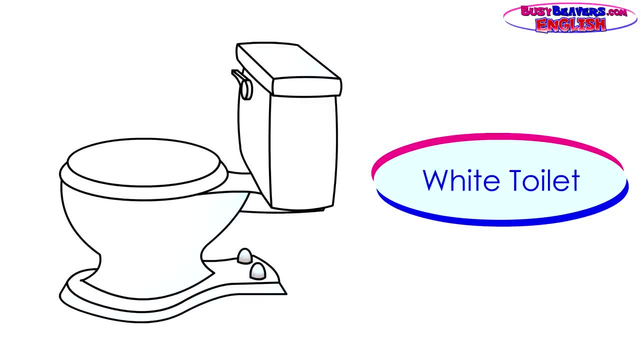 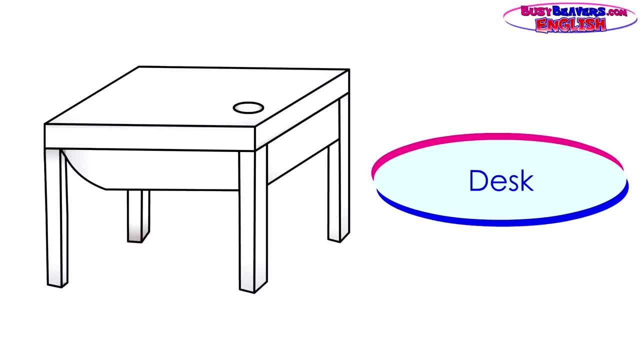 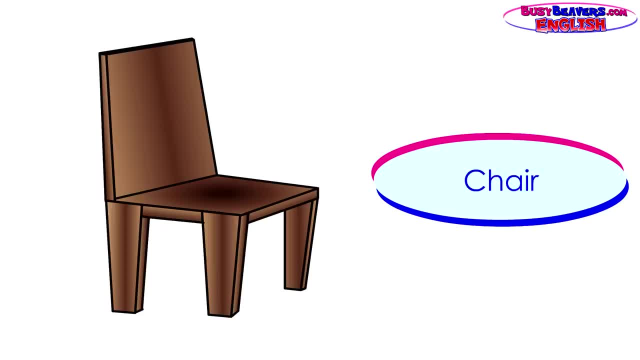 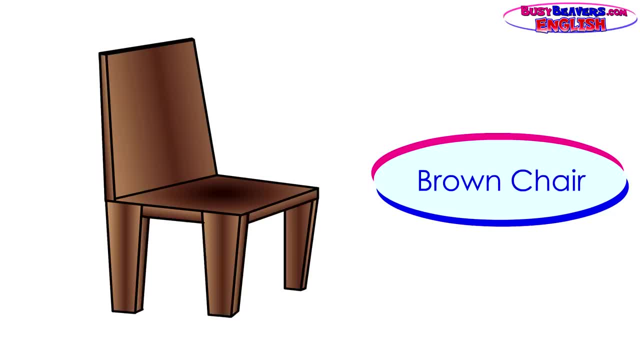 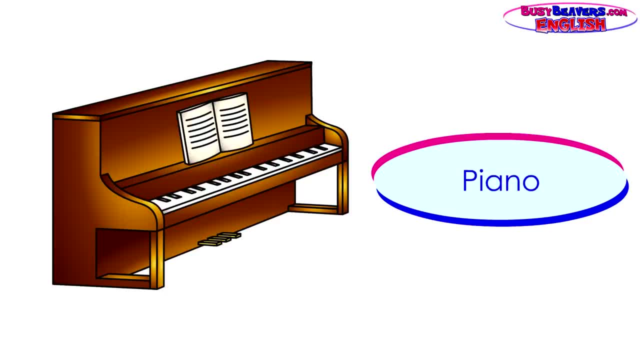 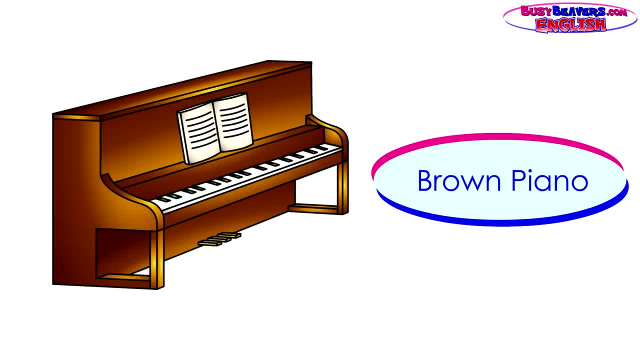 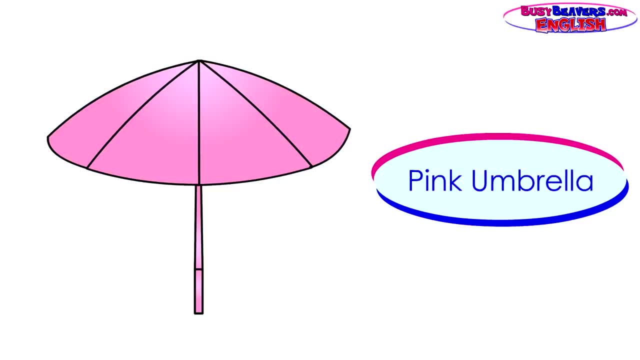 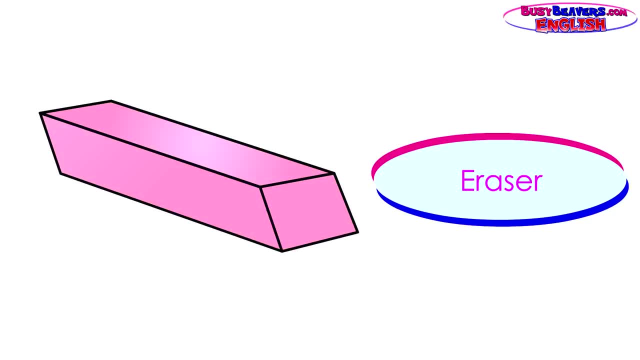 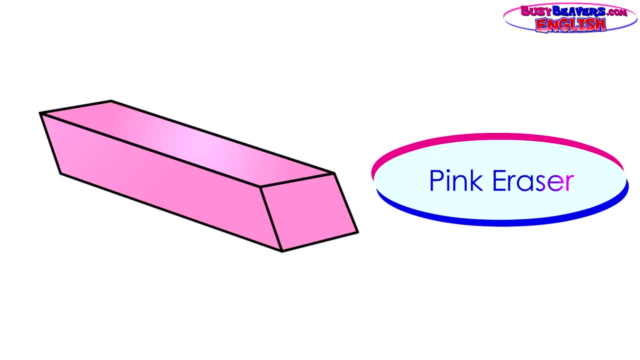 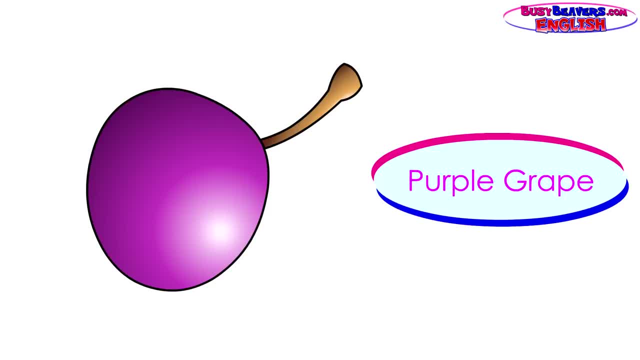 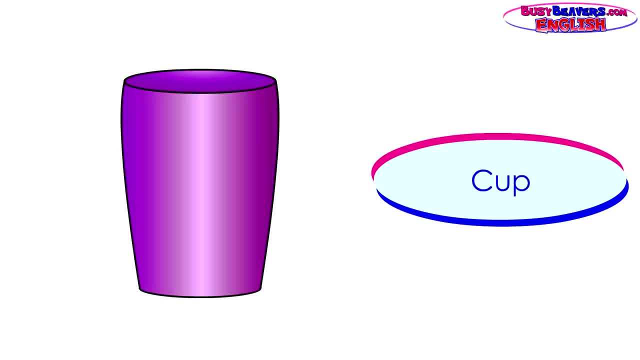 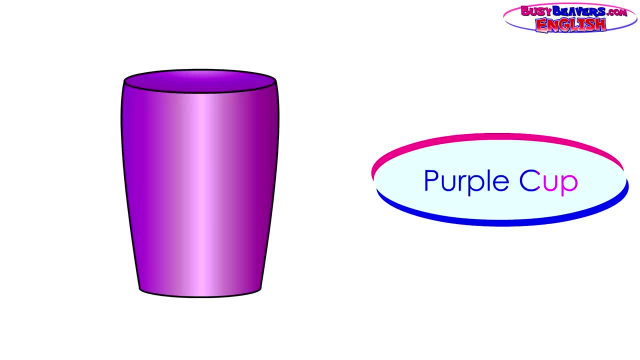 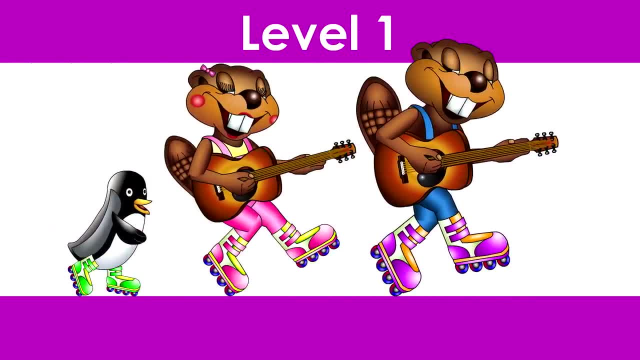 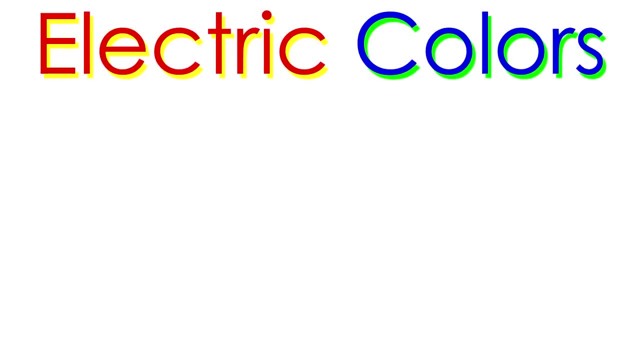 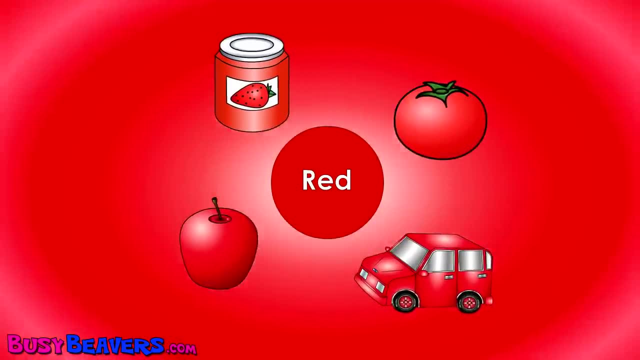 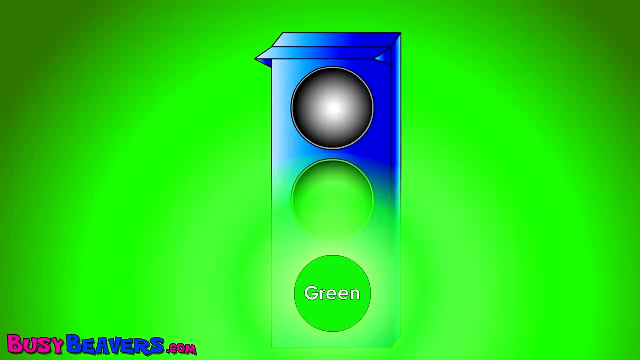 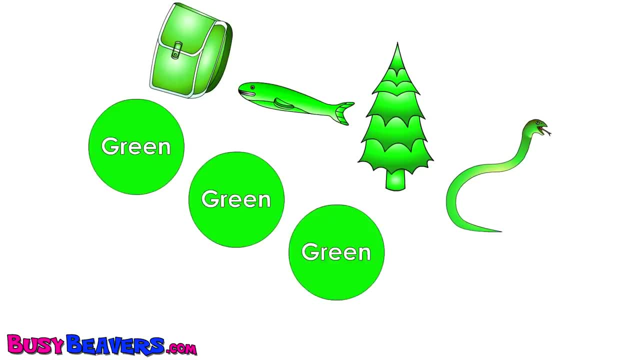 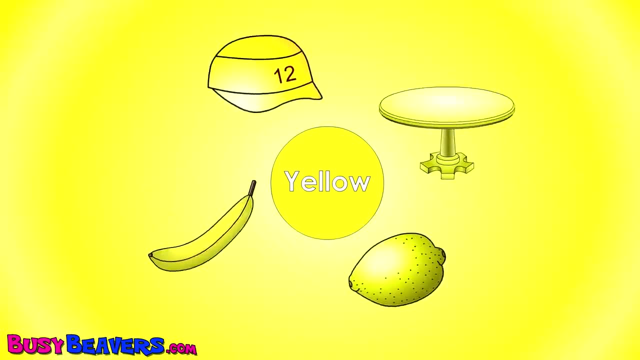 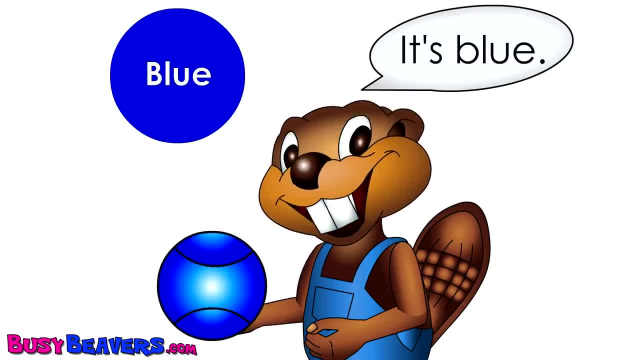 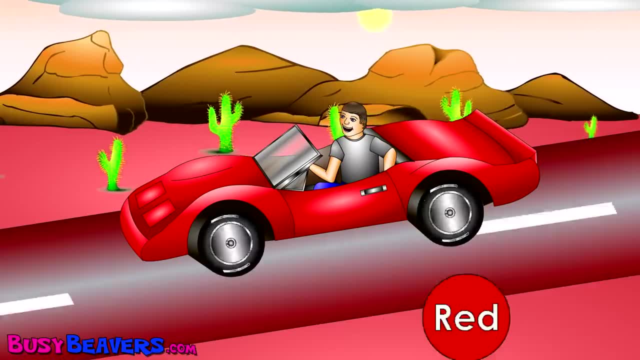 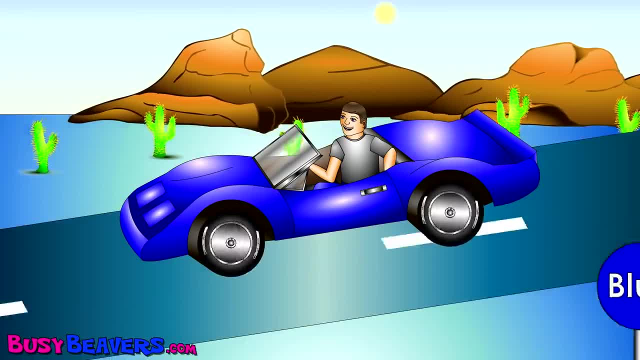 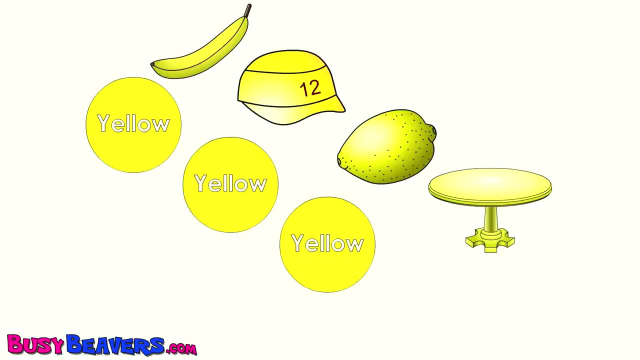 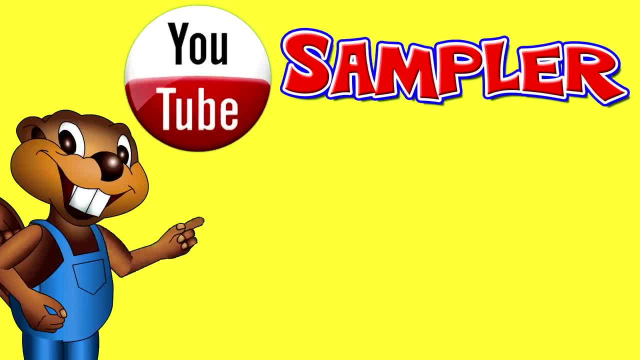 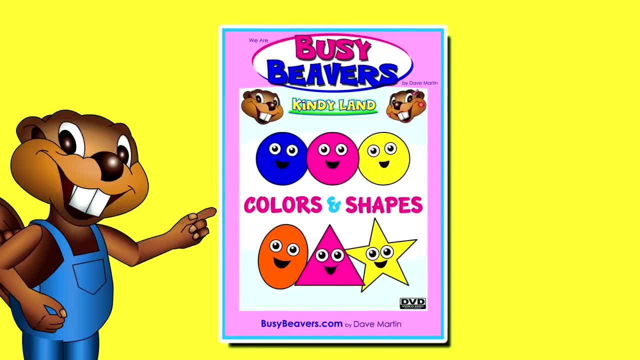 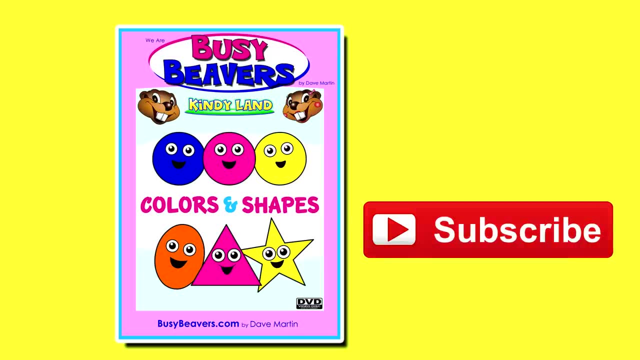 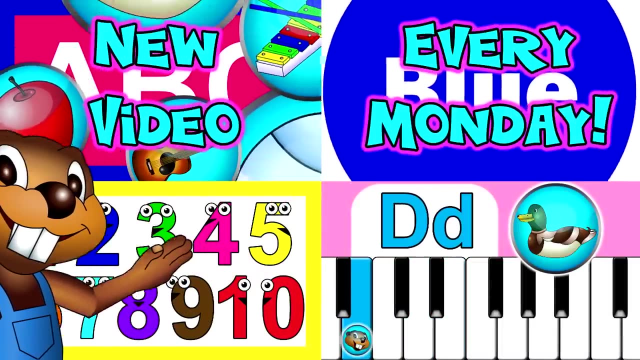 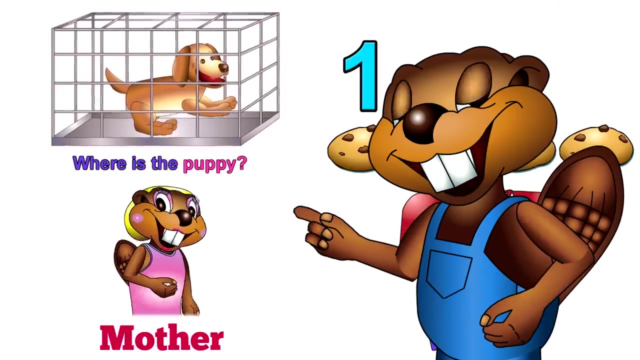 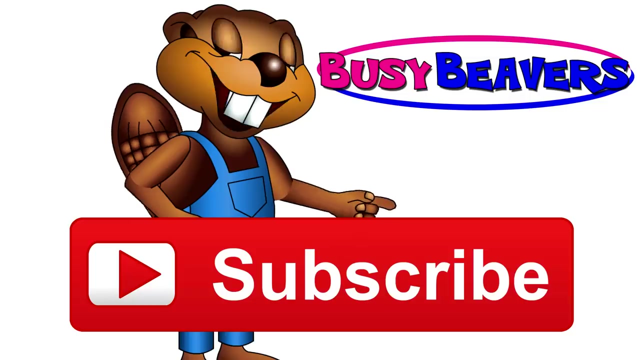 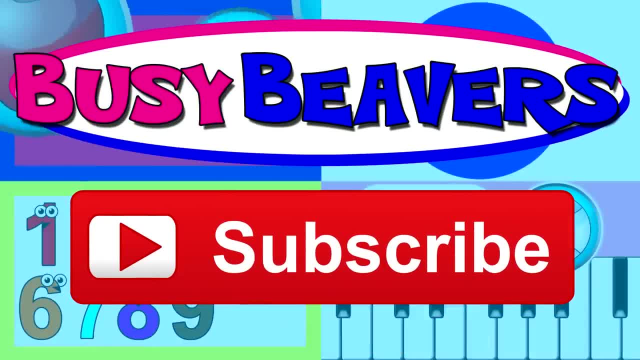 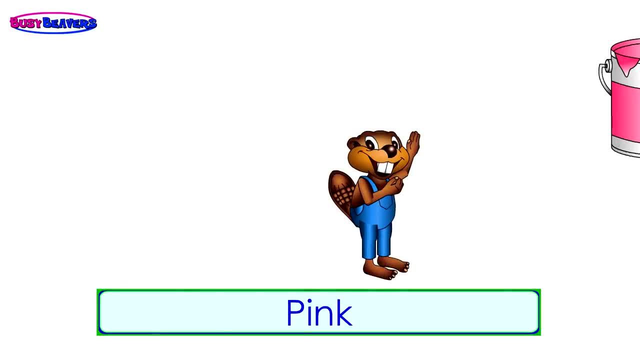 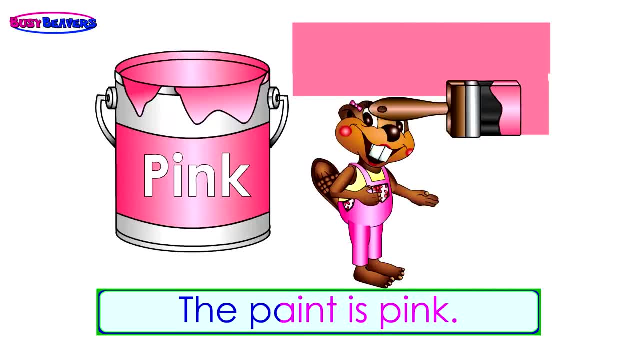 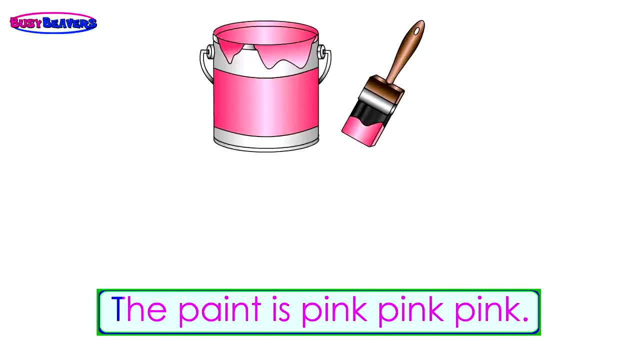 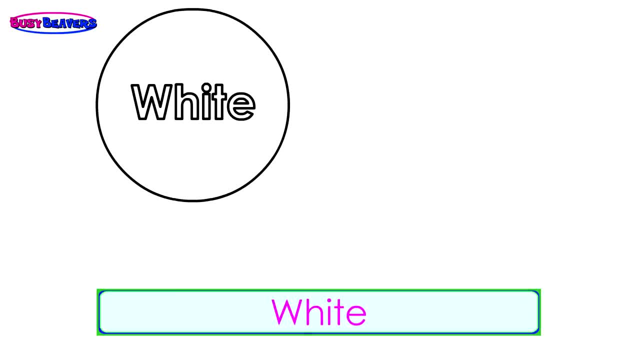 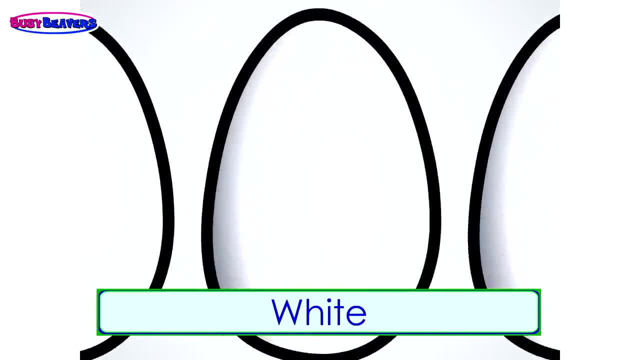 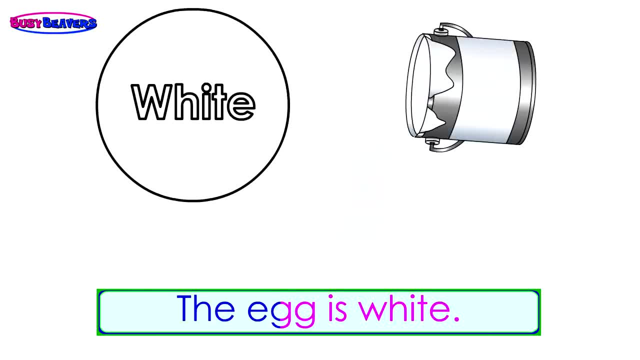 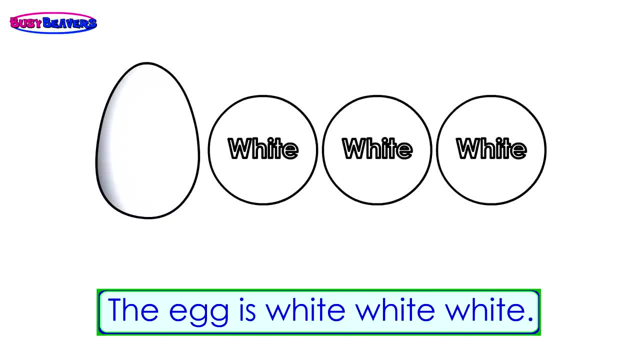 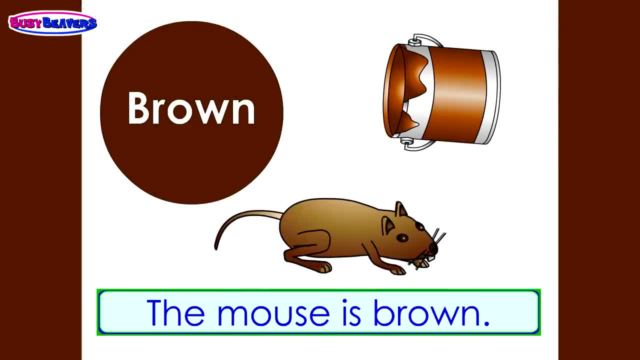 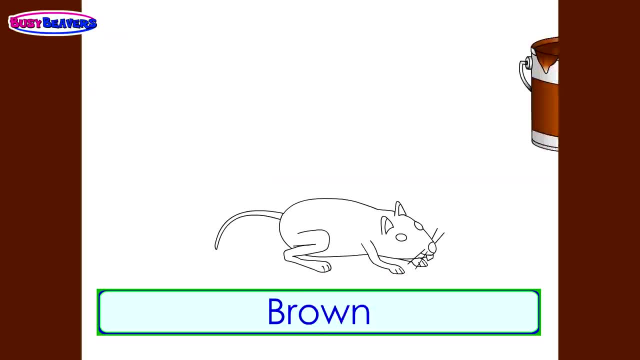 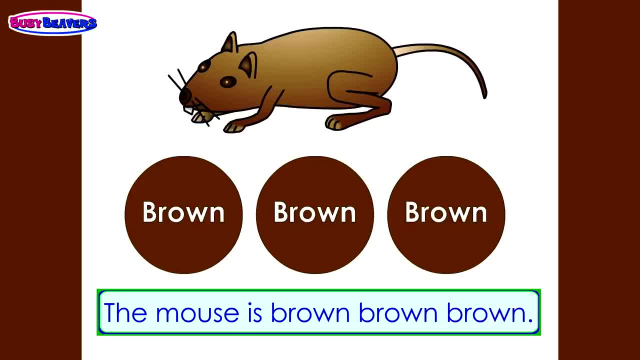 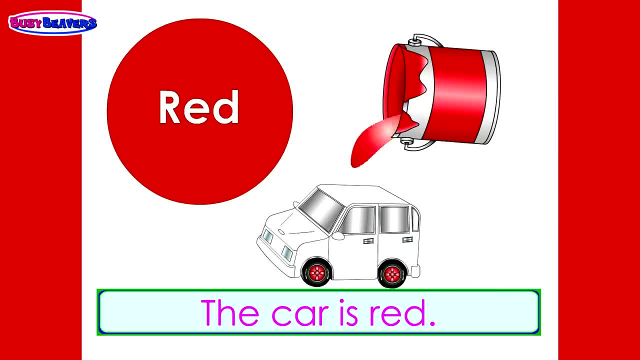 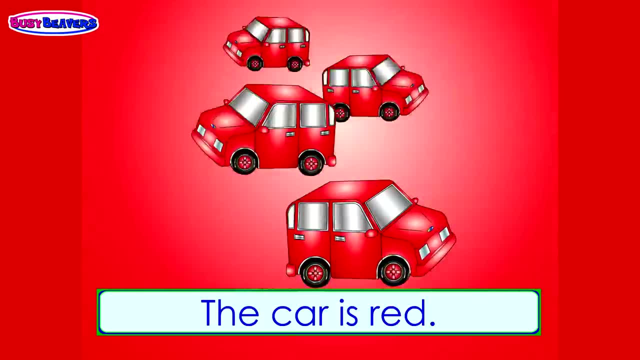 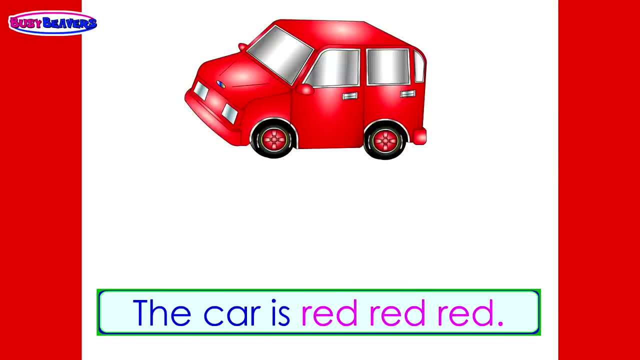 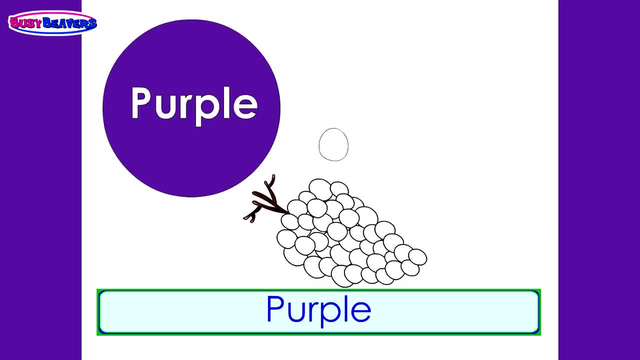 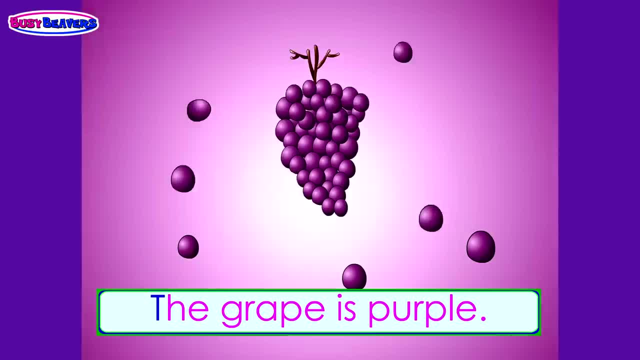 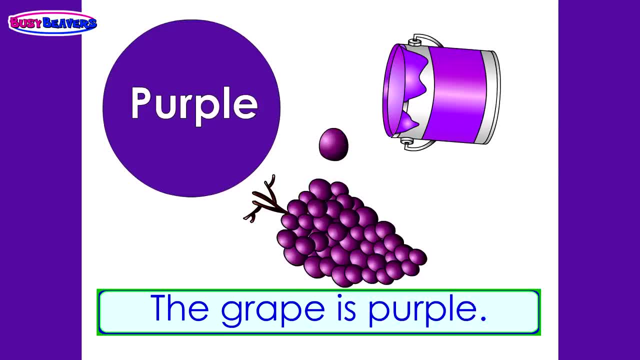 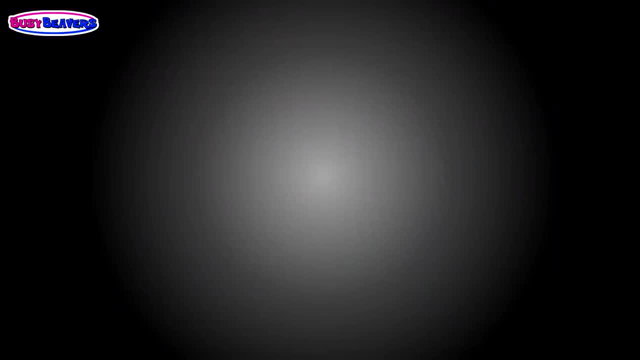 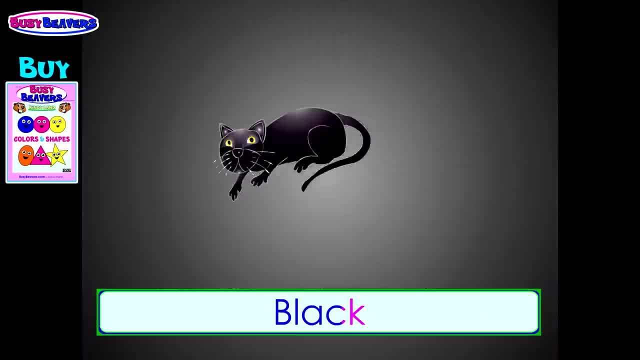 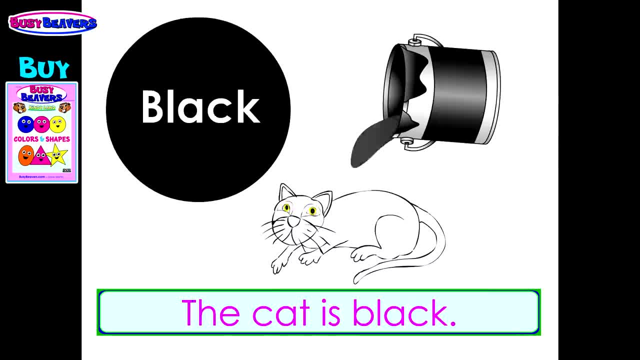 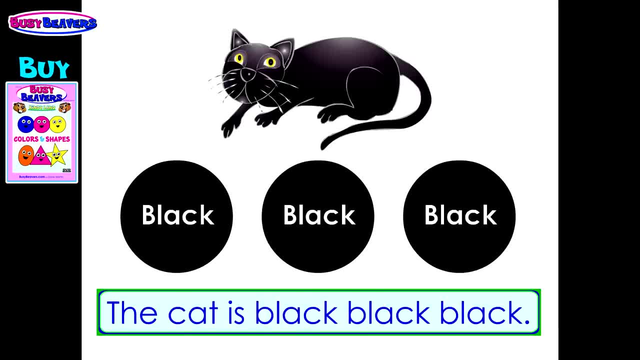 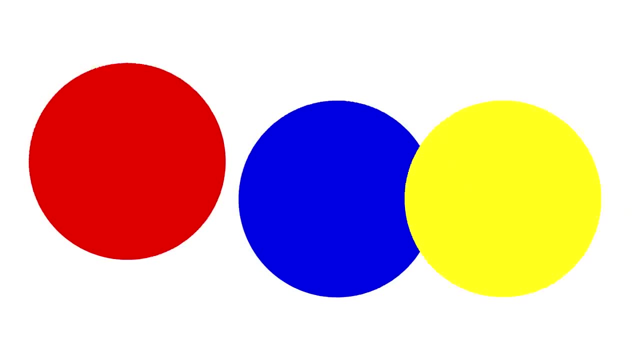 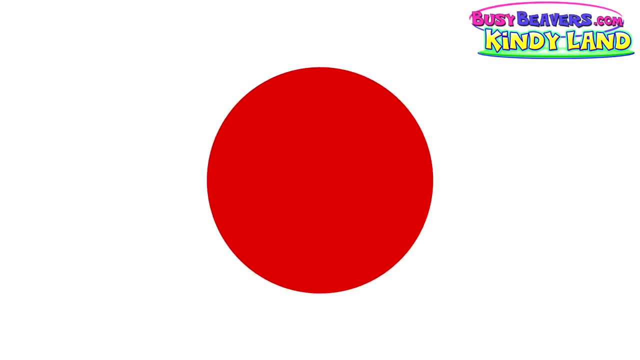 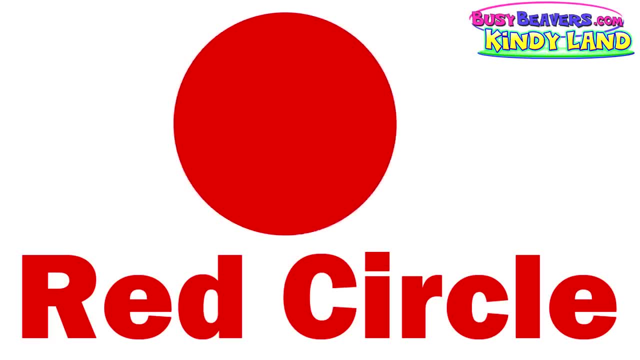 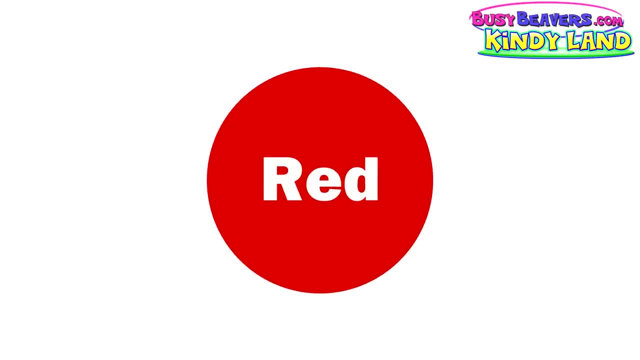 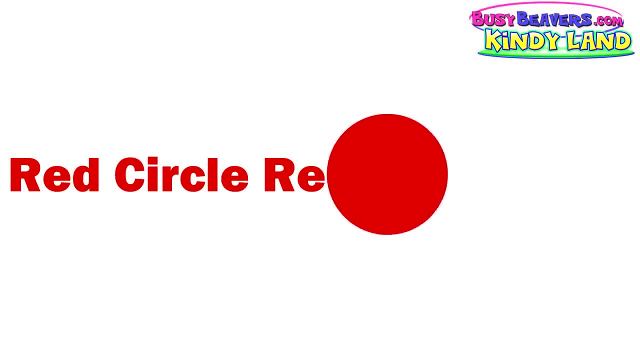 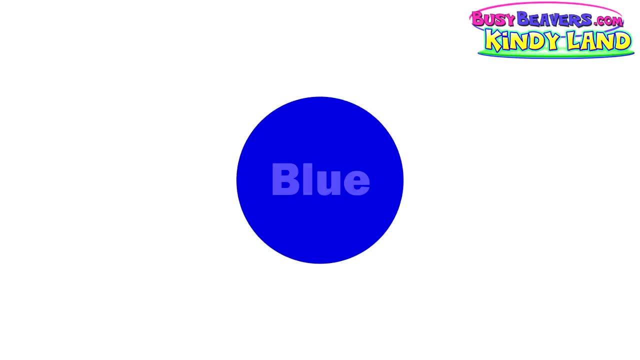 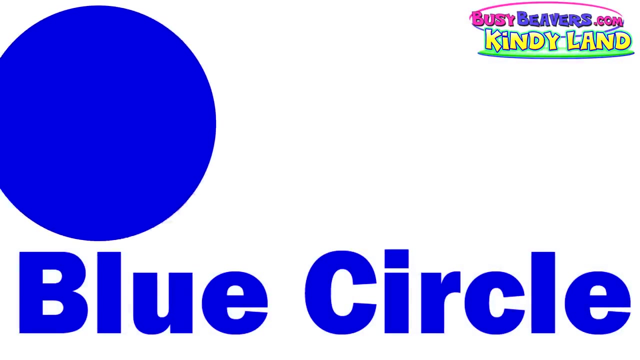 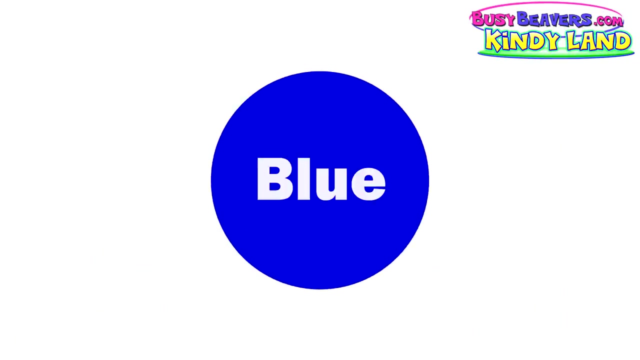 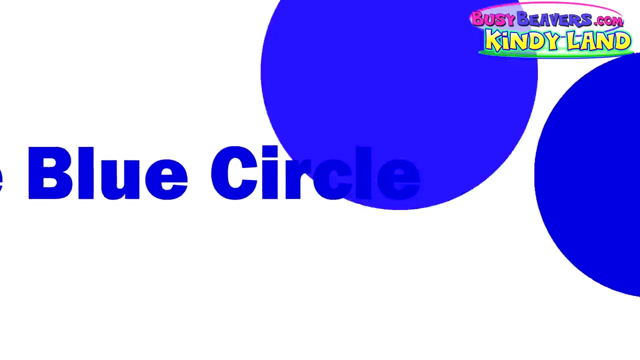 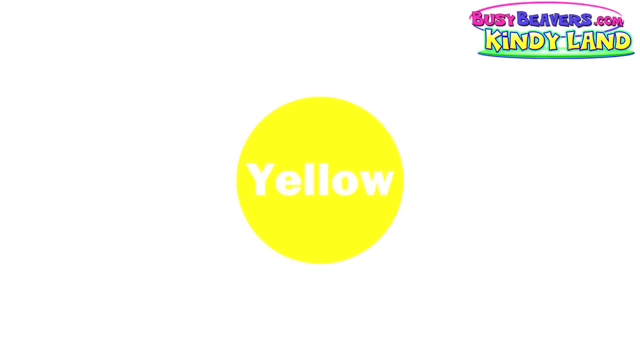 What's this? It's a box. What's this? It's a box. Red circle, red circle, Blue, blue, blue, blue, Blue circle, blue circle, Blue, blue, blue, blue, Blue circle, blue circle, Yellow, yellow, yellow, yellow. 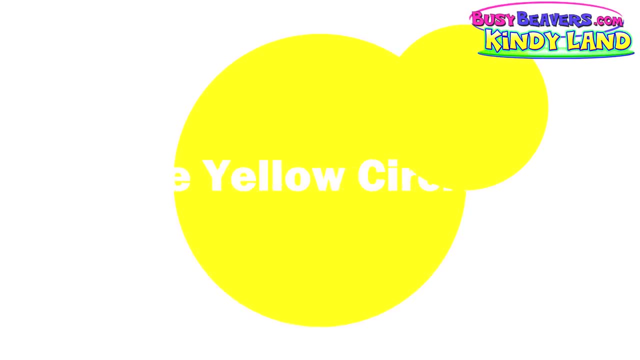 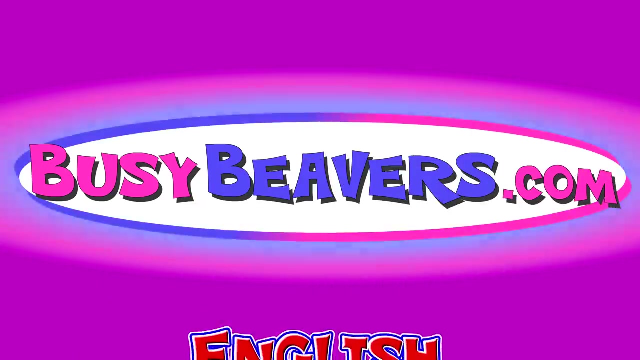 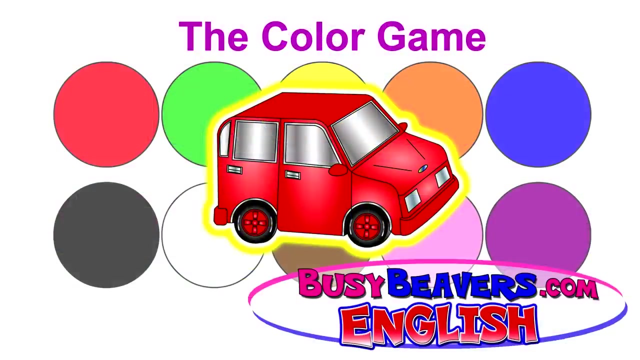 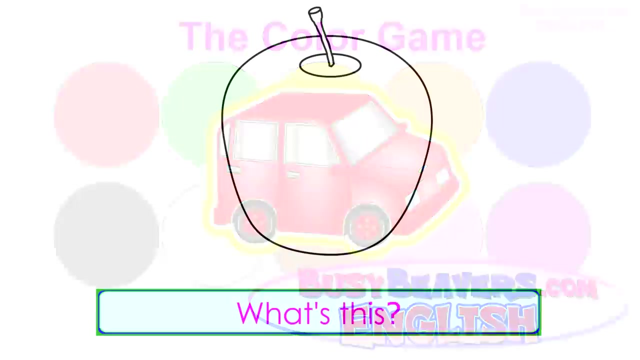 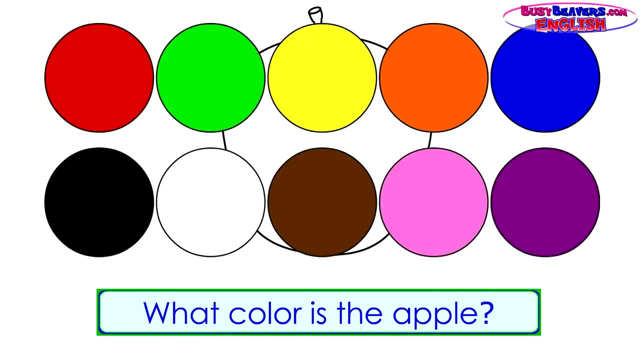 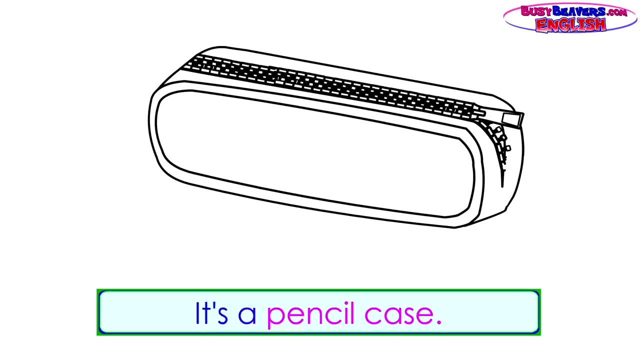 Yellow circle, yellow circle, Yellow, yellow, yellow, yellow, Yellow circle, yellow circle. The Color Game. What's this? It's an apple. What color is the apple? The apple is red. What's this? It's a pencil case. What color is the pencil case? 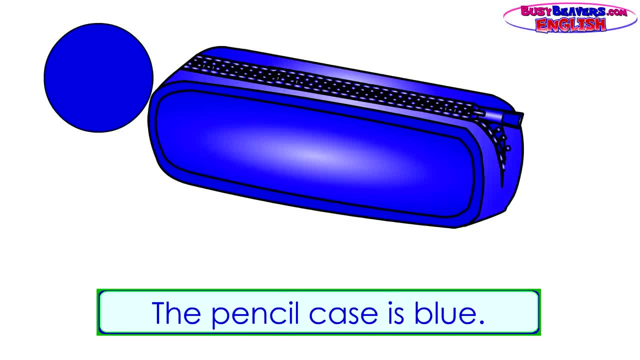 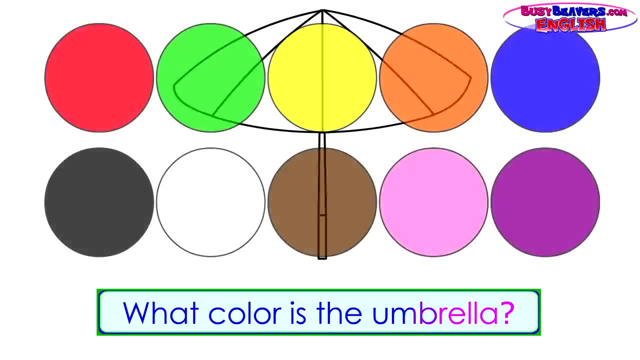 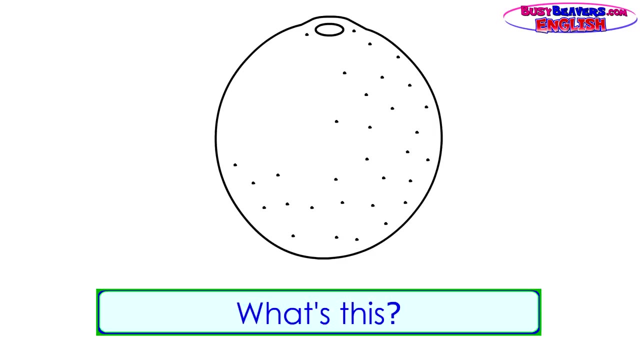 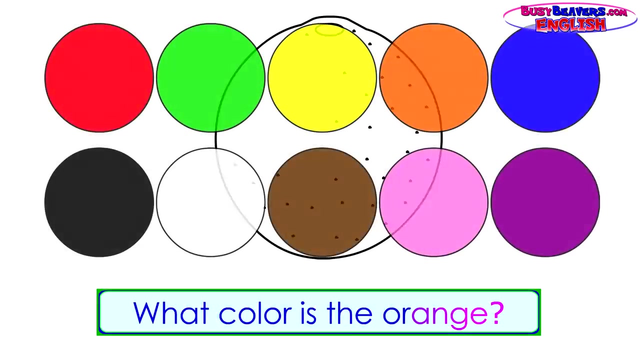 The pencil case is blue. What's this? It's an umbrella. What color is the umbrella? The umbrella is pink. What color is the umbrella? What's this? It's an orange. What color is the orange? The orange is orange. 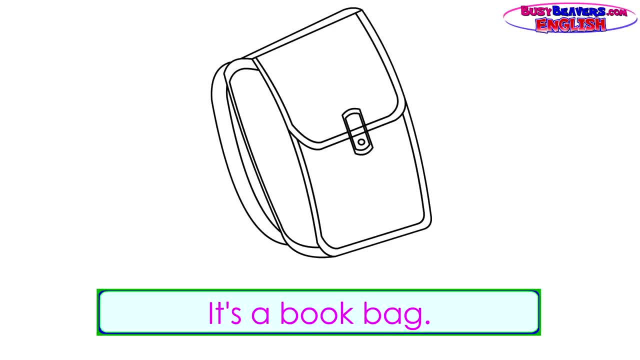 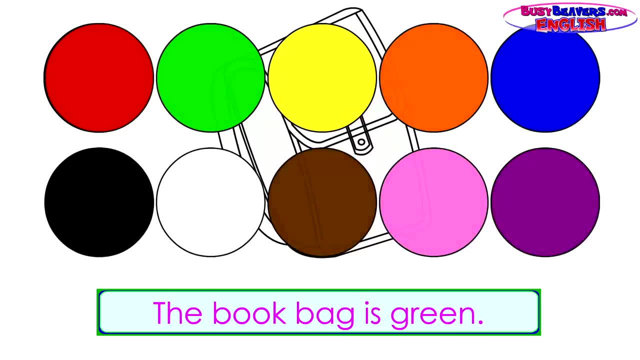 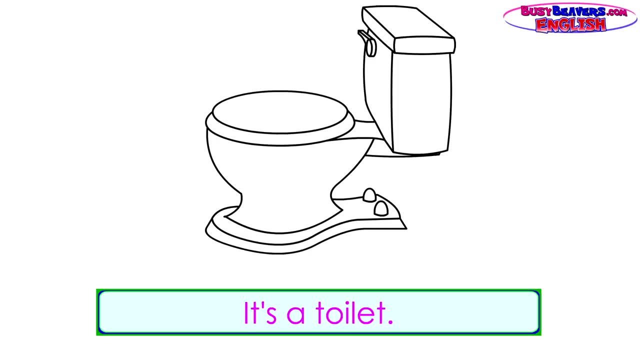 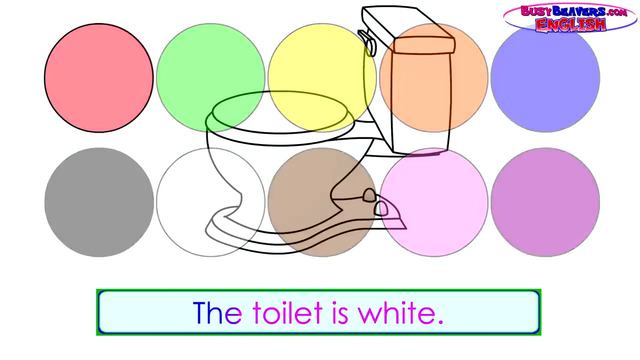 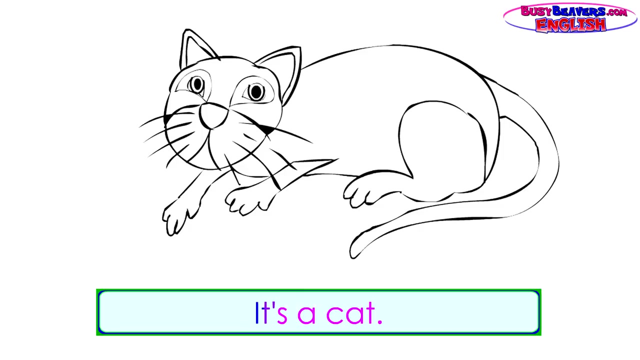 What's this? It's a book bag. What color is the book bag? The book bag is green. What's this? It's a toilet. What color is the toilet? The toilet is white. What's this? It's a cat. 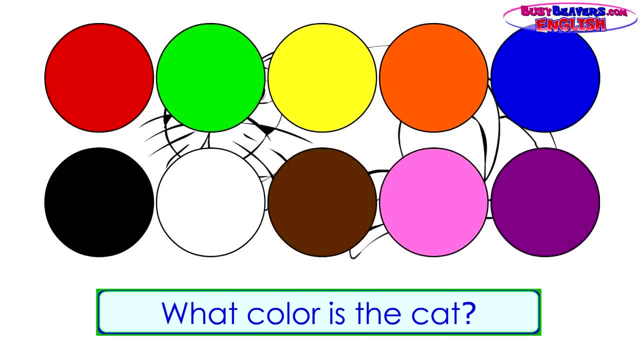 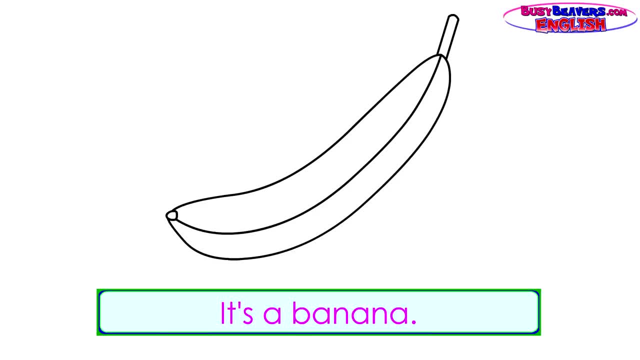 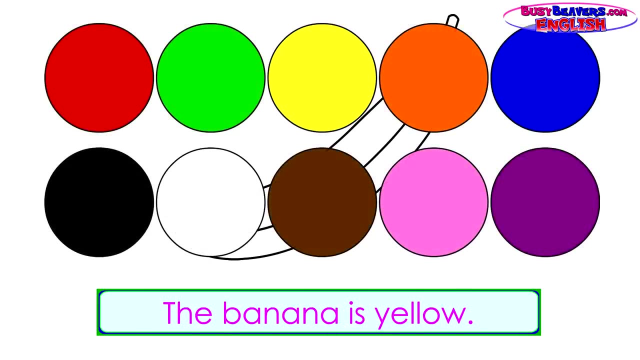 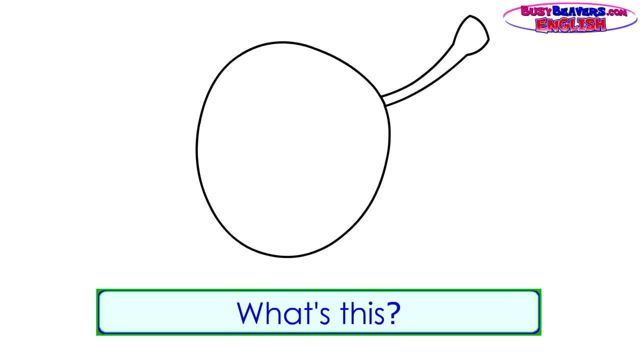 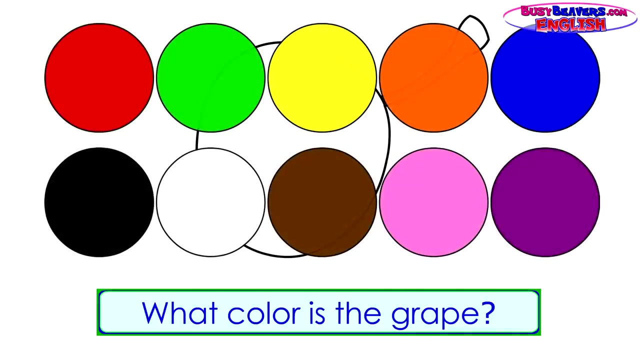 What color is the cat? The cat is black. What's this? It's a banana. What color is the banana? The banana is yellow. What's this? It's a grape. What color is the grape? The grape is purple. 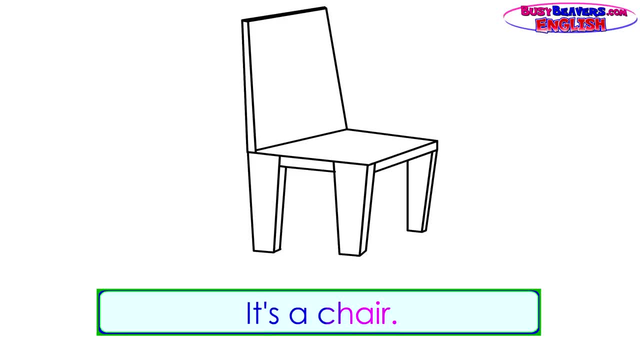 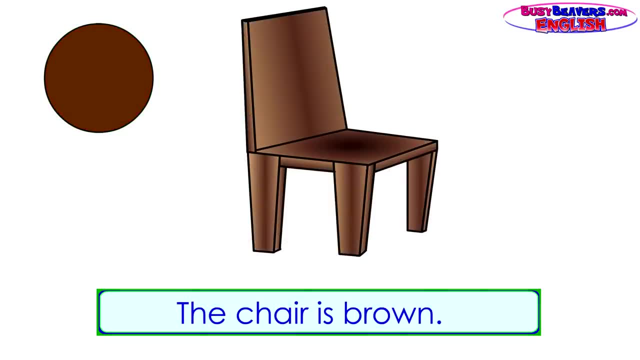 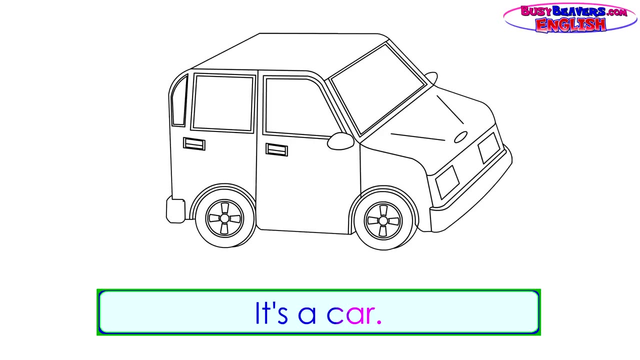 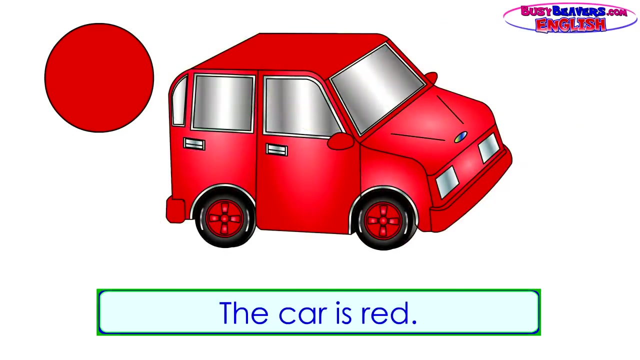 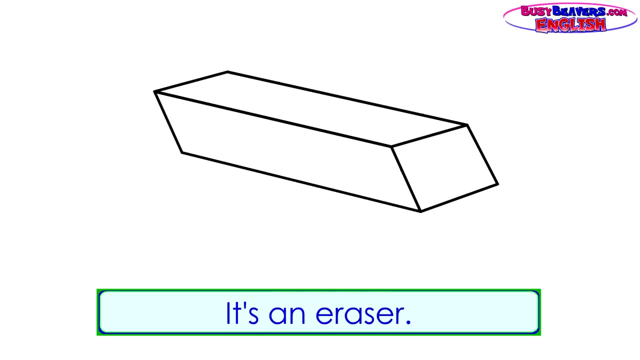 What's this? It's a chair. What color is the chair? The chair is brown. What's this? It's a car. What color is the car? The car is red. What's this? It's an eraser. What color is the eraser? 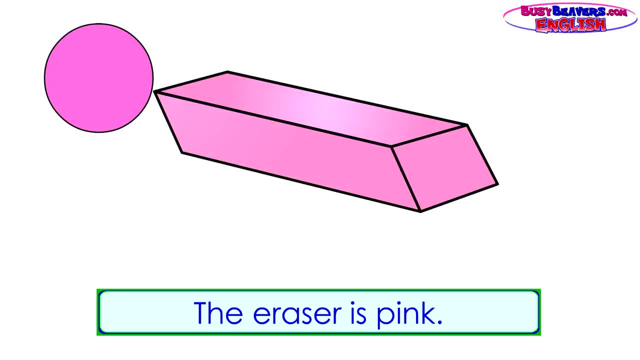 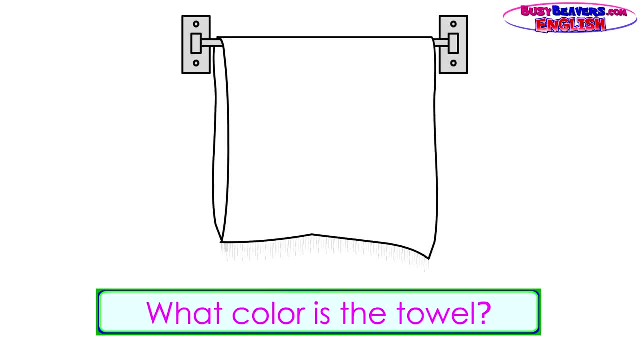 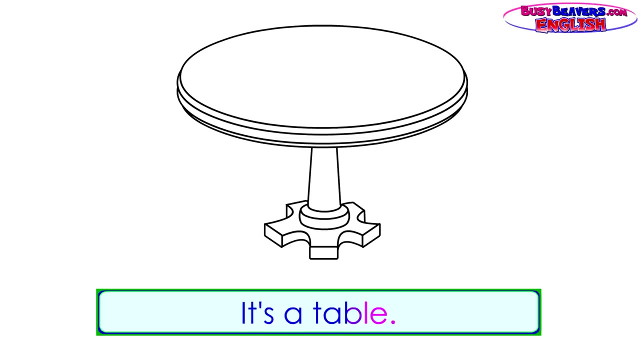 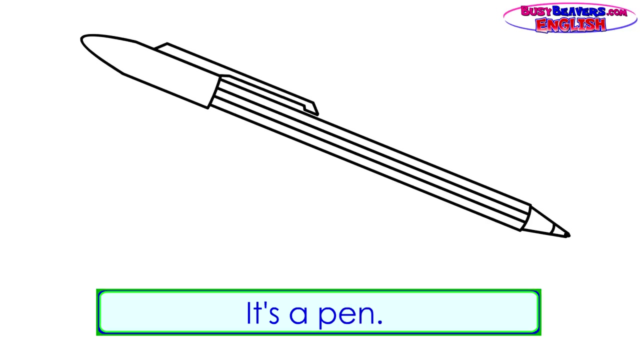 The eraser is pink. What's this? It's a towel. What color is the towel? The towel is green. What's this? It's a table. What color is the table? The table is orange. What's this? It's a pen. 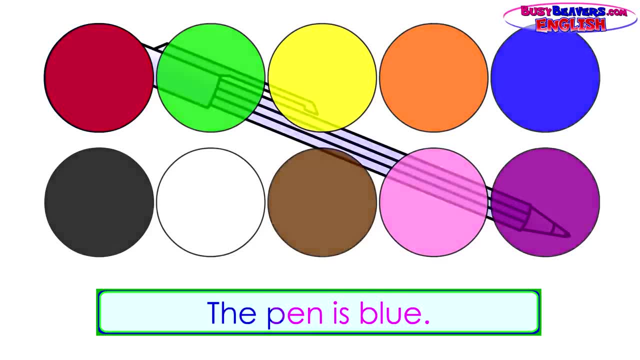 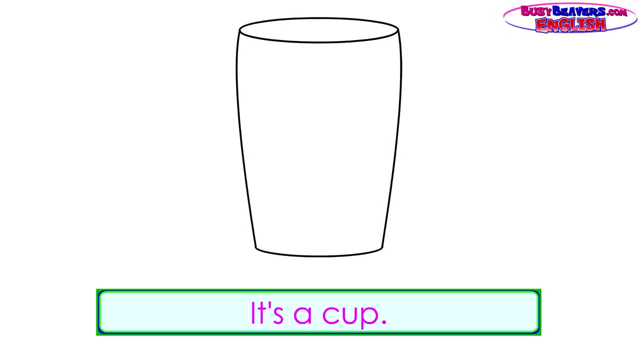 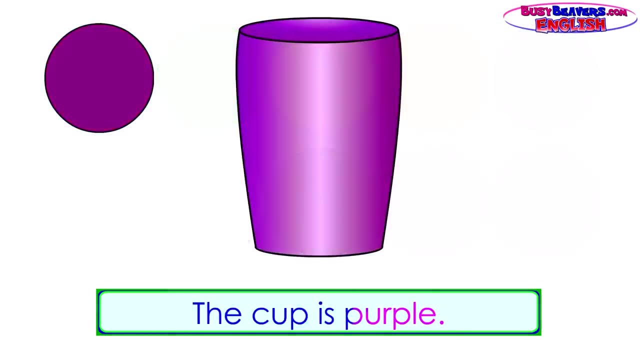 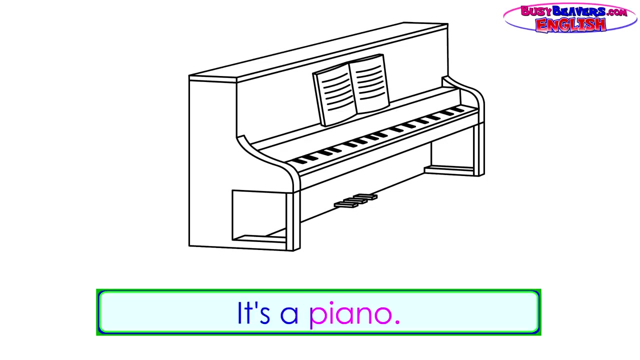 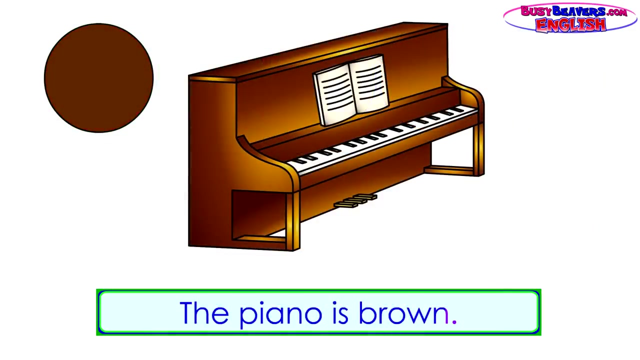 What color is the pen? The pen is blue. What's this? It's a cup. What color is the cup? The cup is purple. What's this? It's a piano. What color is the piano? The piano is brown. 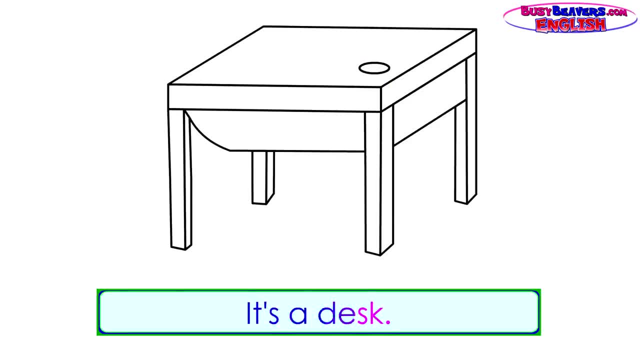 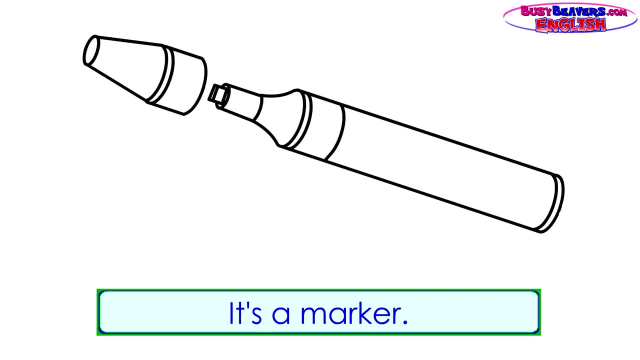 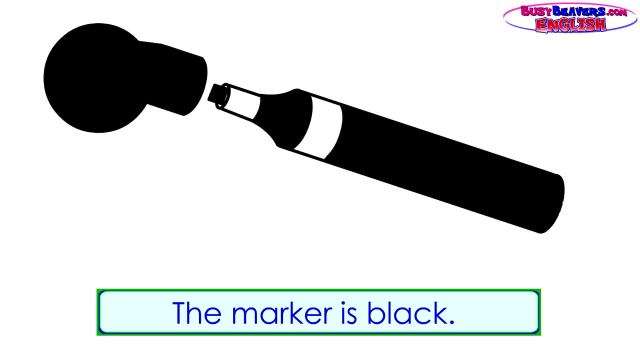 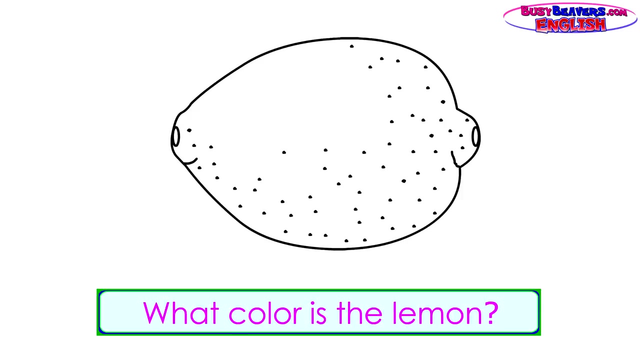 What's this? It's a desk. What color is the desk? The desk is white. What's this? It's a marker. What color is the marker? The marker is black. What's this? It's a lemon. What color is the lemon? 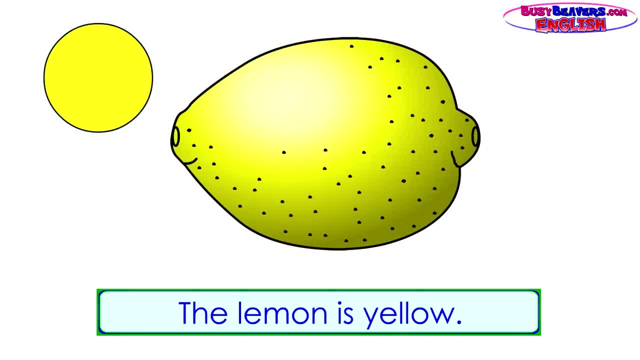 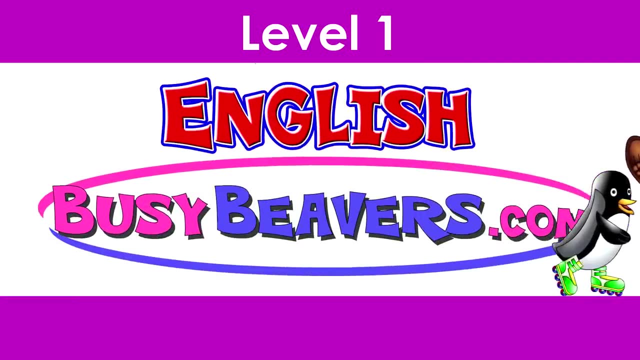 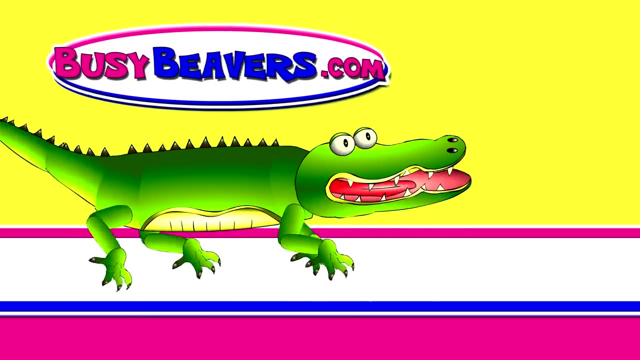 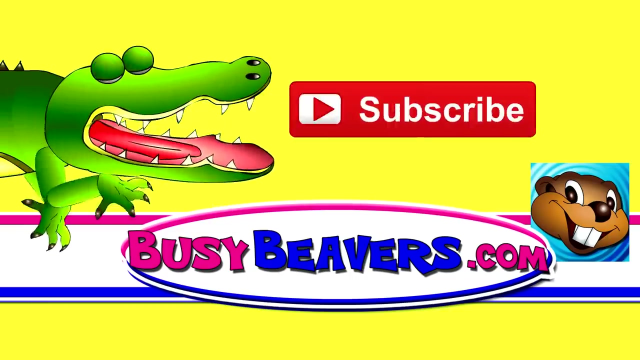 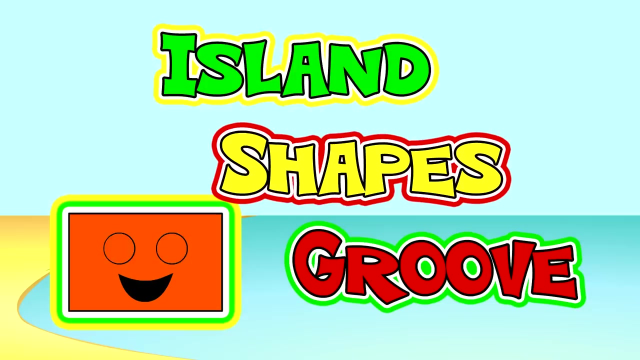 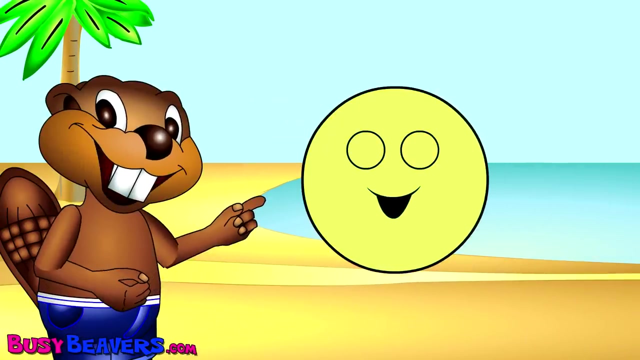 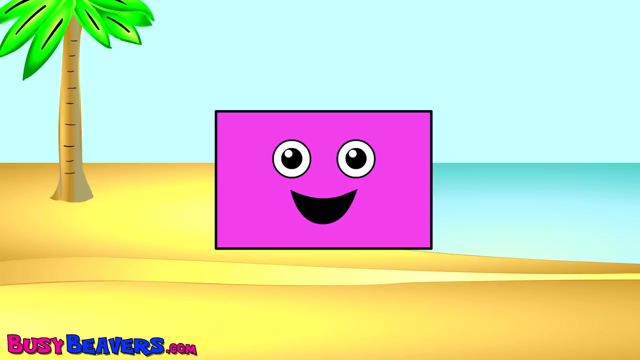 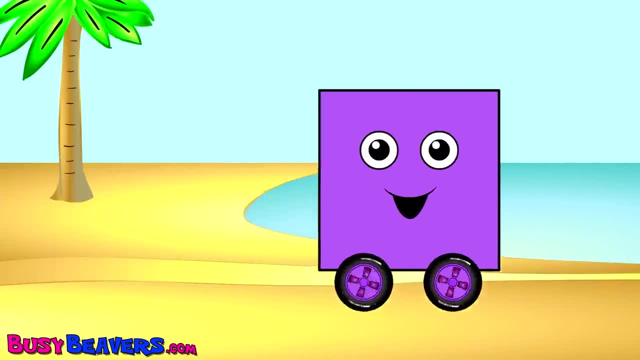 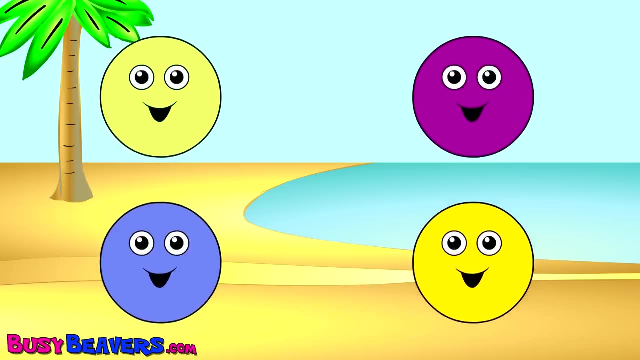 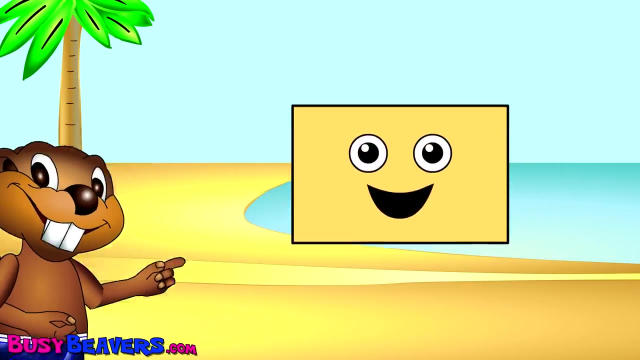 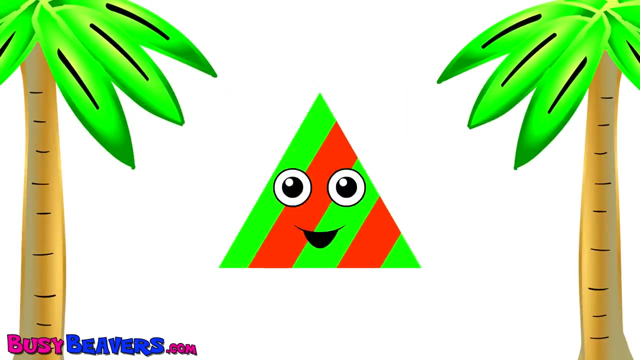 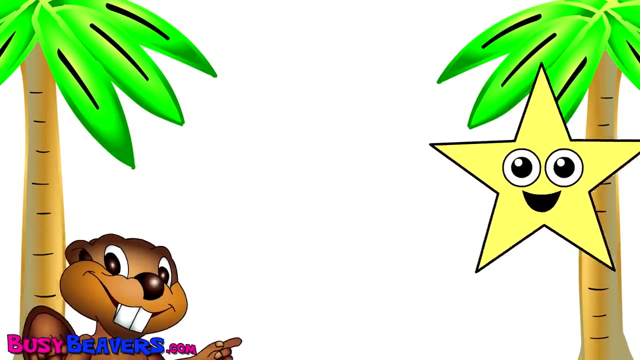 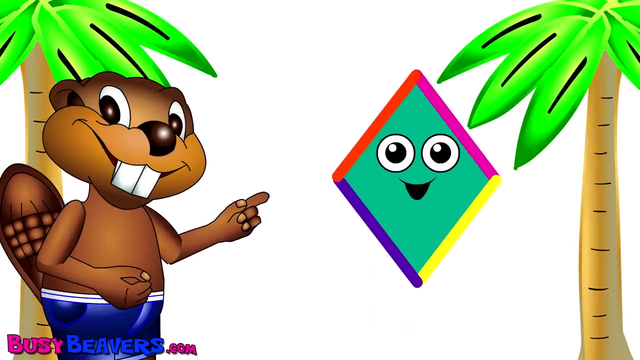 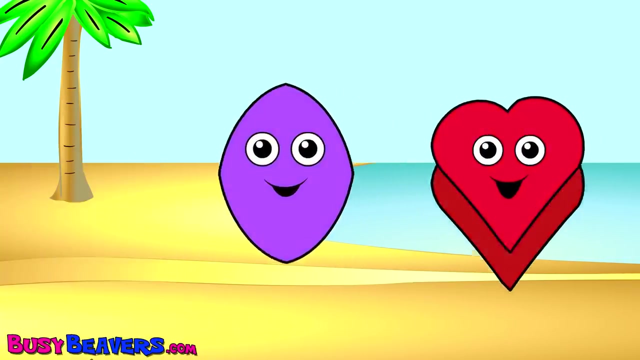 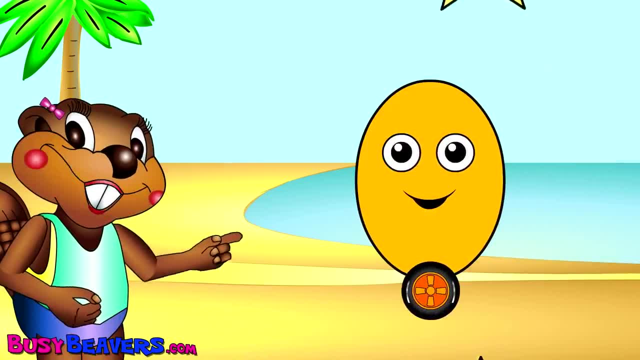 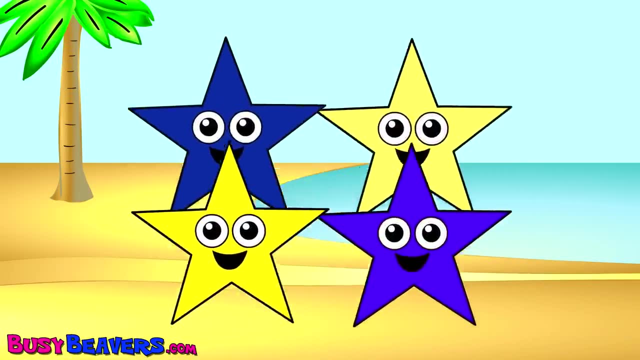 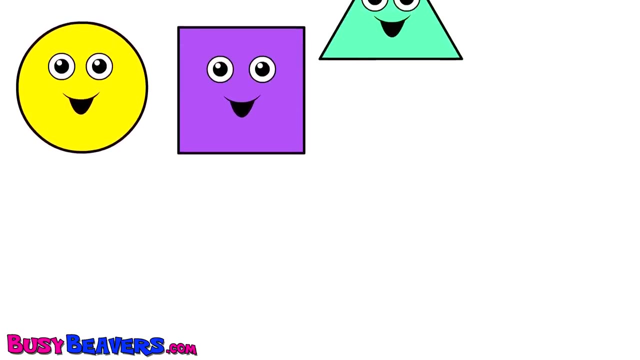 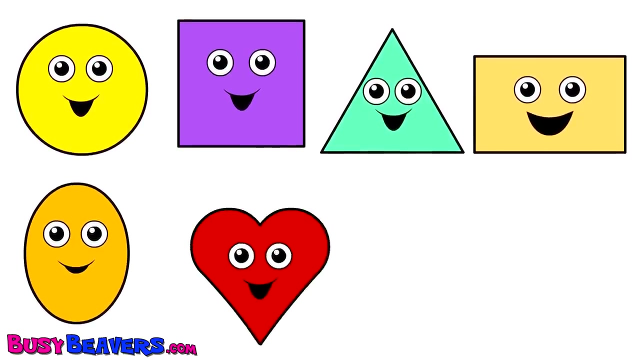 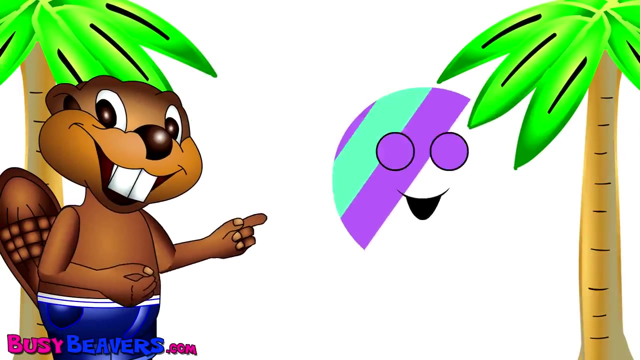 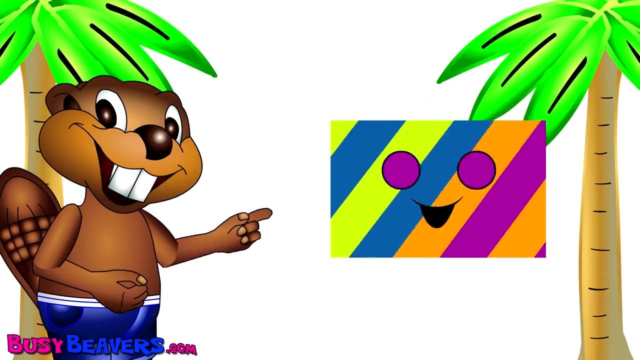 Diamond Star Star- Oval- Oval Heart- Heart- Diamond Diamond Star- superstardom Circle- square triangle- rectangle circle circle square- square triangle- rectangle star- triangle- triangle star. 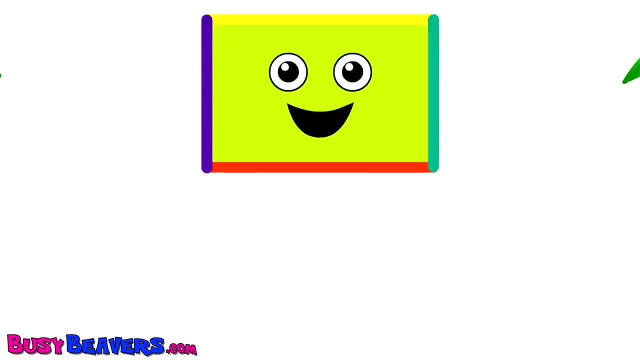 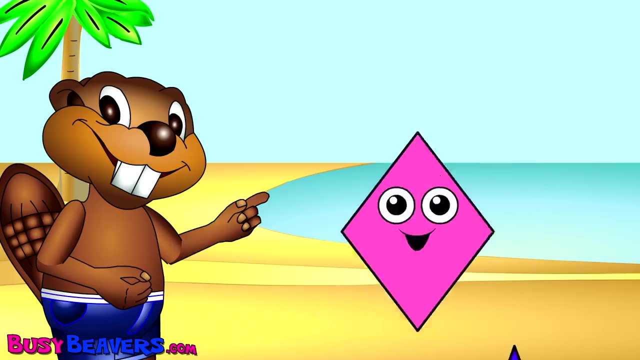 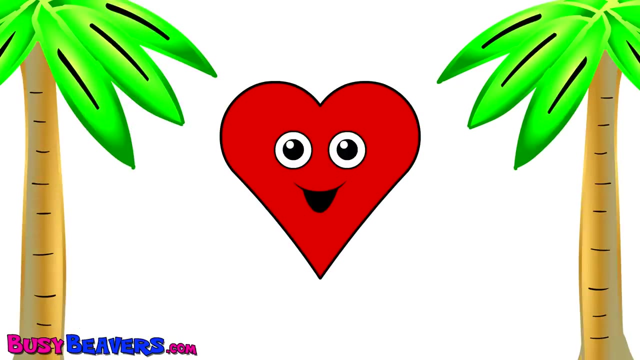 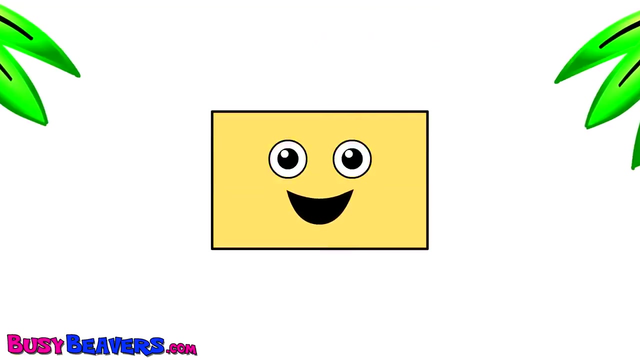 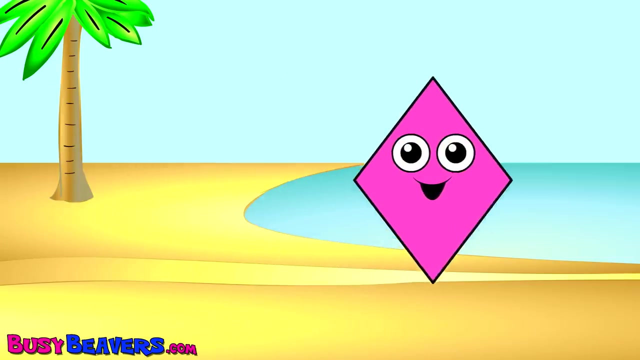 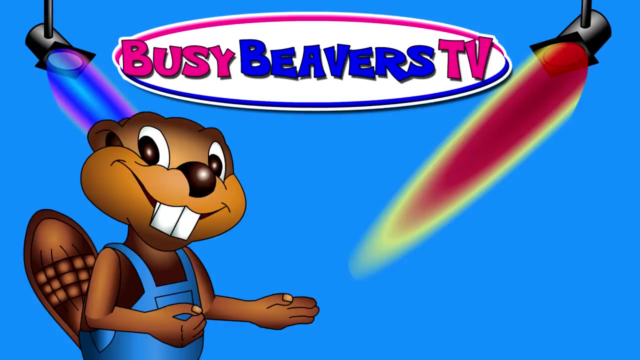 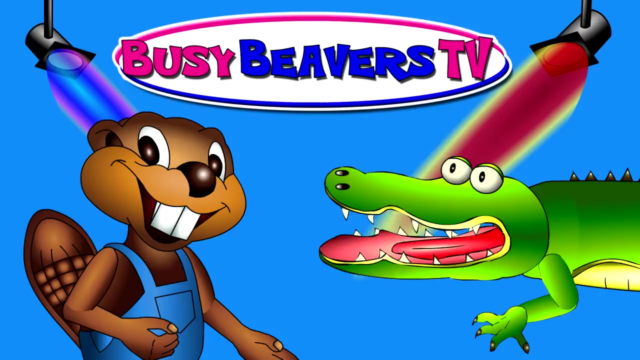 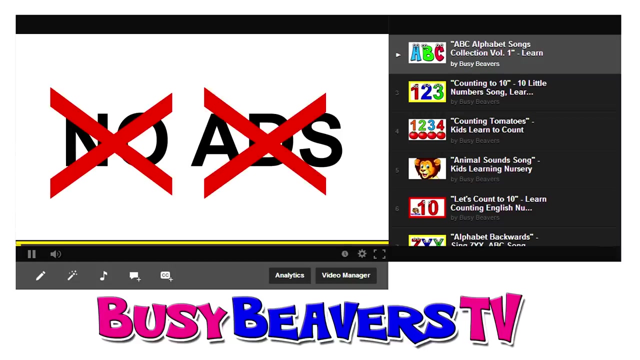 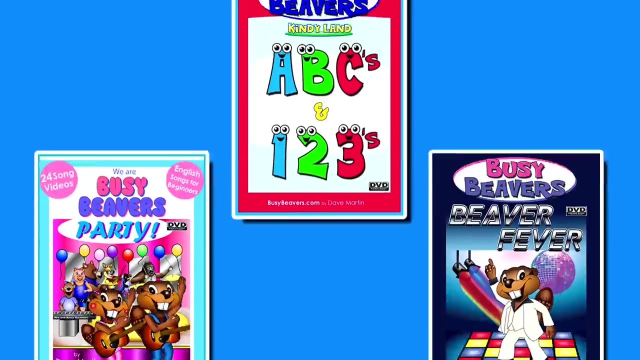 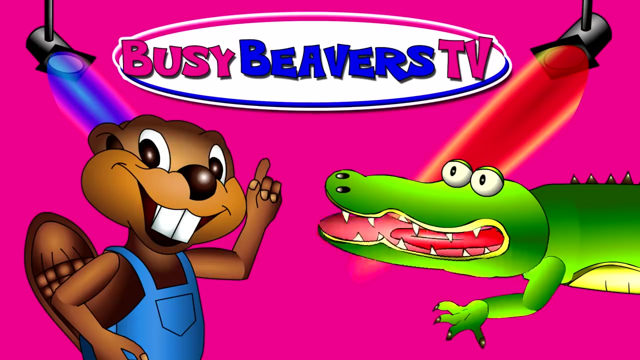 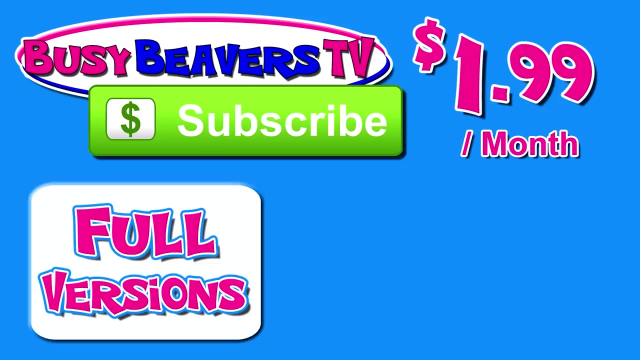 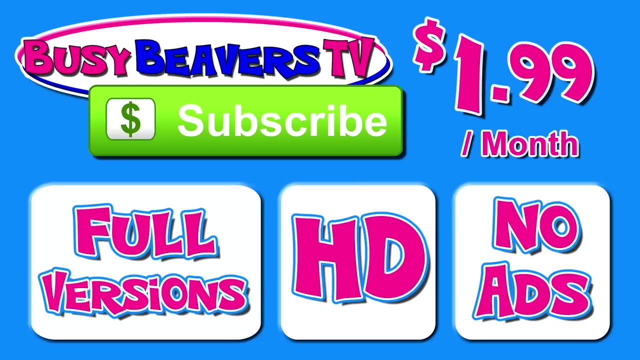 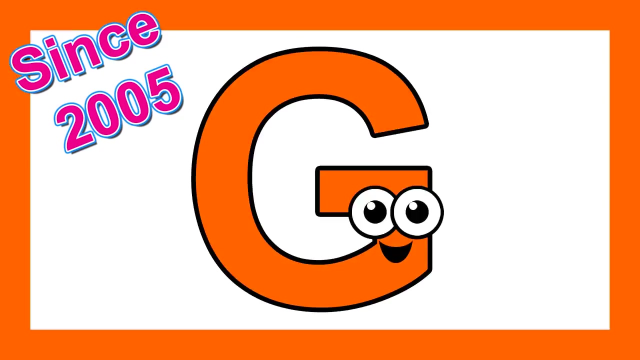 Rectangle triangle. rectangle. Oval heart diamond star. Oval oval heart- heart Diamond diamond star. Oval oval diamond star. Oval oval diamond star. Oval oval diamond star. Since 2005, children all around the world have been learning their ABCs. 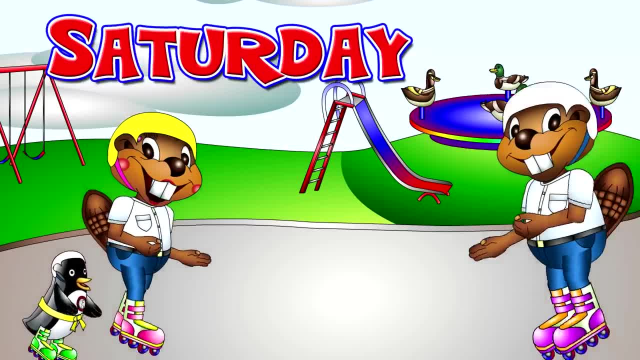 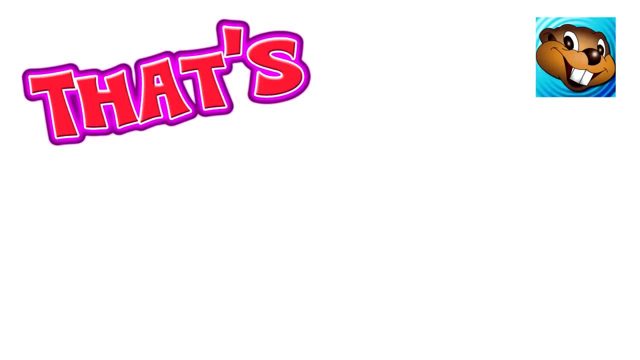 1-2-3s, colors shapes, days of the week and more with Busy Beavers. Our videos have been seen over 500 million times on YouTube. Now that's education gone viral. Tell them about the new languages we teach. 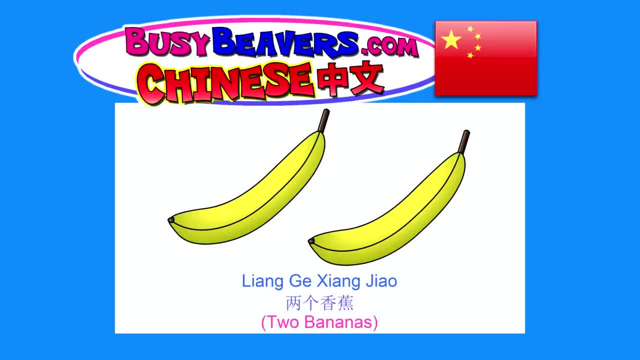 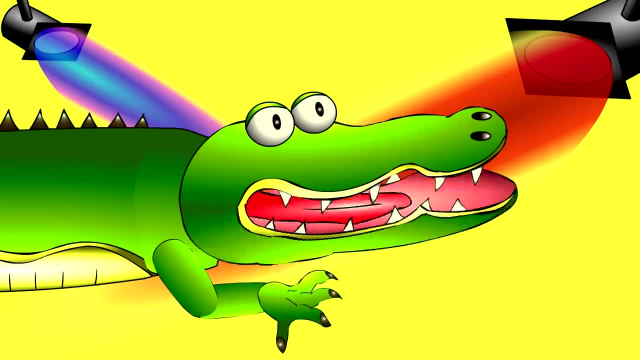 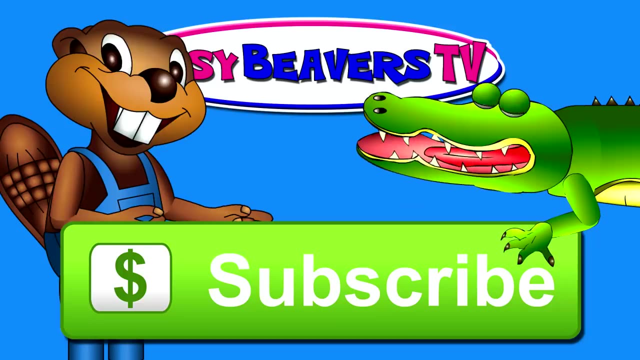 Right, We've translated our English learning videos into Chinese, French, Korean and many more languages coming soon. It's a global community after all. Oh, that's totally worth $2.. You can try it out first before you buy. Too late, I just subscribed. 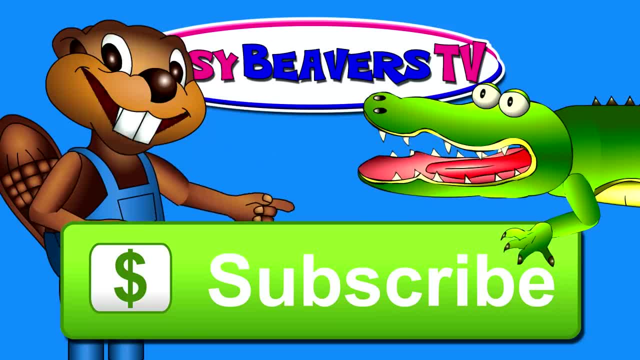 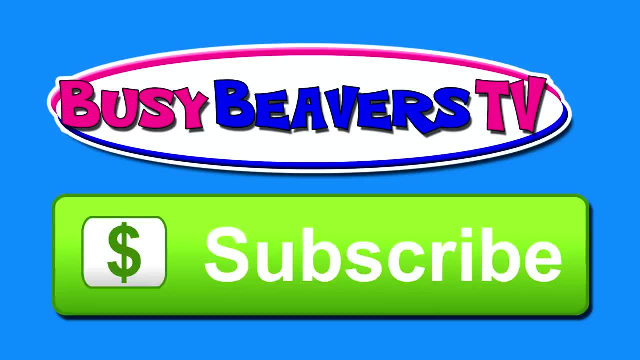 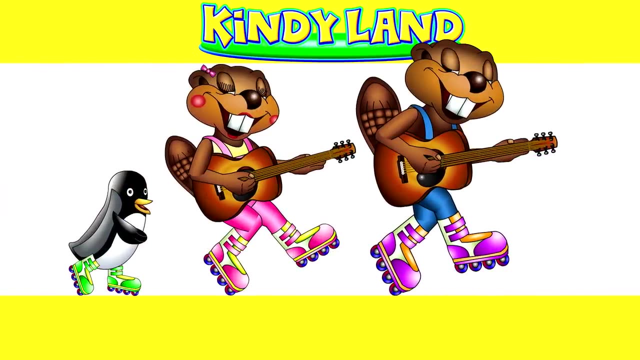 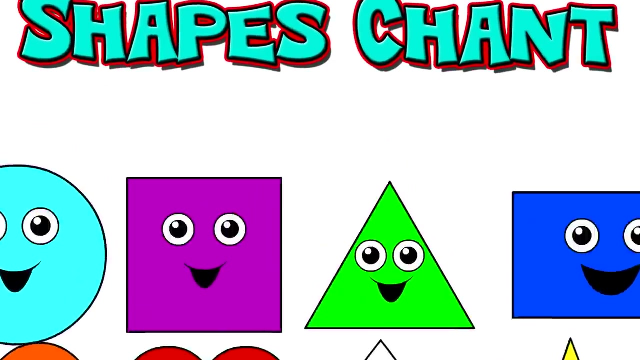 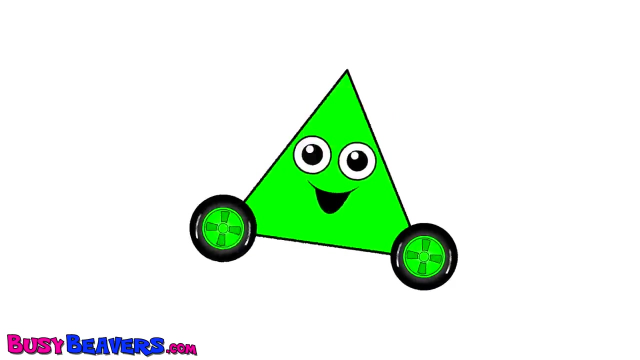 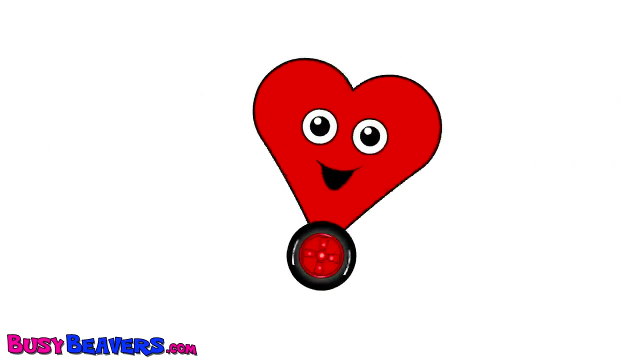 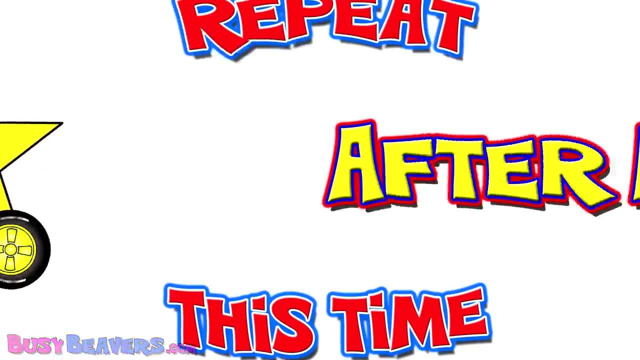 Looks like he's a Busy Beaver. Click this button and you can be a Busy Beaver too. Thanks for watching. See you next time. Shapes, chant, Circle, Square, Triangle, Rectangle, Oval Heart, Diamond Star- Repeat after me this time. 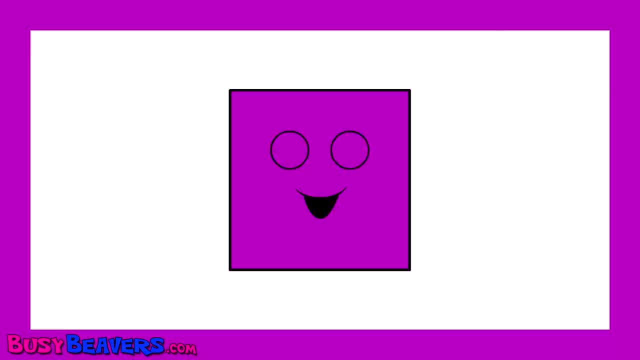 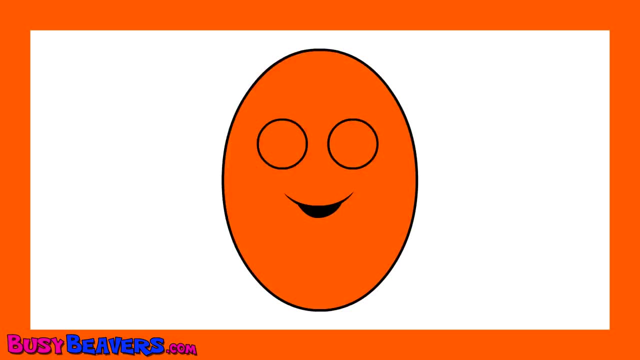 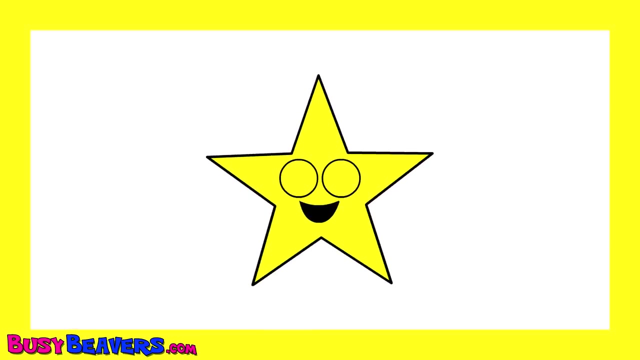 Circle, Circle, Square, Square, Triangle, Triangle, Rectangle, Rectangle, Oval, Oval, Heart, Heart, Diamond, Diamond, Star, Star. Let's be really quiet this time. Circle, Circle, Square, Square, Triangle, Triangle. 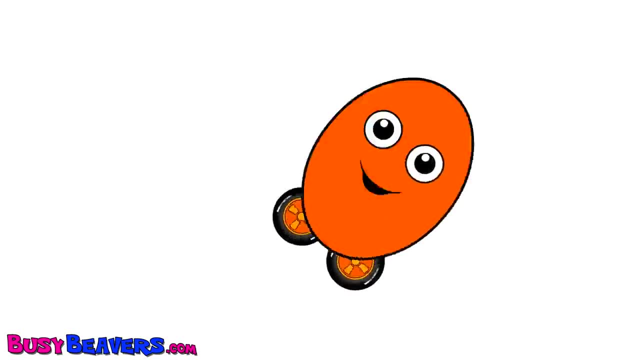 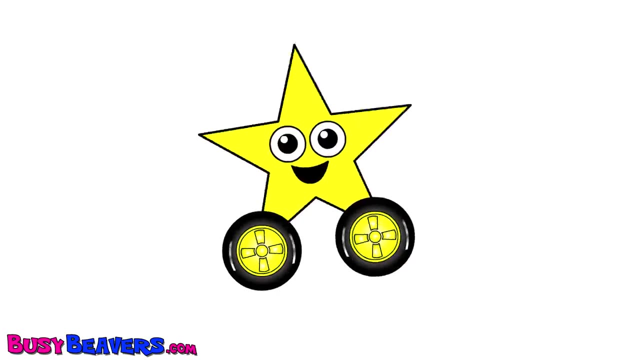 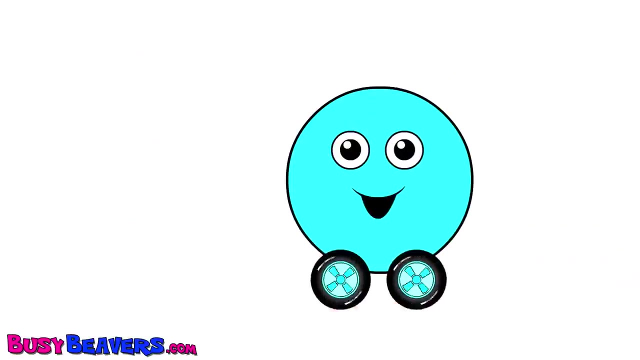 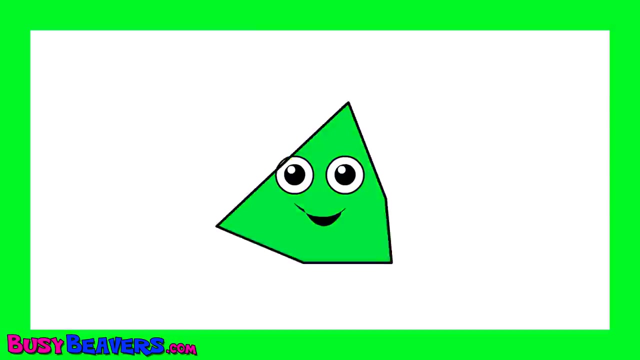 Rectangle, Rectangle, Rectangle, Oval, Oval, Oval, Heart, Heart, Diamond, Diamond, Star, Star, Star. Let's try it even quieter: Circle, Circle, Square, Square, Triangle, Triangle, Rectangle, Rectangle, Oval. 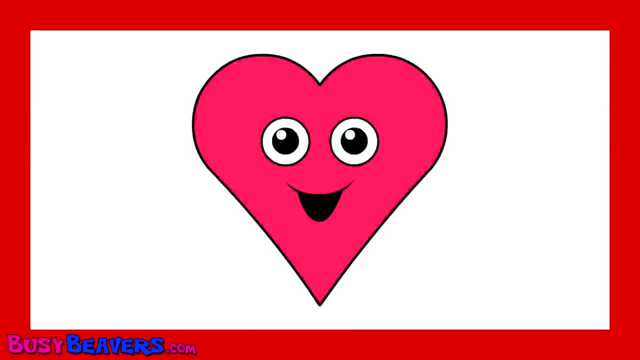 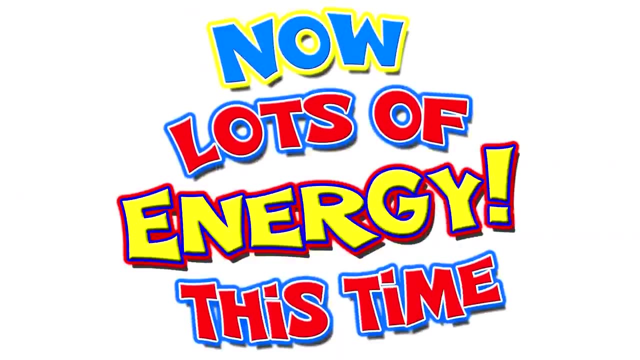 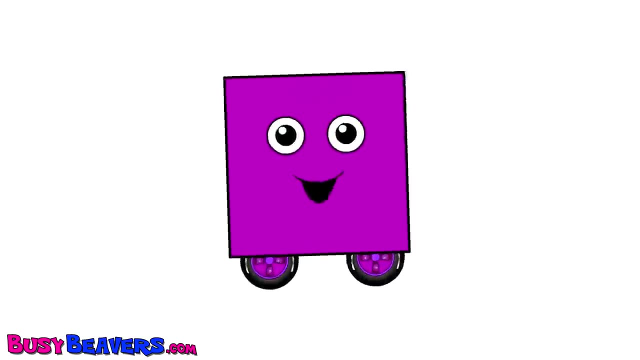 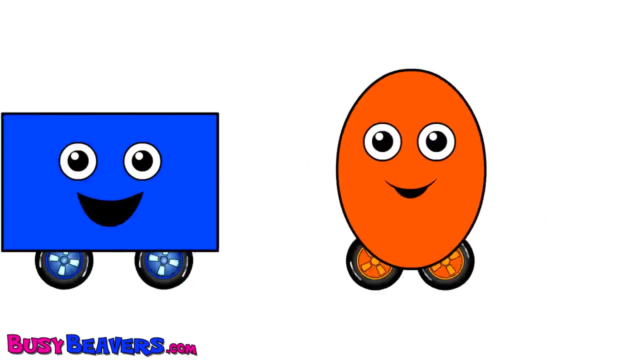 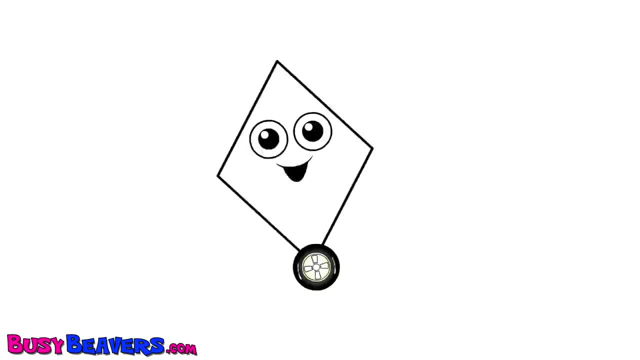 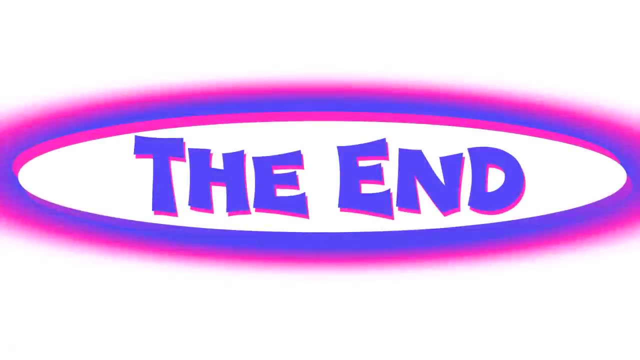 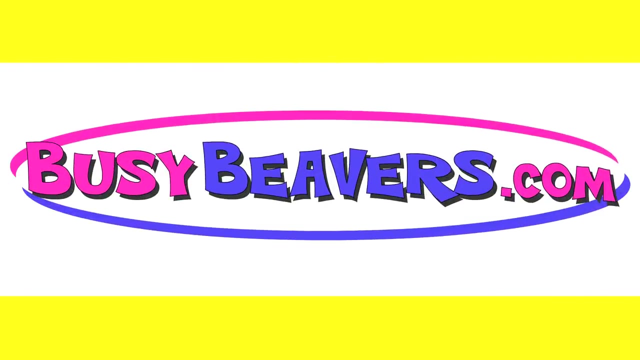 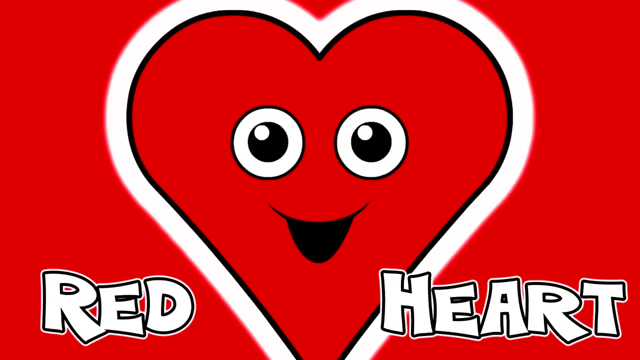 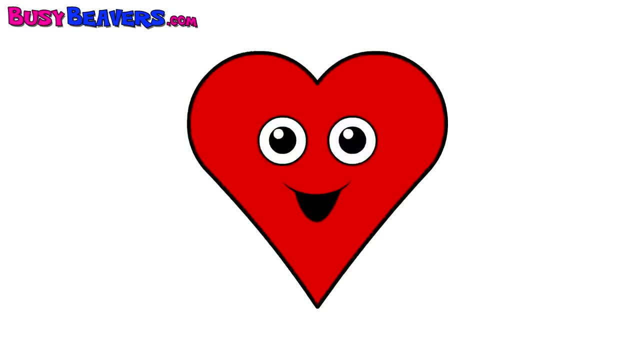 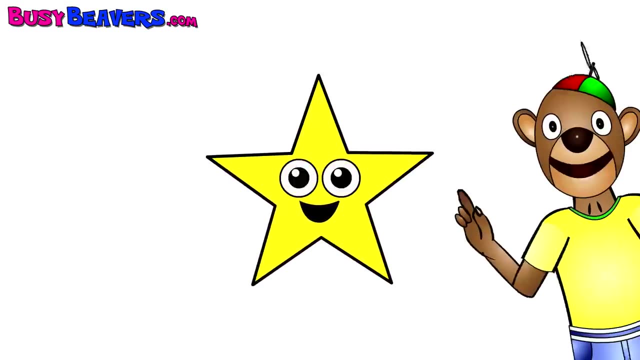 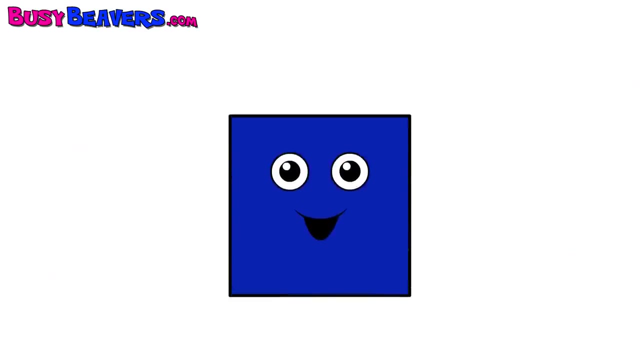 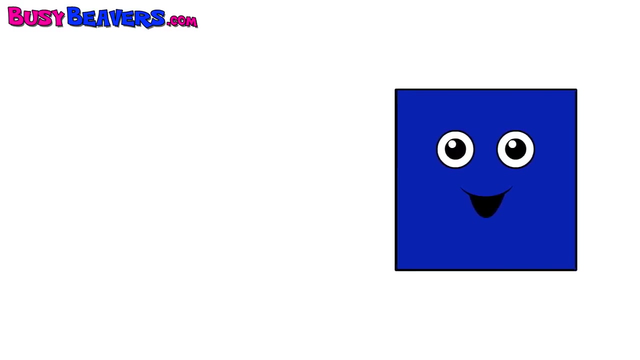 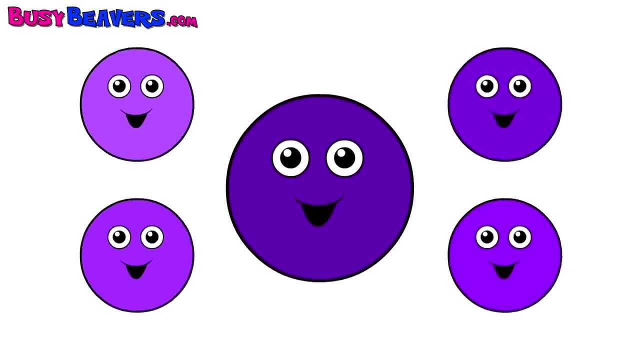 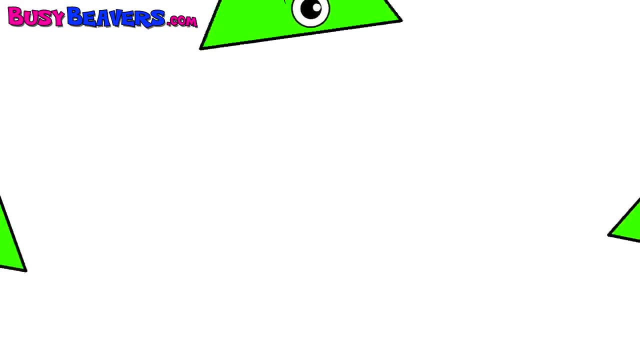 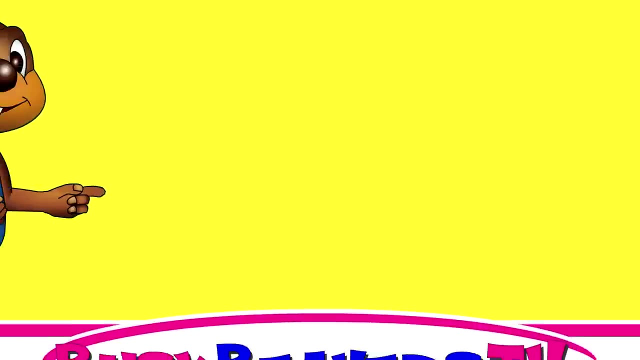 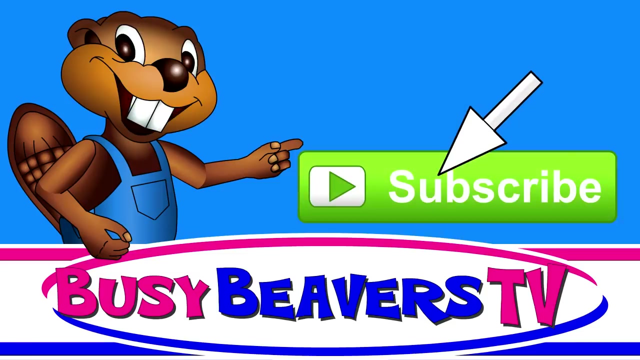 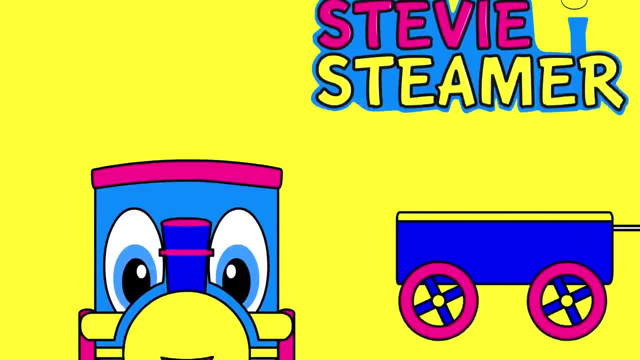 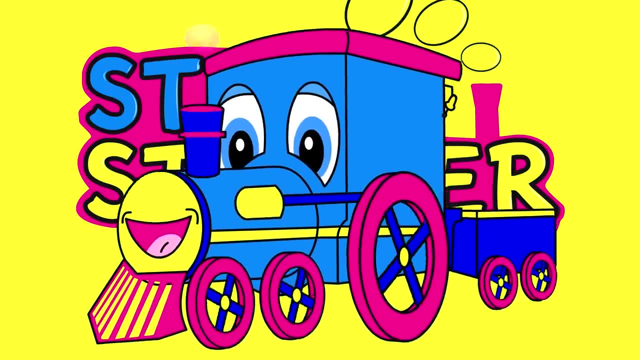 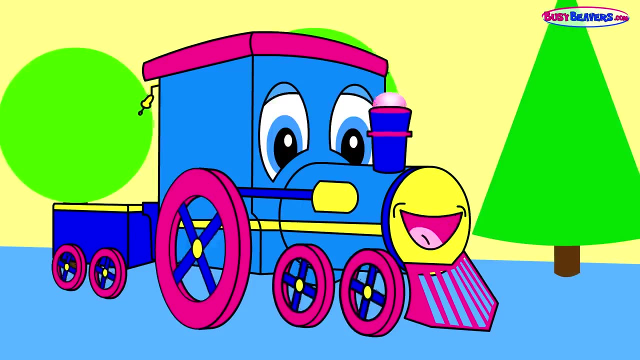 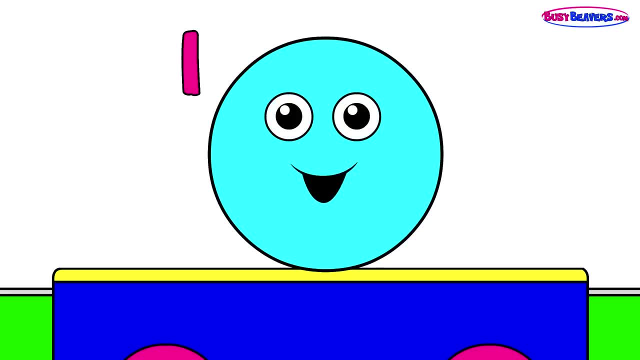 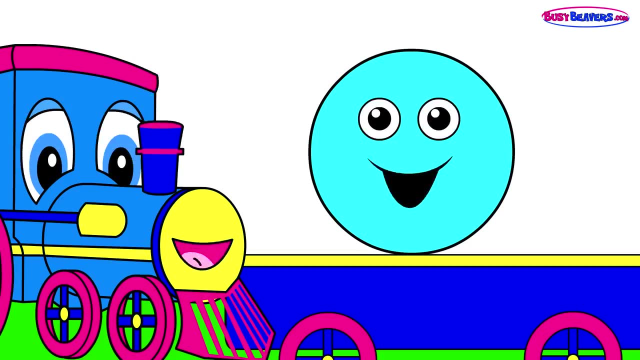 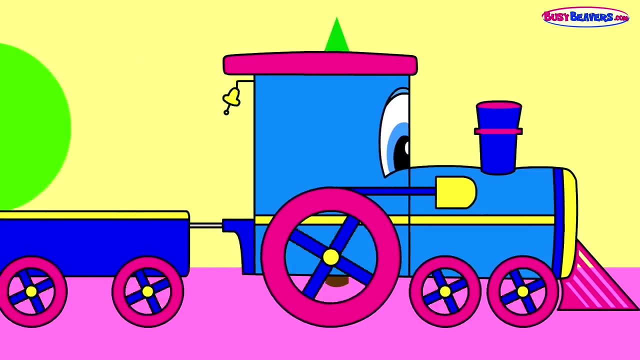 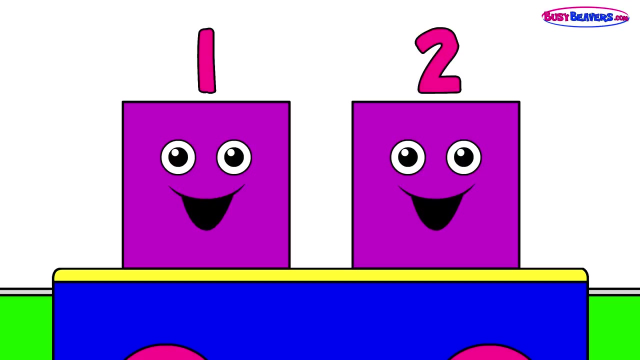 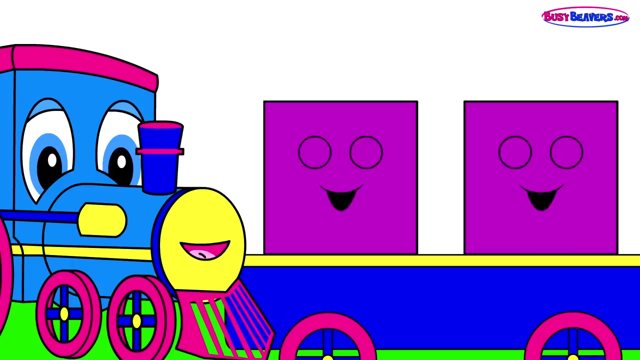 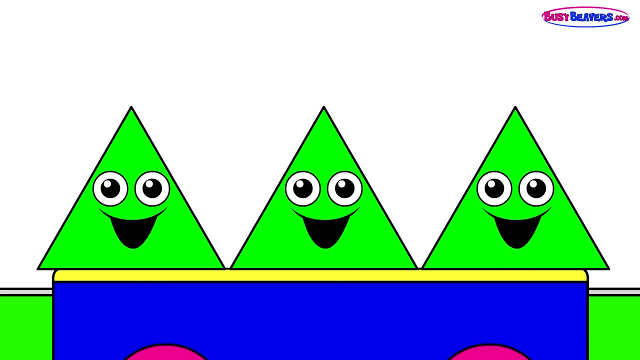 Circle One, One circle, Hello, circle, Hello Stevie, Cool circle. Squares One, Two, Two, squares, Hi, squares, Hi Stevie, Steamer Squares. Triangles One, Two, Three. 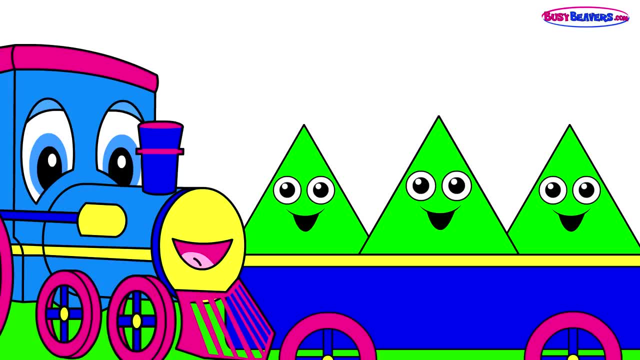 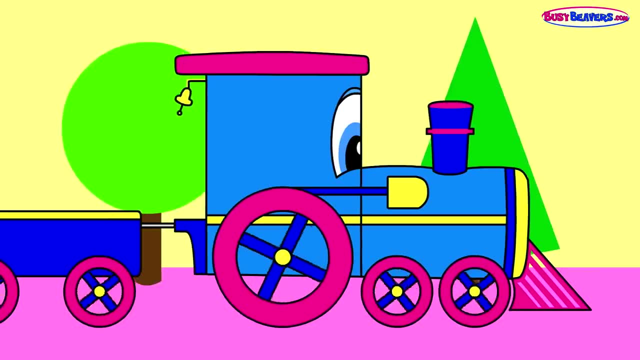 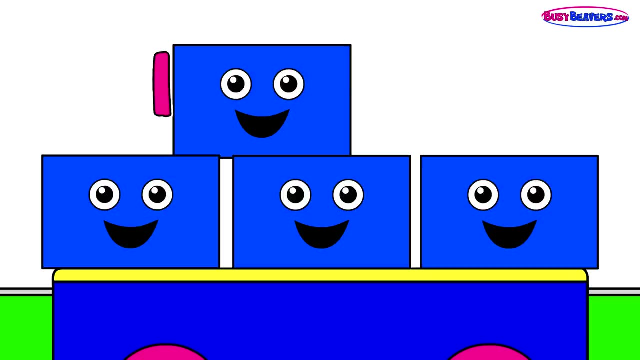 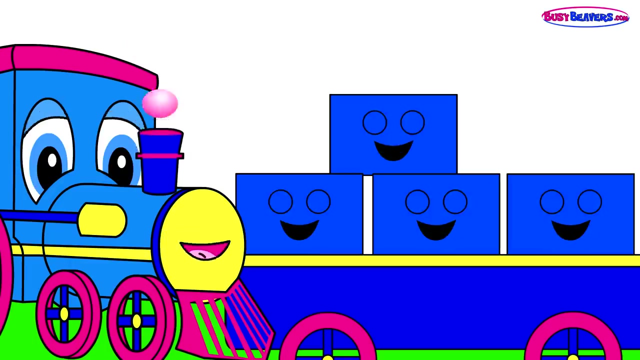 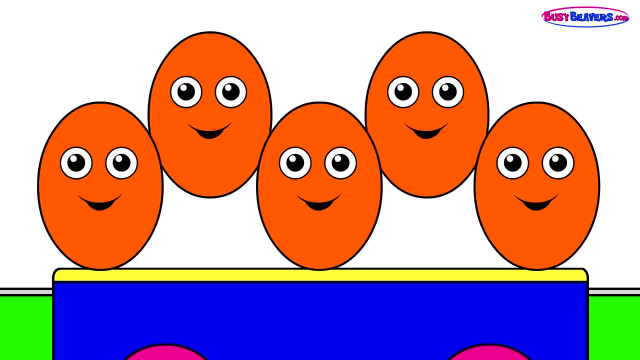 Three triangles, Hello triangles, Hello Nice shapes. Rectangles: One, Two, Three, Four, Four. rectangles, Hi, rectangles, Hi. Stevie Steamer Love the rectangles Ovals. One, Two, Three, Four. 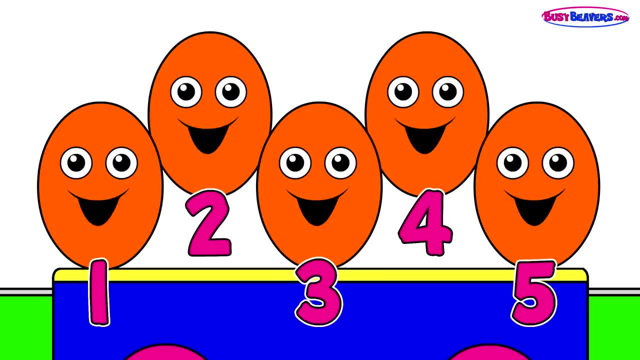 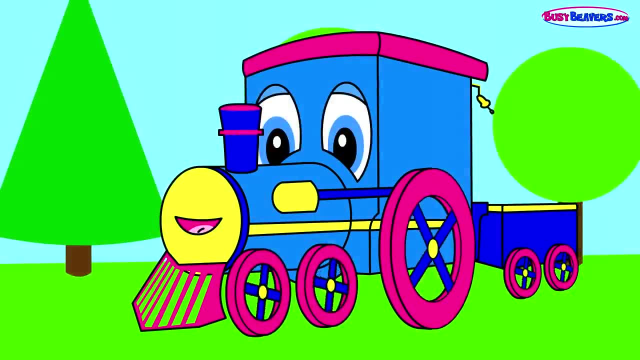 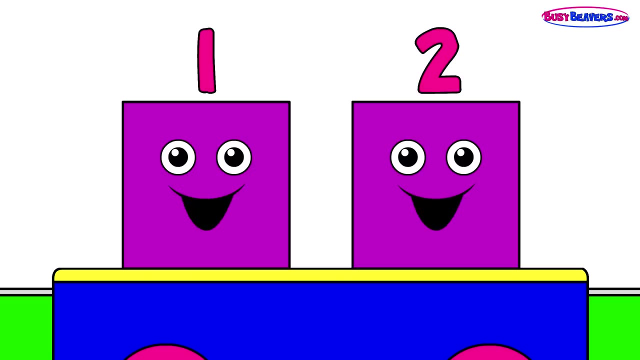 Five, Five ovals, Hey, ovals. Well, that's all the shapes for today. Let's count them one more time: One circle, One, two squares. One, two, three triangles. One, two, three triangles. 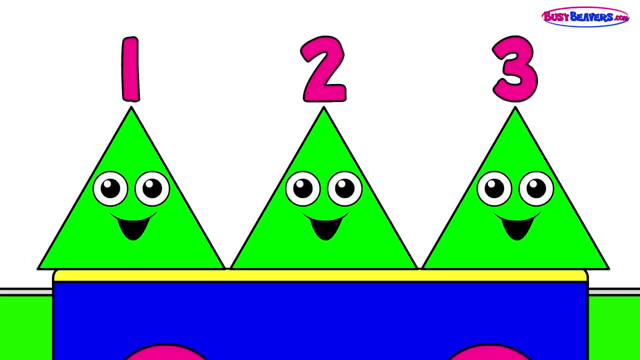 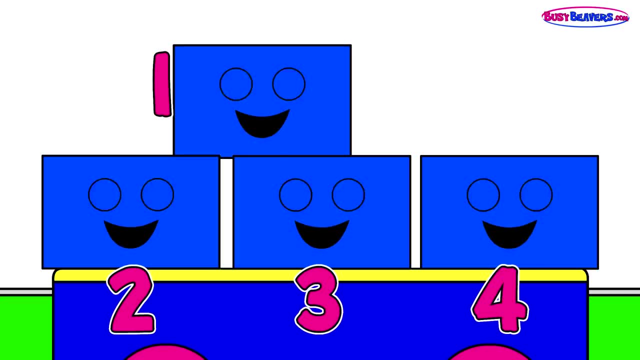 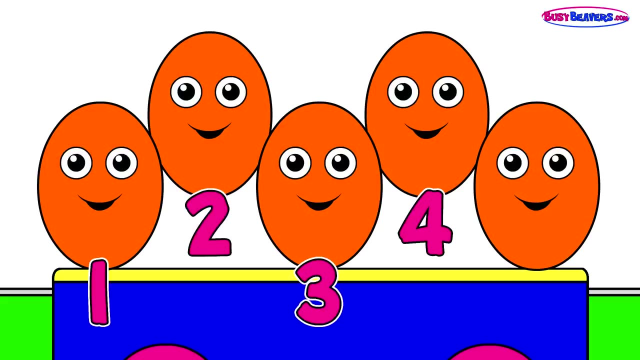 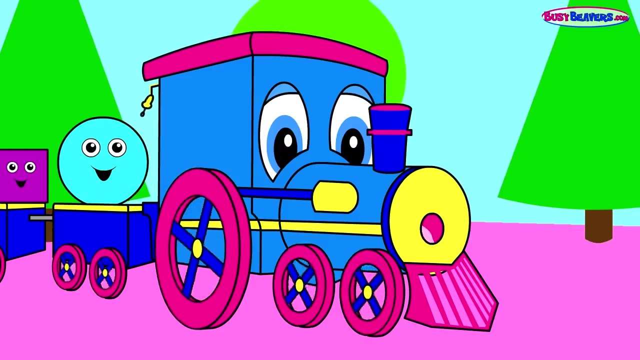 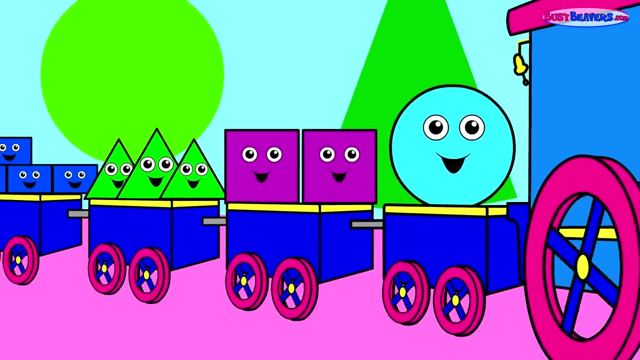 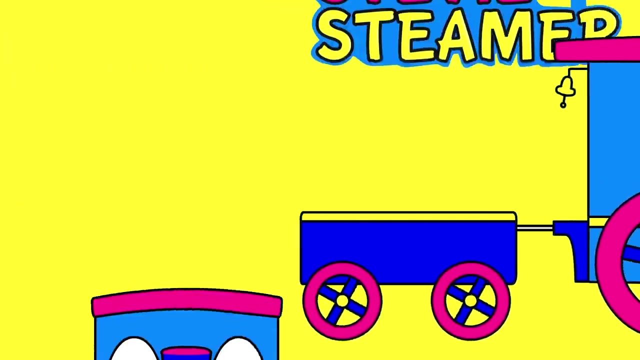 One, two, three triangles. One, two, three, four rectangles. One, two, three, four, five ovals. All aboard, Here we go. Steamy steamer, That's my name. Steamy steamer, I'm a train. 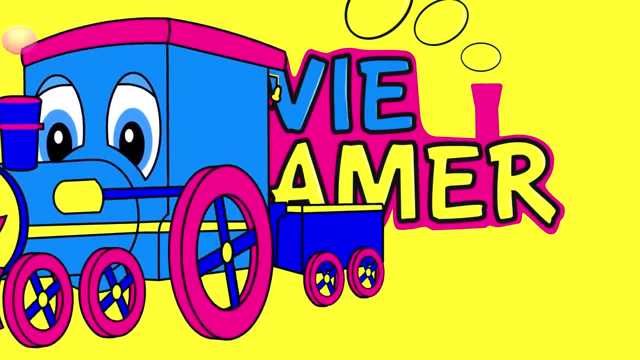 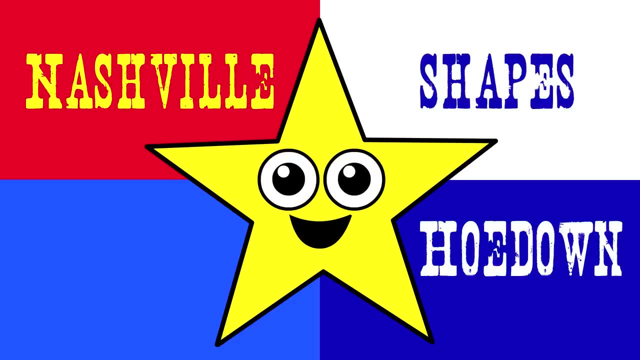 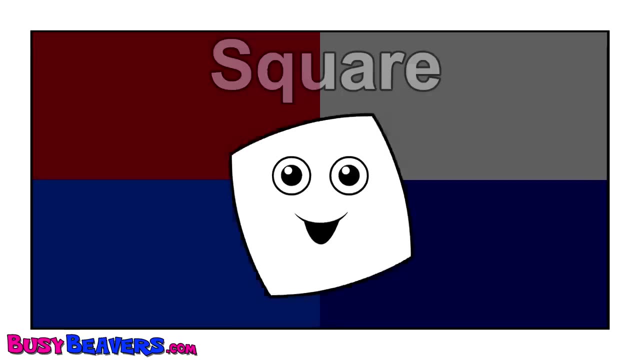 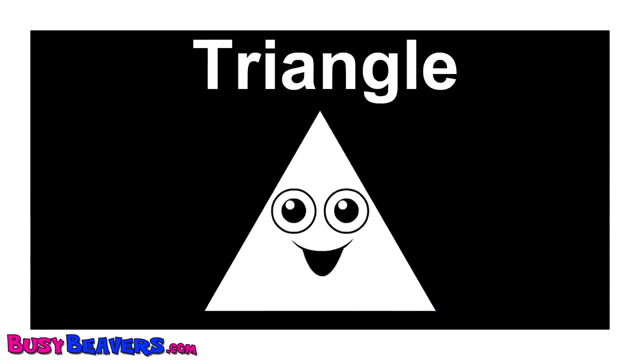 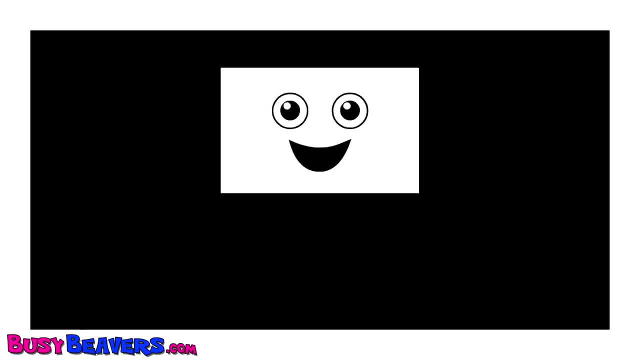 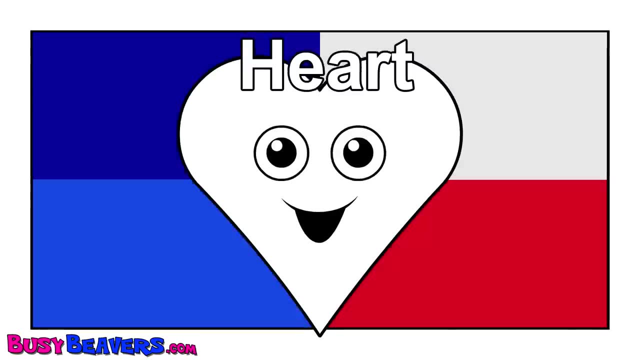 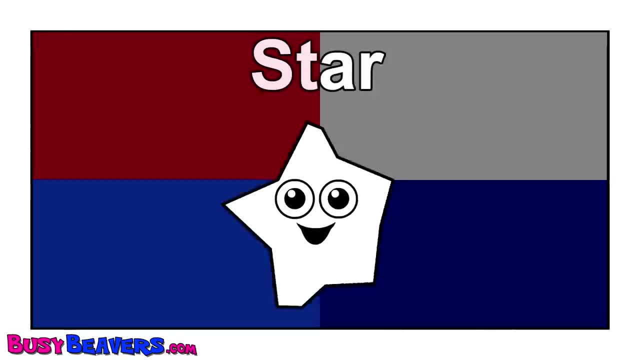 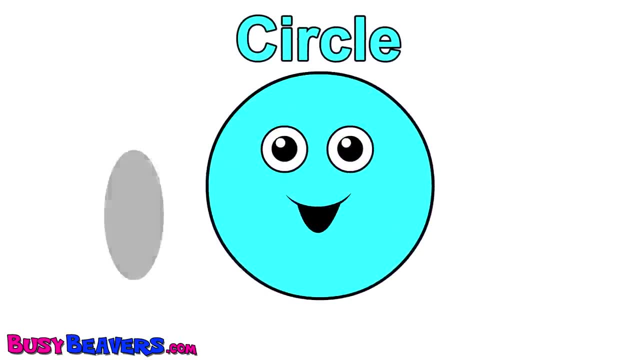 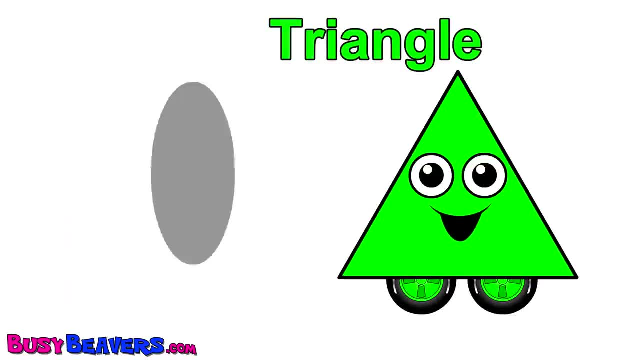 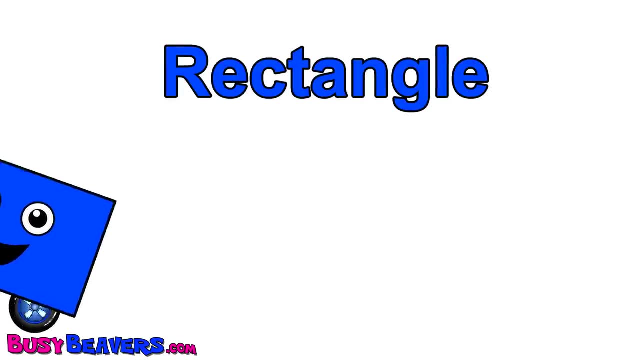 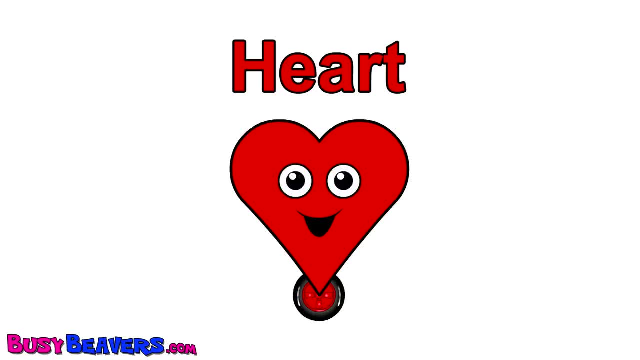 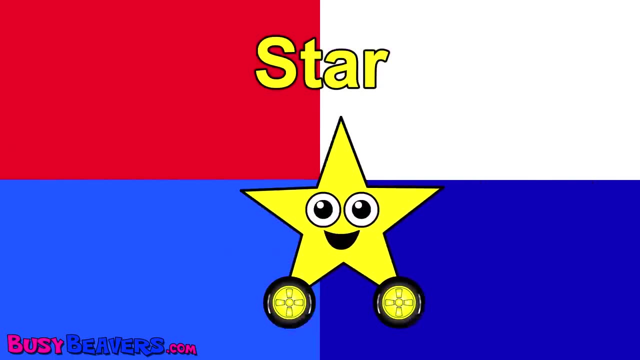 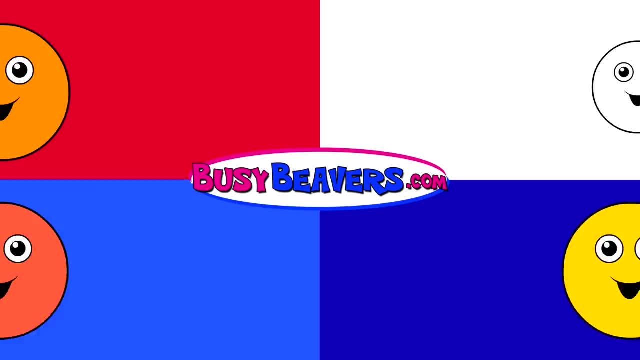 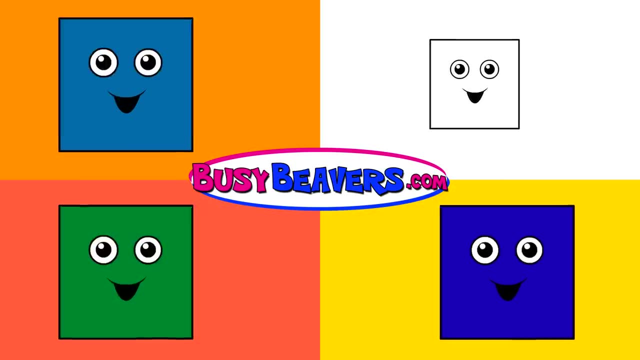 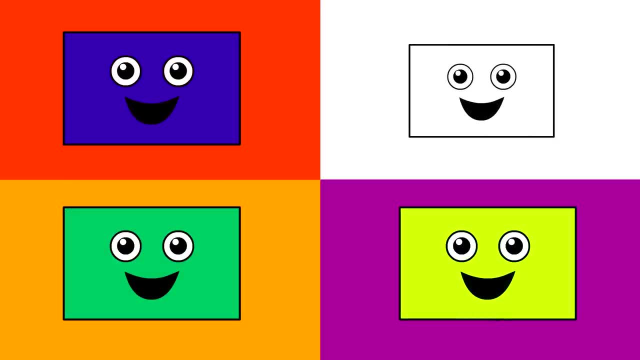 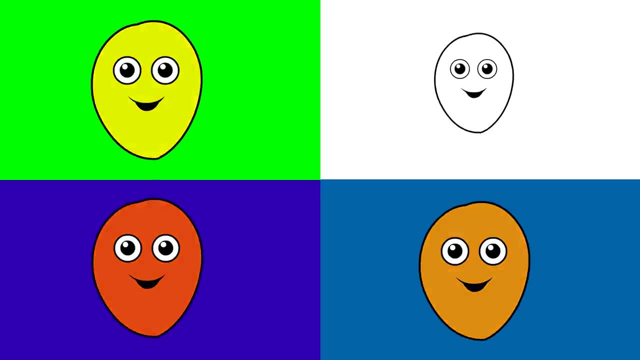 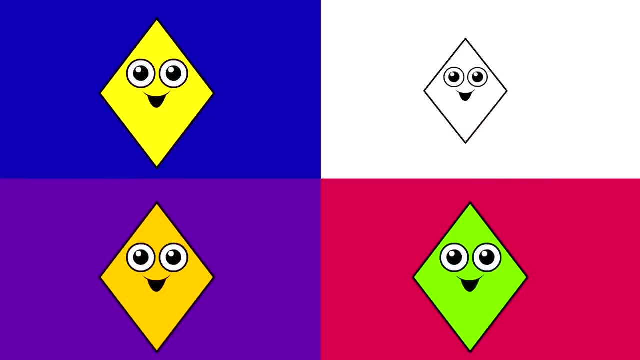 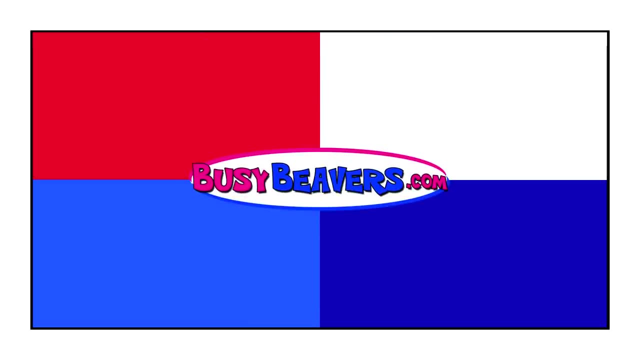 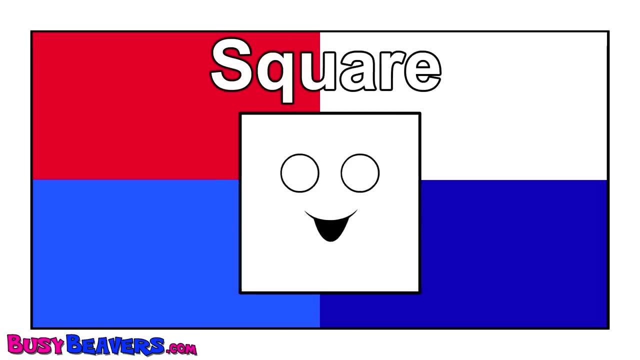 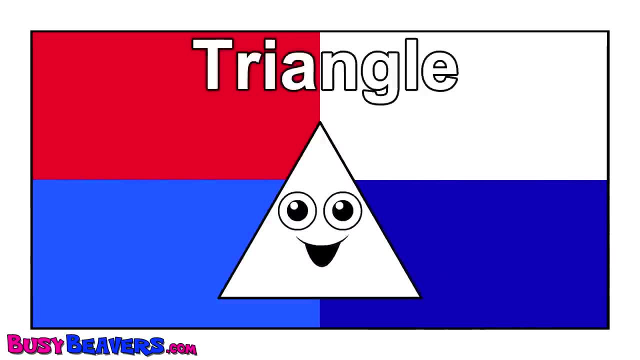 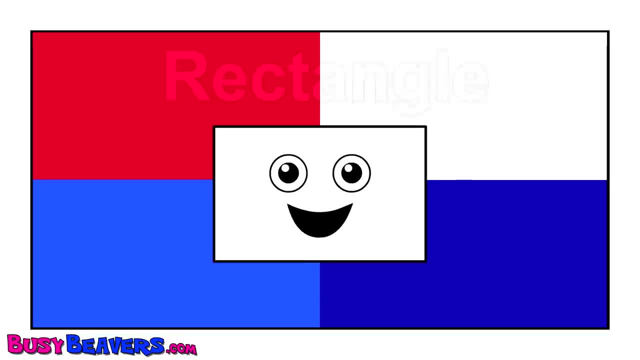 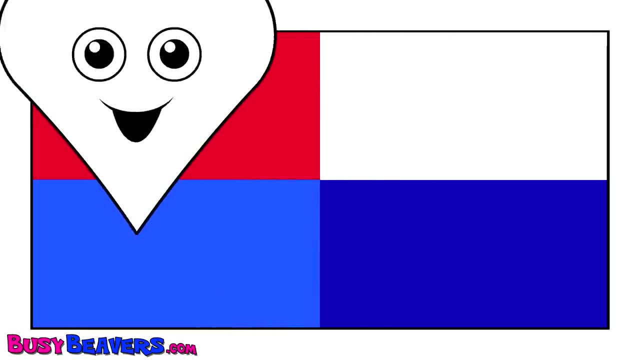 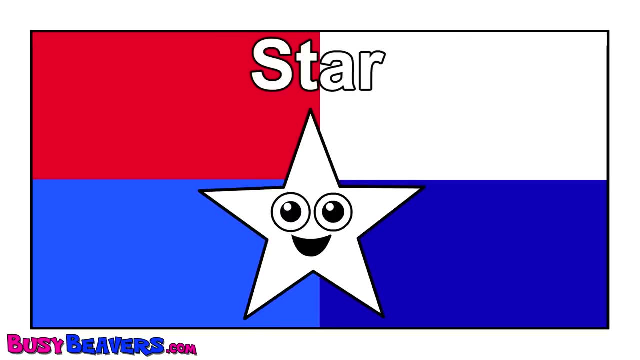 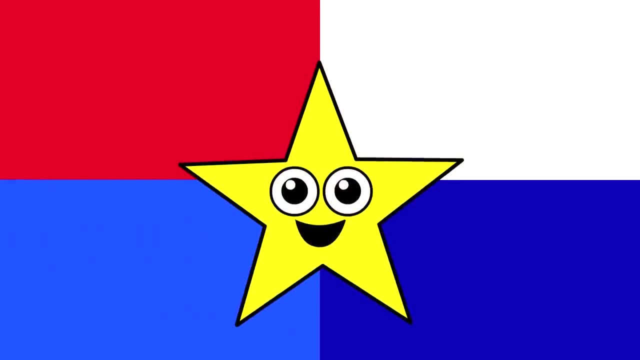 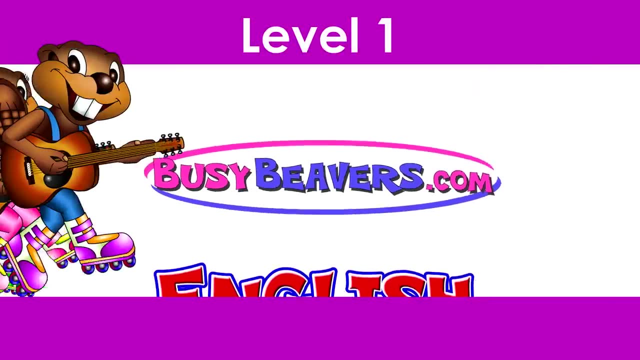 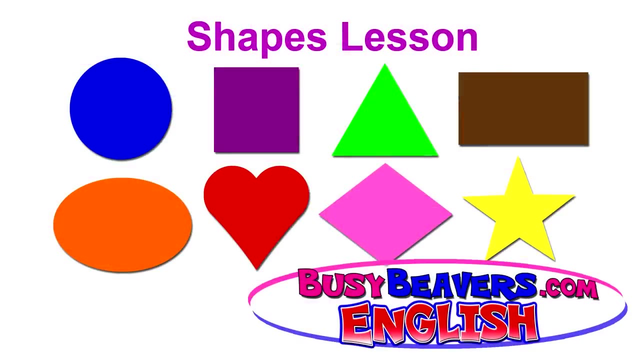 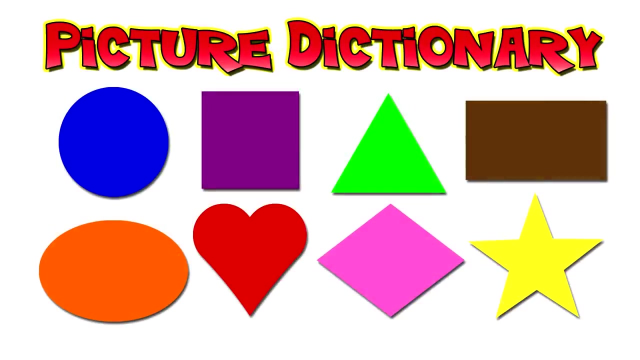 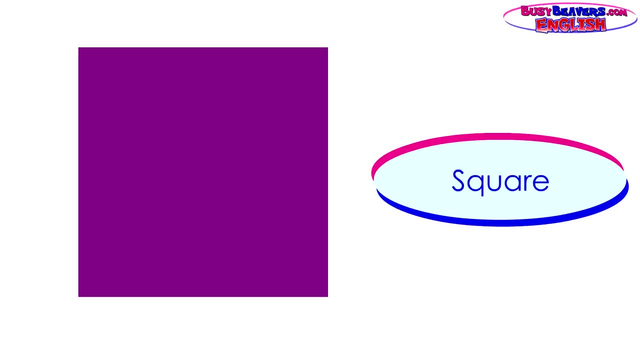 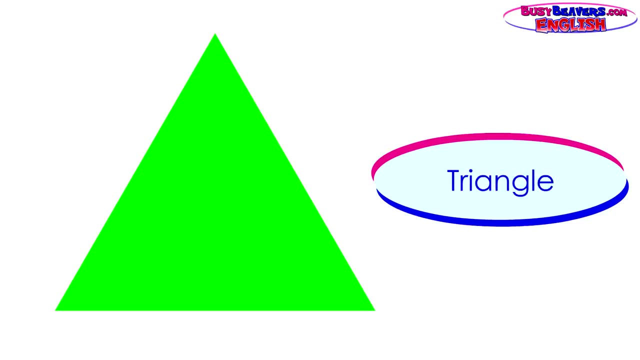 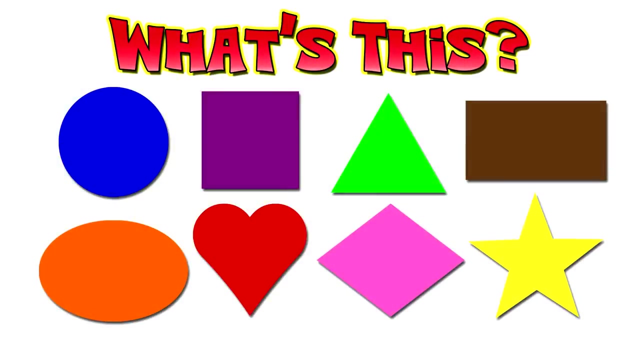 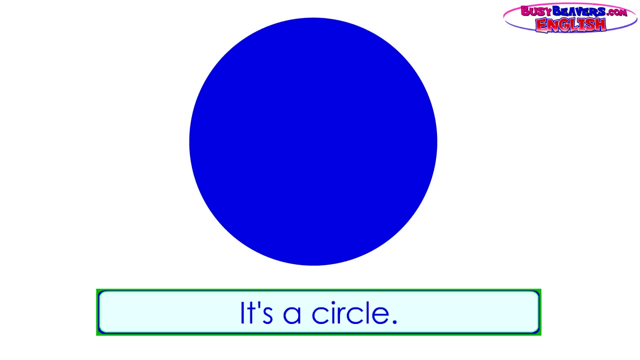 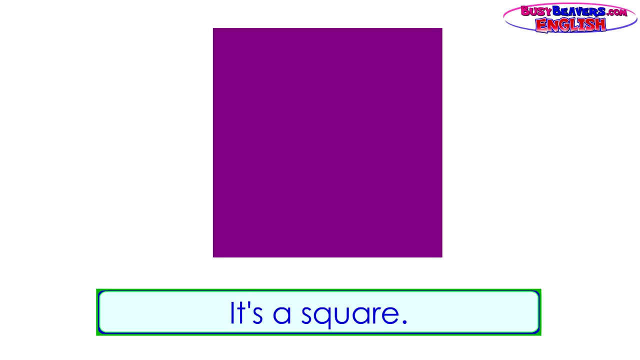 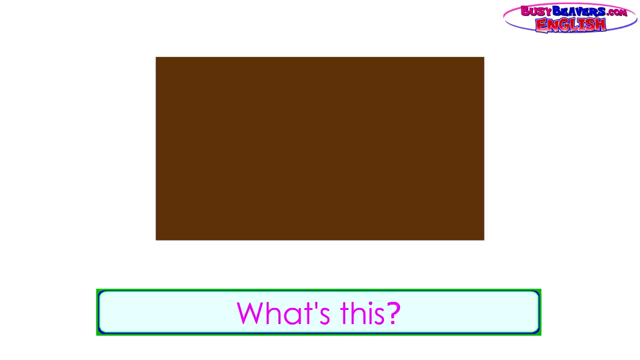 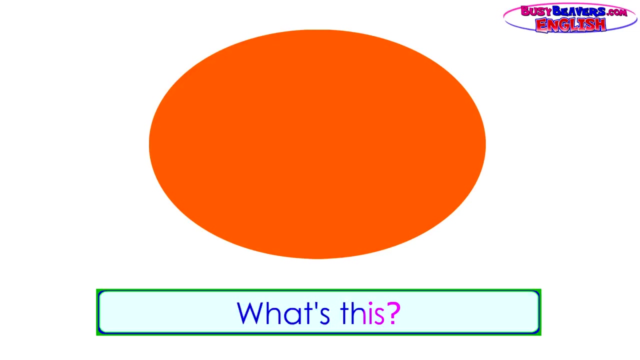 Circle Square Square, Triangle, Triangle, Rectangle, Oval Heart, Diamond Star. What's this? It's a circle. What's this? It's a square. What's this? It's a triangle. What's this? It's a rectangle. What's this? It's an oval. 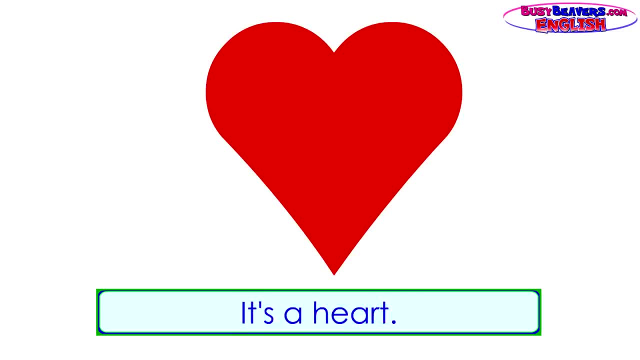 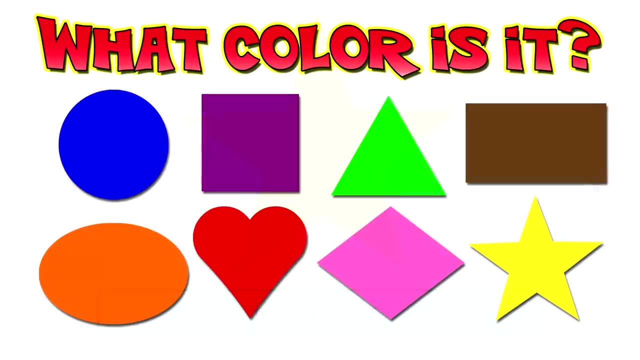 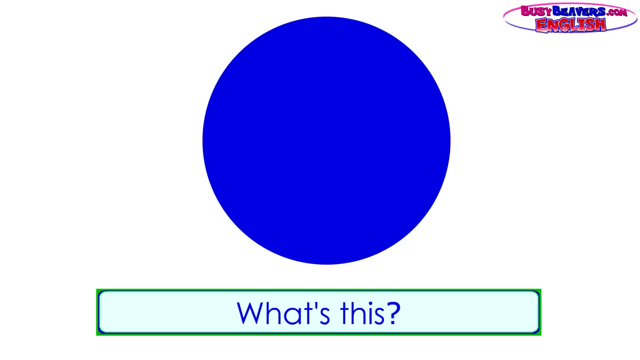 What's this? It's a heart. What's this? It's a diamond. What's this? It's a star. What's this? It's a circle. What color is the circle? The circle is blue. What's this? 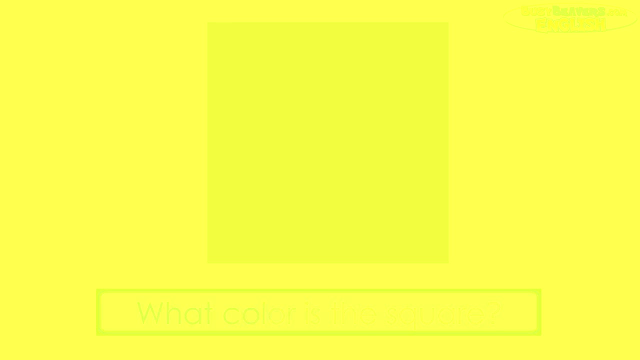 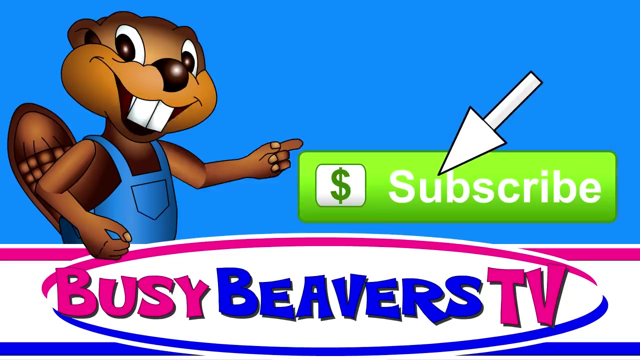 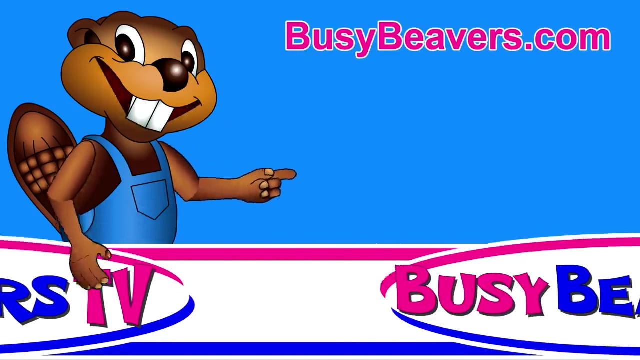 It's a square. What color is the square? This clip was a free sample. You can watch the full video by clicking this button here To become a paying subscriber to our new channel, youtubecom slash Busy Beavers TV, Or become a paying subscriber to our website, busybeaverscom. 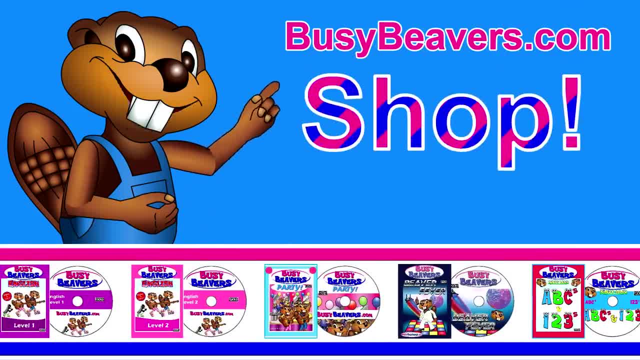 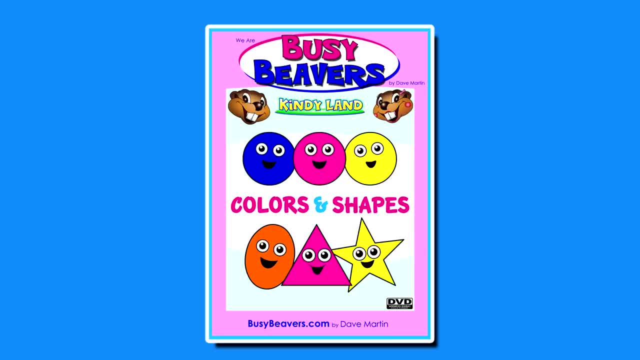 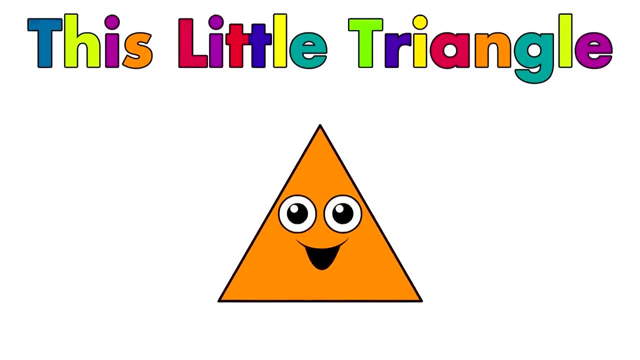 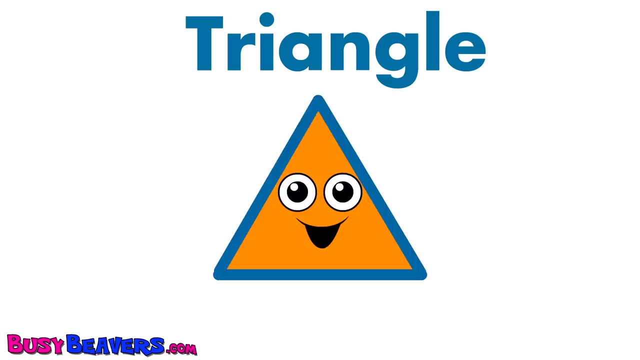 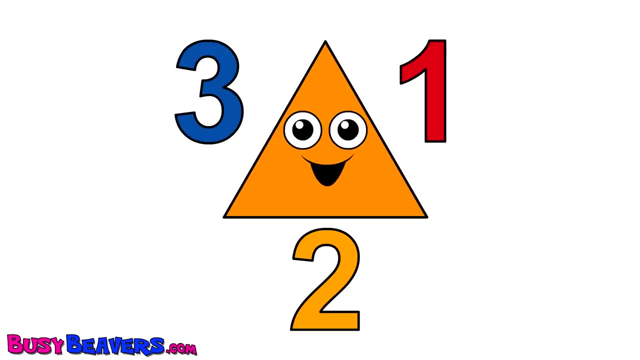 Also available on a DVD from our online shop. Okay, here we go. This little triangle has three sides. This little triangle has three sides. This little triangle has three sides: One, two, three sides. This little square has four sides. 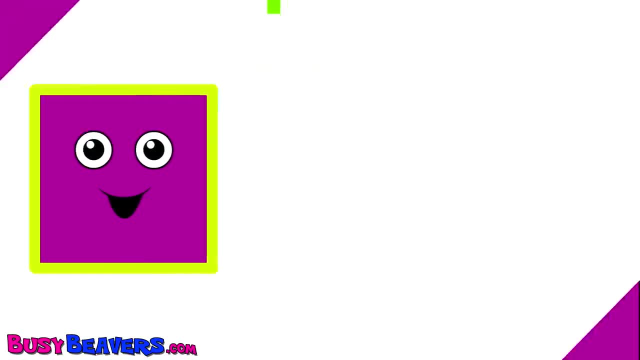 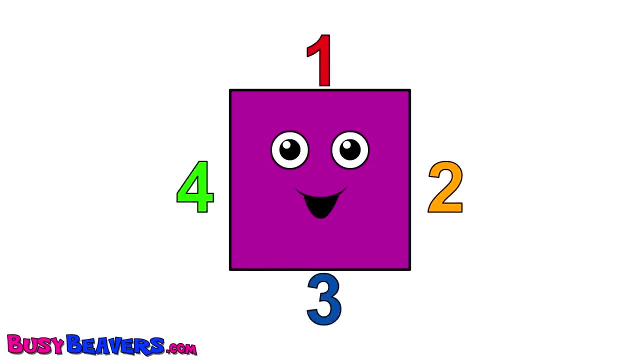 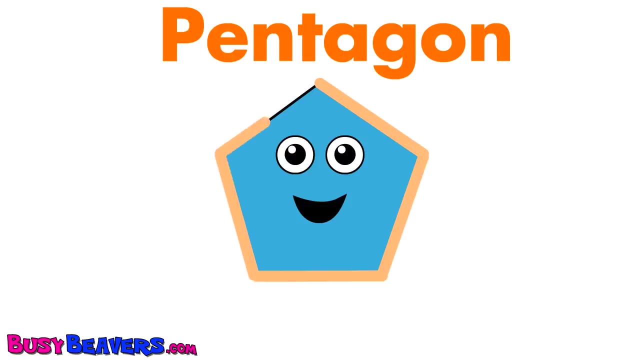 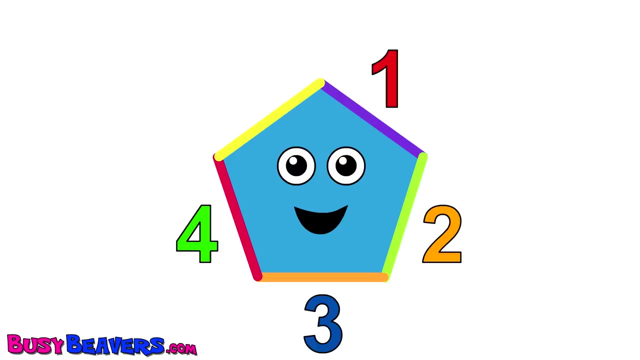 This little square has four sides. This little square has four sides: One, two, three, four sides. This little pentagon has five sides. This little pentagon has five sides. This little pentagon has five sides: One, two, three, four, five. 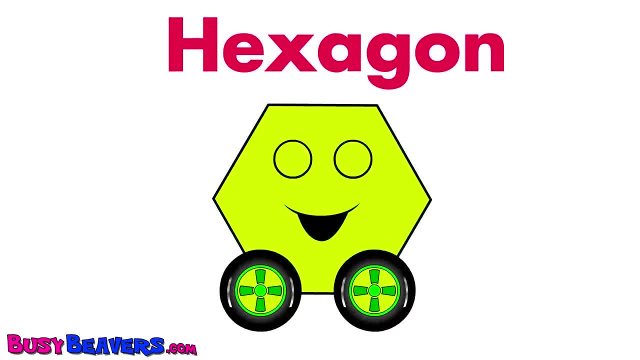 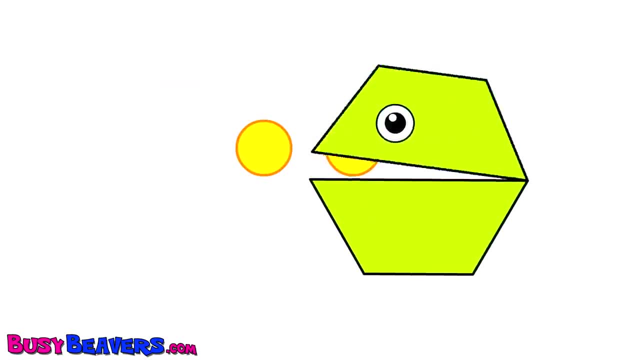 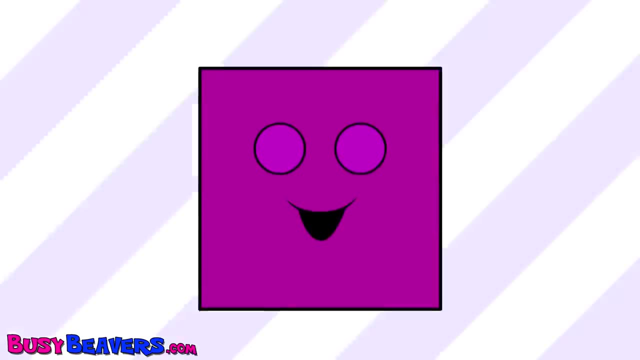 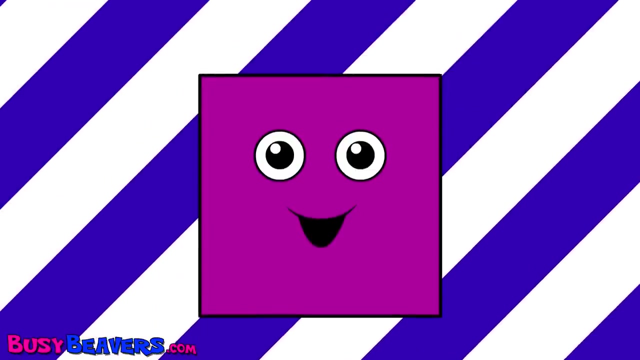 This little hexagon has six sides. This little hexagon has six sides. This little hexagon has six sides: One, two, three, four, five, six. That was pretty good, It's fun. This little heptagon has six sides. 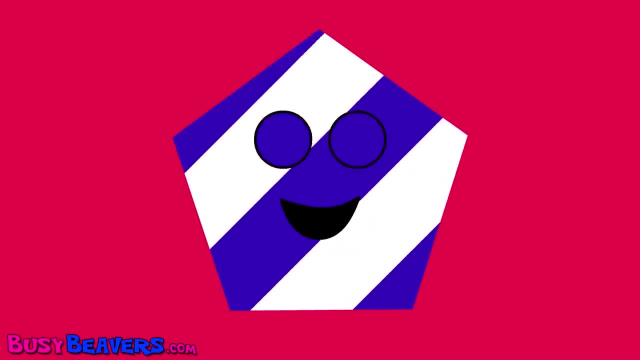 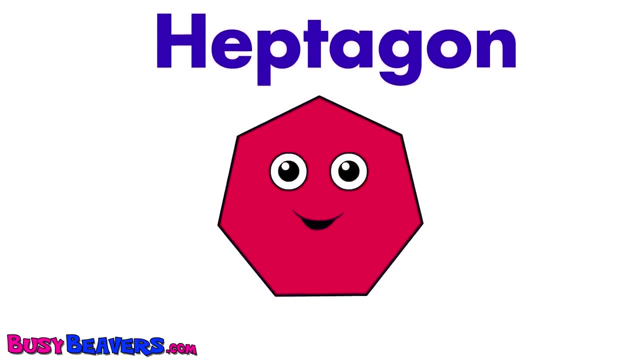 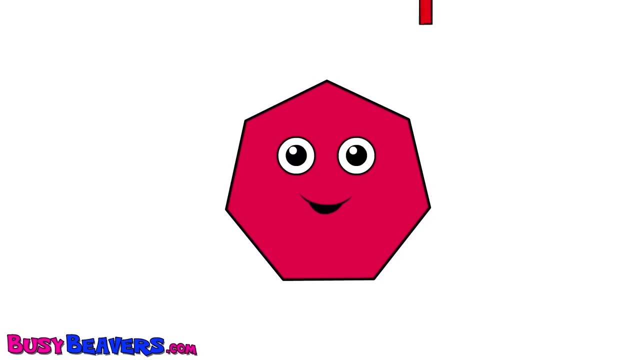 This little hexagon has six sides. This little hexagon has six sides. This little heptagon has seven sides. This little heptagon has seven sides. This little heptagon has seven sides: One, two, three, four, five, six, seven. 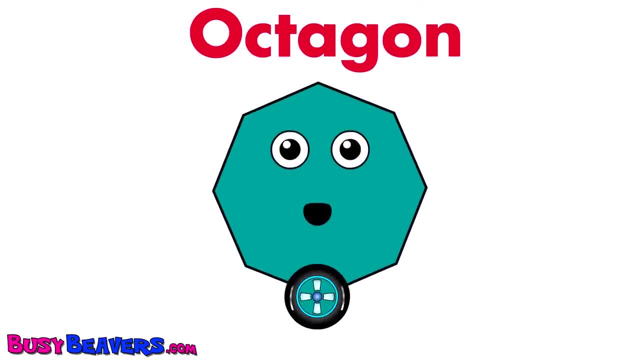 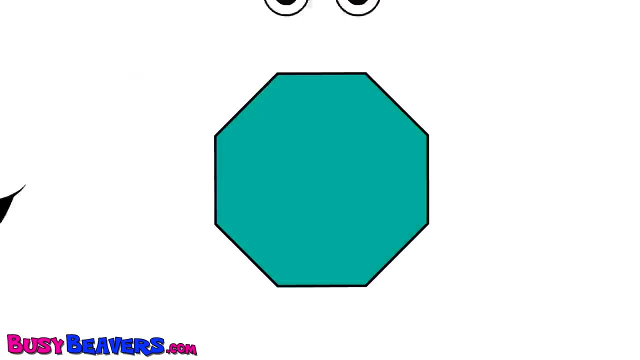 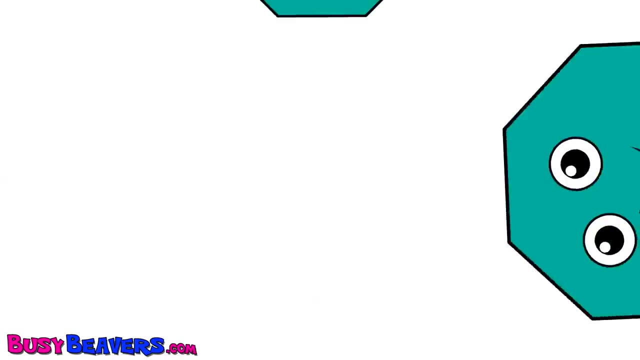 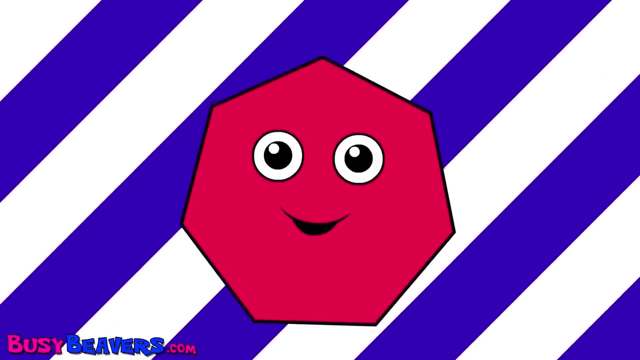 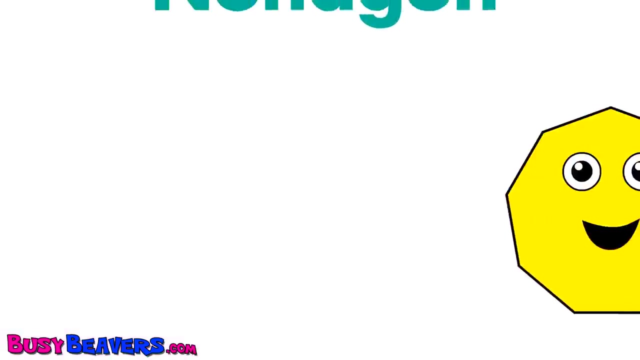 This little octagon has eight sides. This little octagon has eight sides. This little octagon has eight sides: One, two, three, four, five, six, seven, Eight. This little nonagon has nine sides. This little nonagon has nine sides. 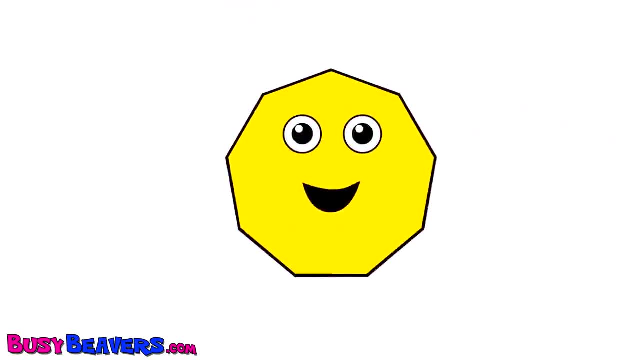 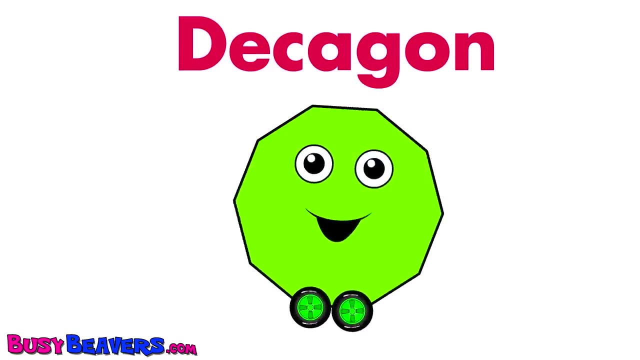 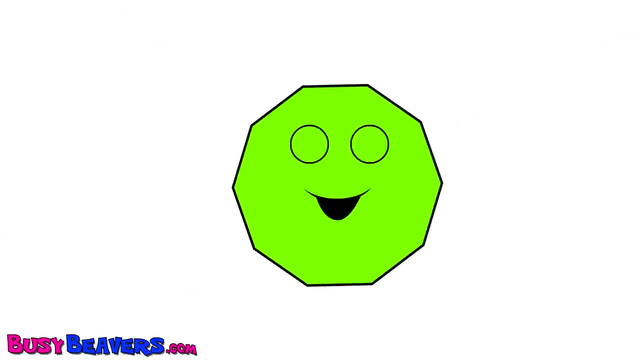 This little nonagon has nine sides: One, two, three, four, five, six, 5,, 6,, 7,, 8,, 9. This little decagon has ten sides. This little decagon has ten sides. This little decagon has ten sides. 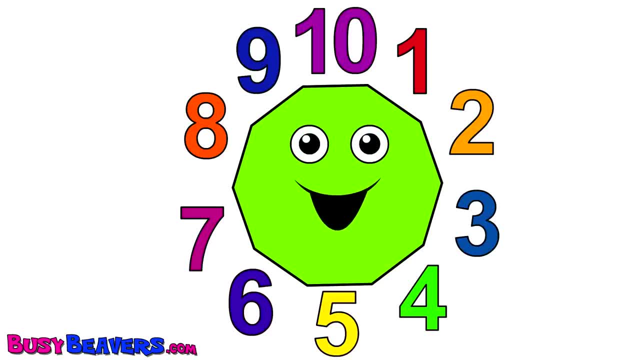 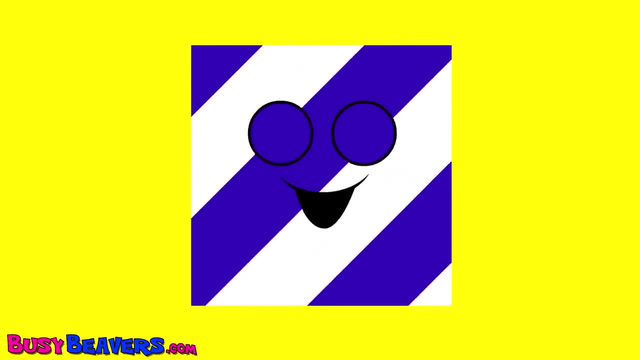 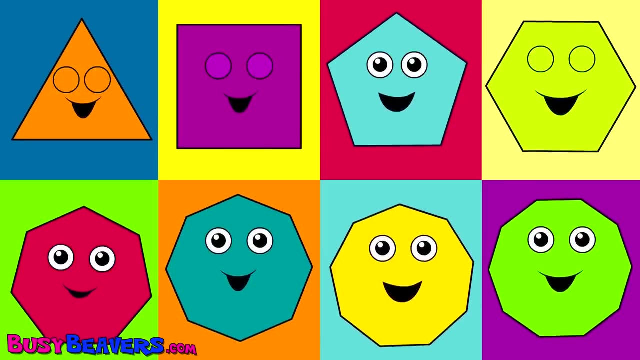 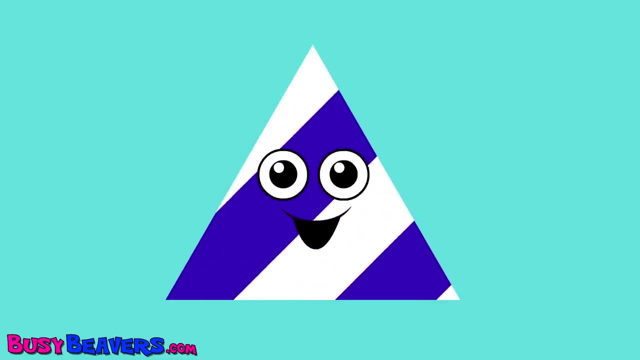 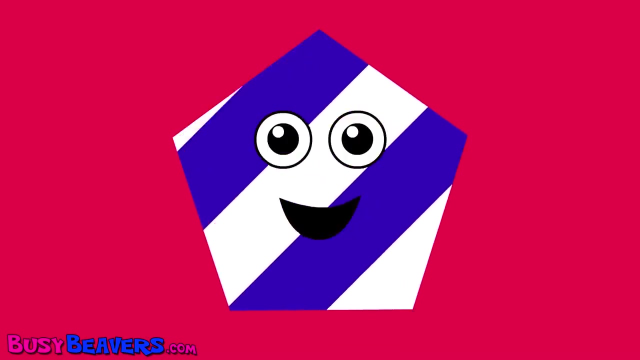 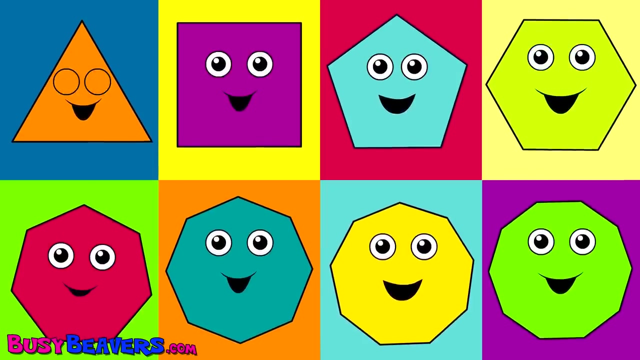 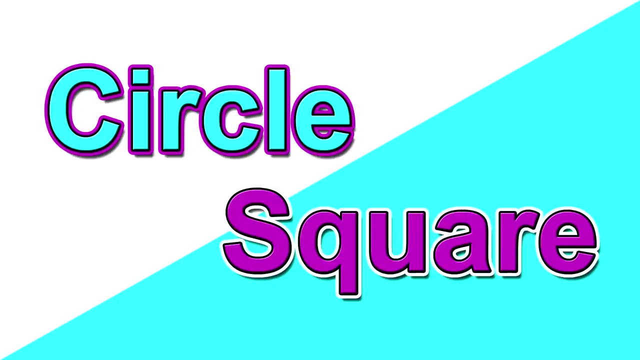 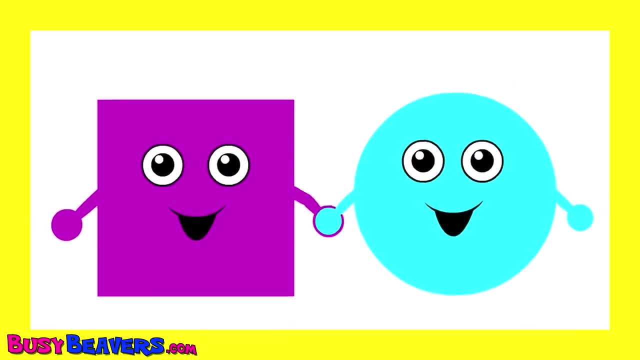 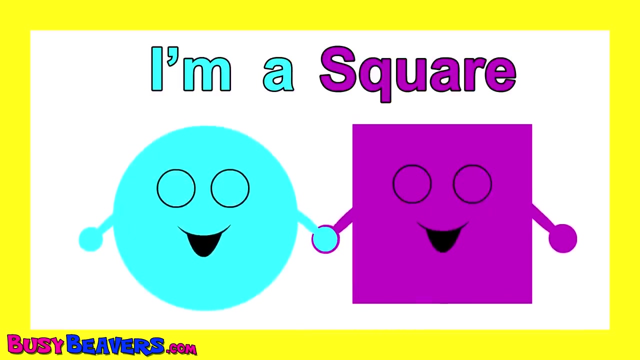 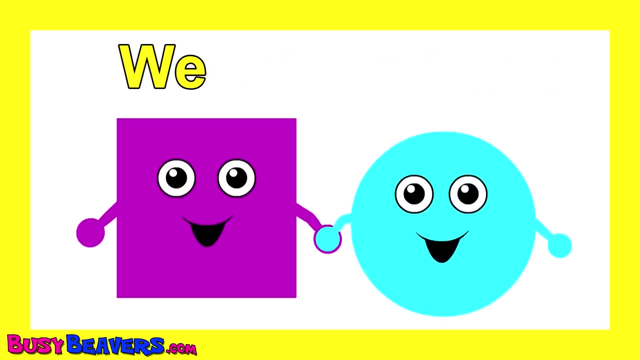 1, 2,, 3, 4, 5,, 6, 7,, 8,, 9, 10, 3, 4,, 5,, 6, 7. Thanks for watching. You're a circle, circle, circle. I'm a square. I'm a square and you're a circle. we don't. 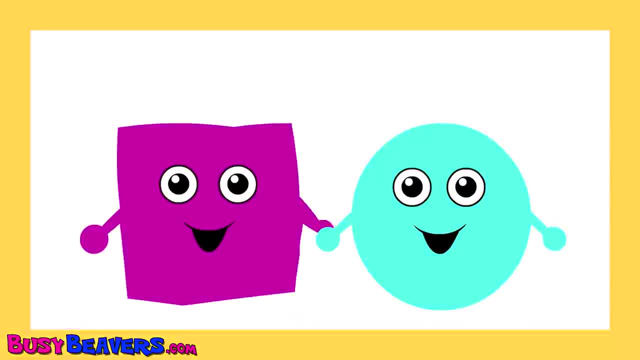 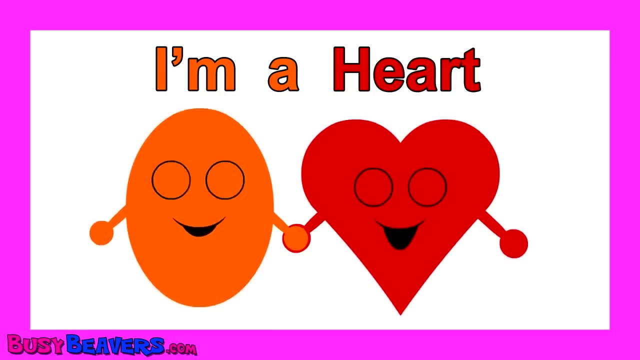 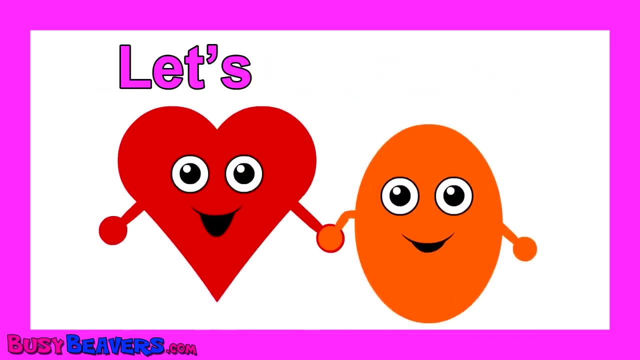 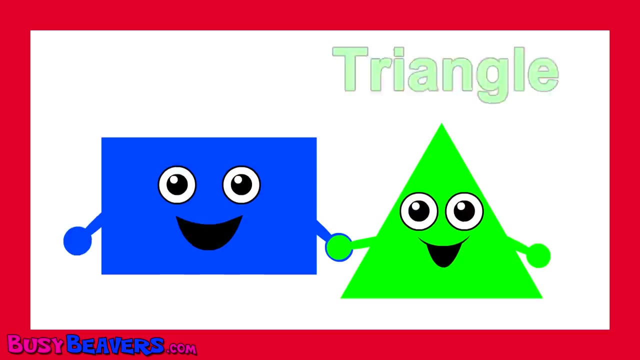 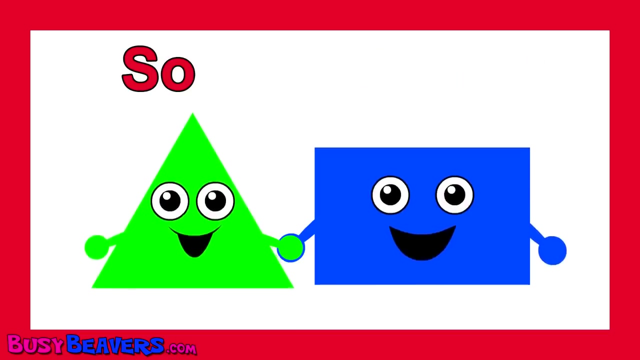 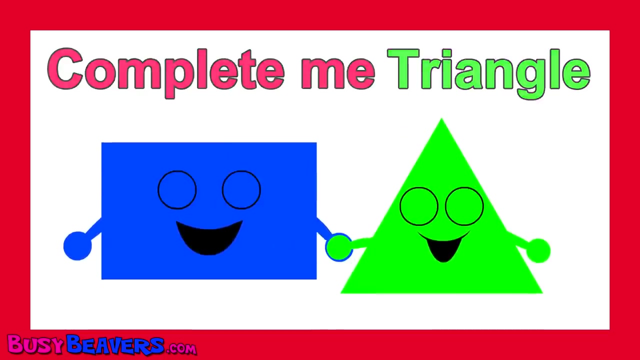 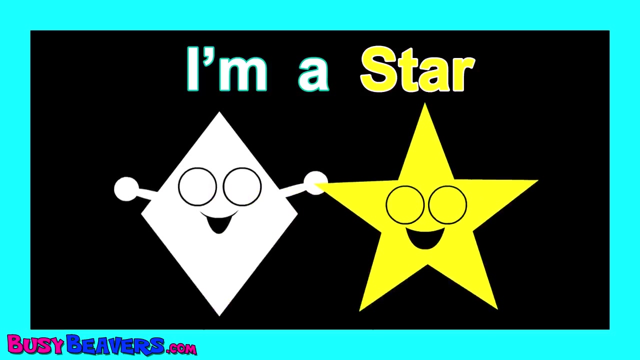 care. You're an oval, oval, oval, I'm a heart. I'm a heart, and you're an oval. let's not part. You're a triangle, triangle, triangle, I'm a rectangle. So neatly you complete me. triangle, You're a diamond, diamond, diamond, I'm a star. 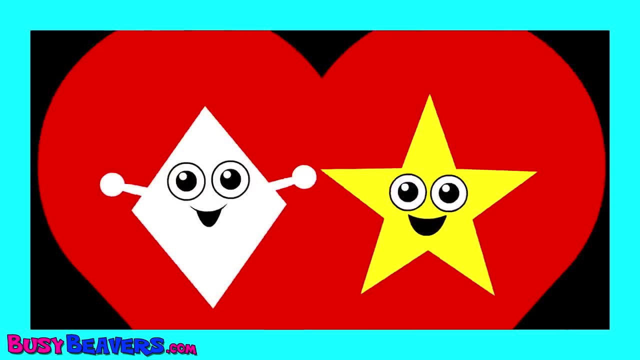 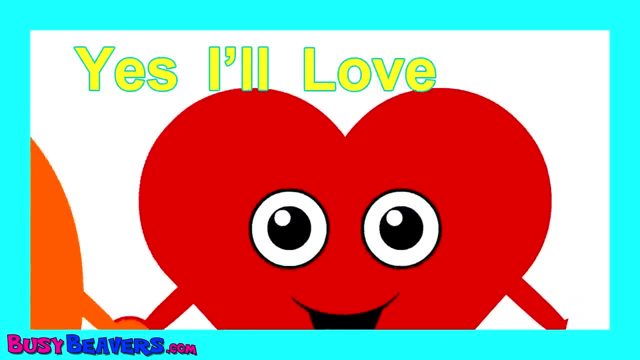 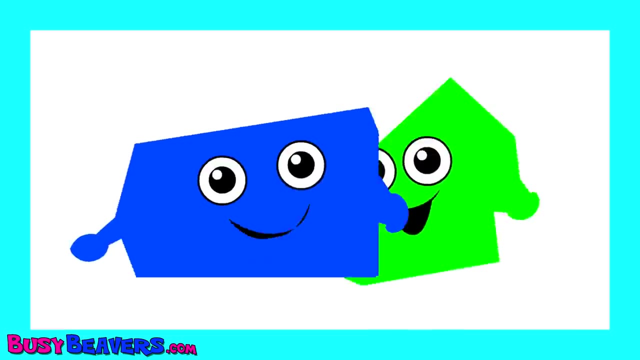 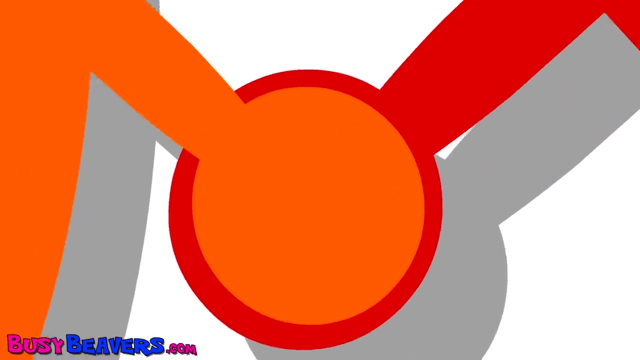 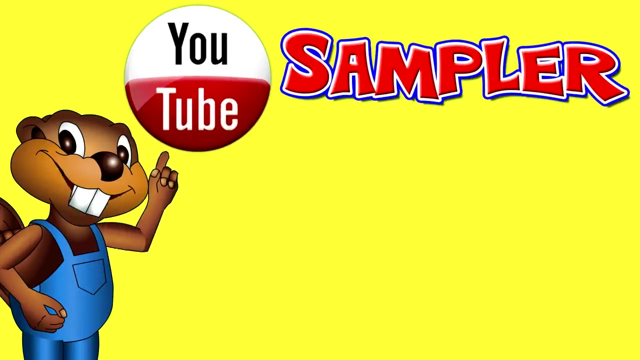 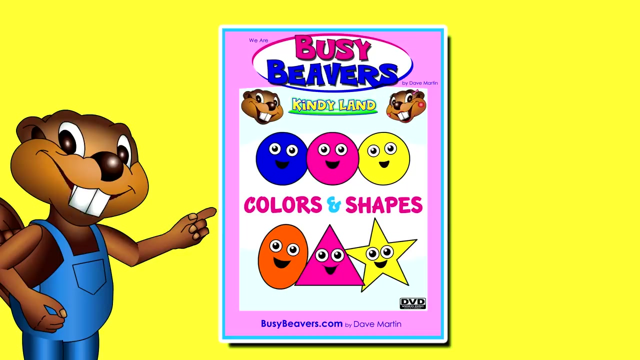 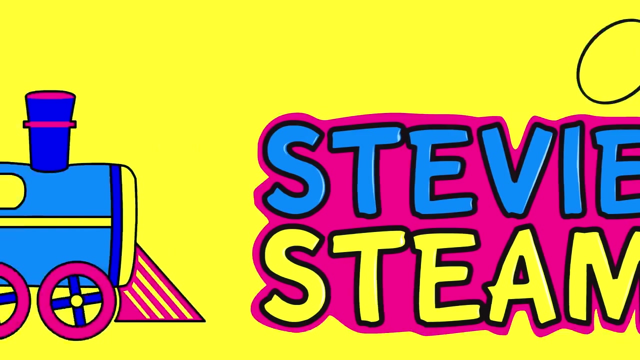 But I'll love you, love you, love you, whatever you are. I'm a star. Yes, I'll love you, love you, love you, whatever you are, I'll love you, love you, love you, whatever you are. Stevie Steamer, that's my name. 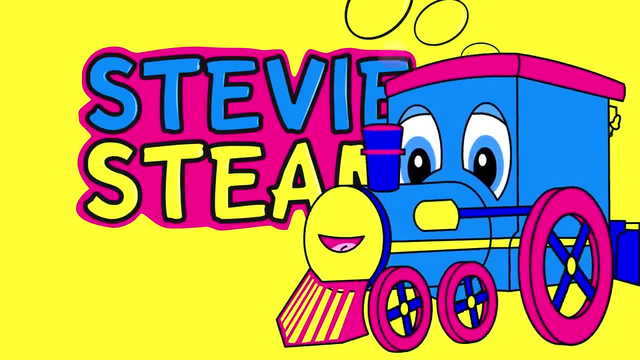 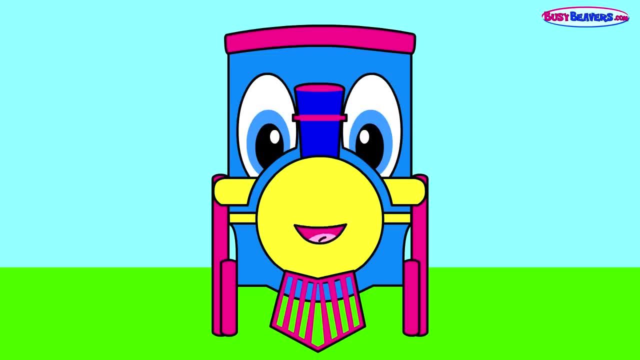 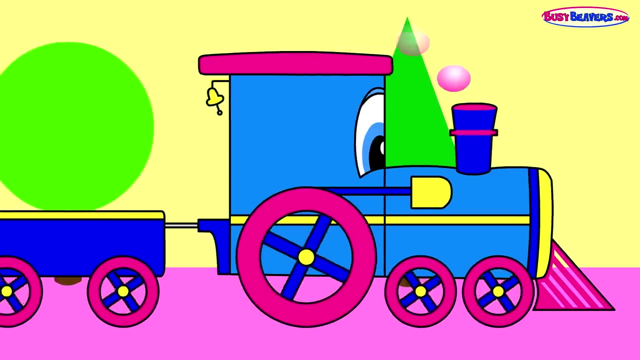 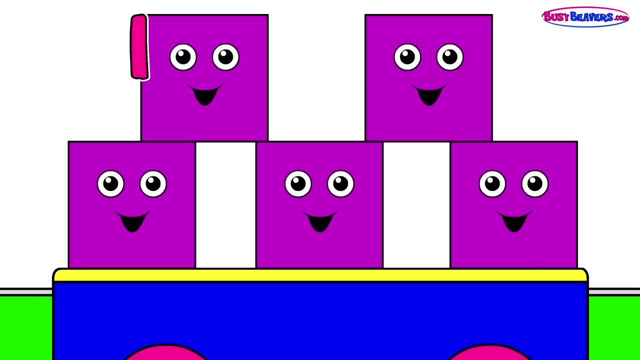 Stevie Steamer, I'm a train. Hello, I'm Stevie Steamer, I'm a train. Today I'm pulling some more shapes. Let's go say hi to the shapes and count them: Squares: One, two, three, four, five. 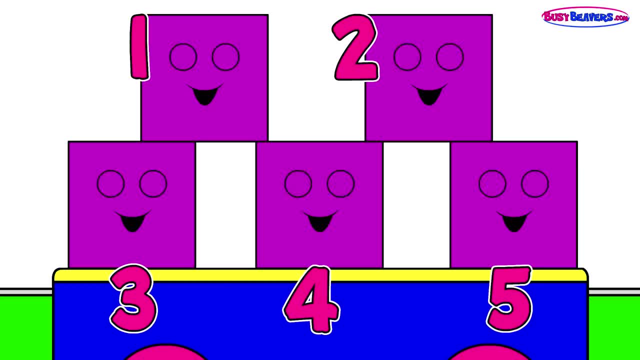 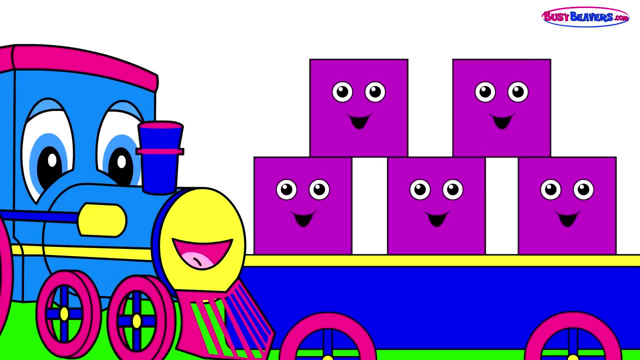 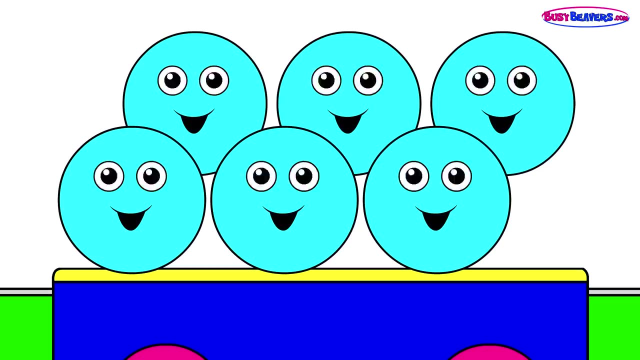 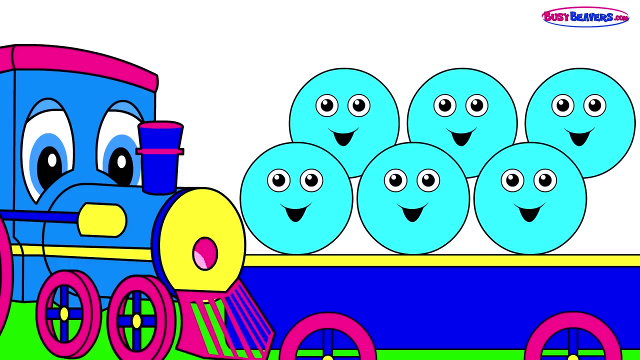 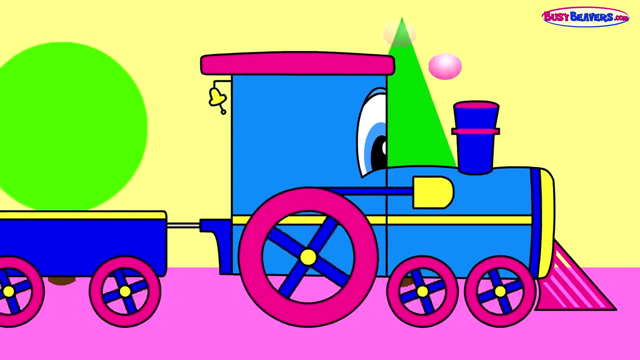 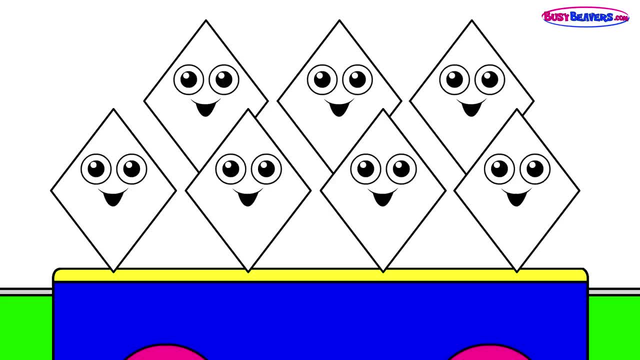 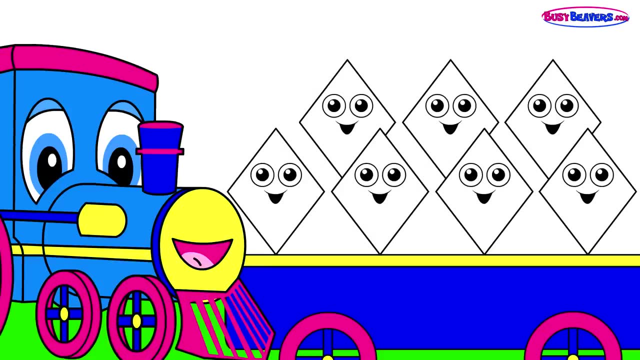 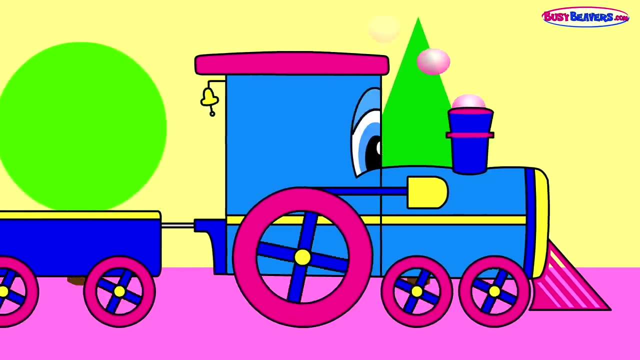 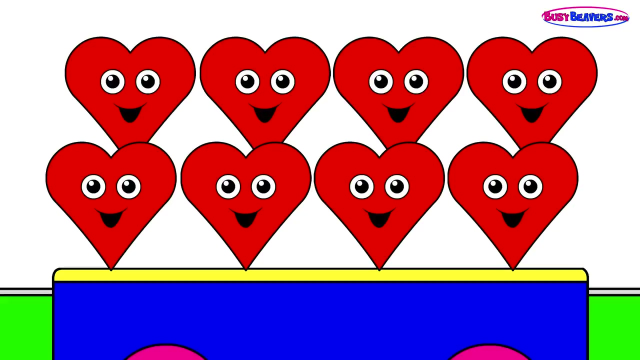 Six, Six, Six, Six, Six, Six, Six, Seven, Eight, Seven, Eight, Nine, Ten, 24, Five, Four, Three, Two, One, Two, One Two One Two, Three, Three, Four, Five, Six, Six, Seven, Seven, Seven Diamonds, Hi diamonds, Hi Stevie, Four, five, six, seven, eight. 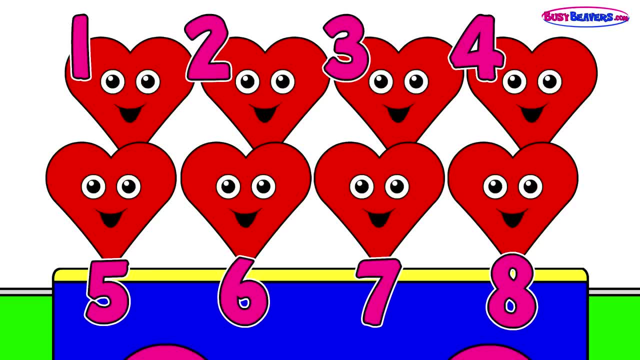 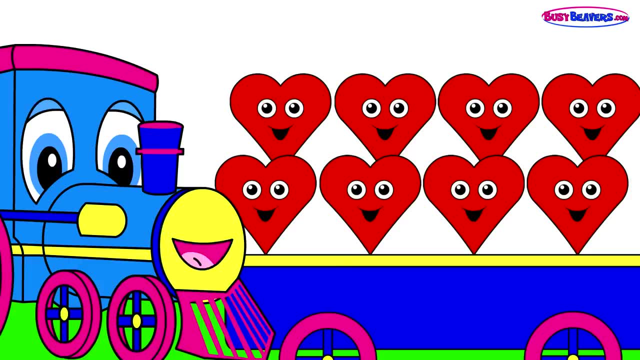 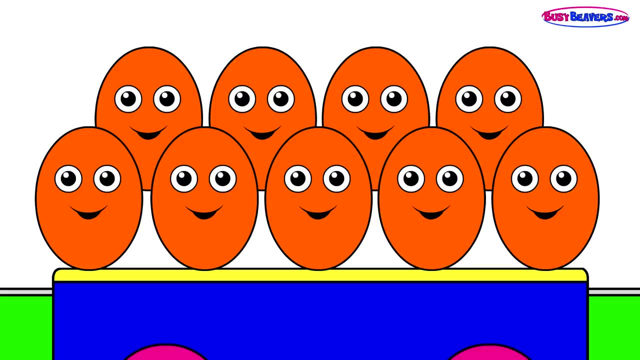 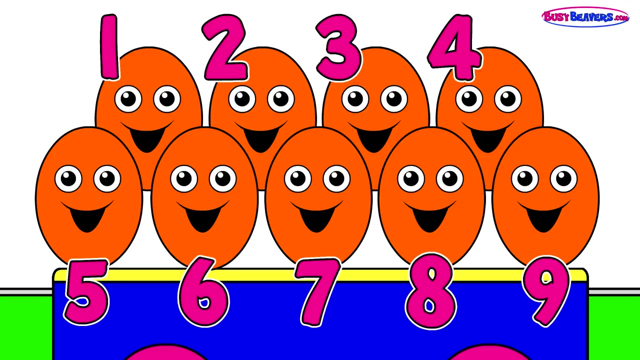 Eight hearts, Hello hearts, Hello, Hey, how you doing Hearts, I love them. Ovals One, two, three, four, five, six, seven, eight, nine, Nine ovals, Hi ovals. 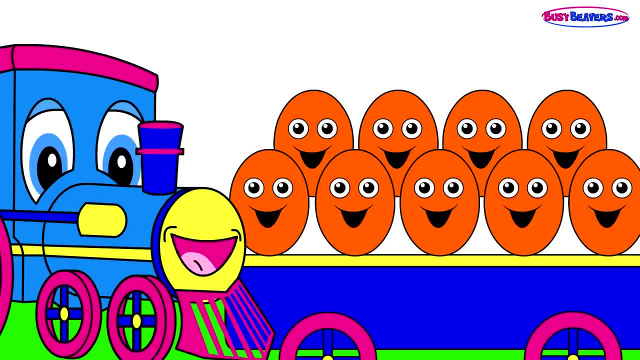 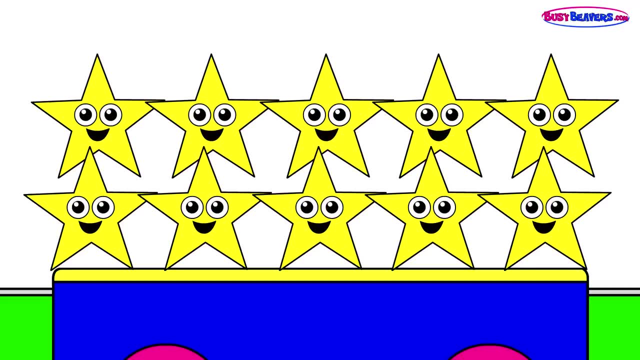 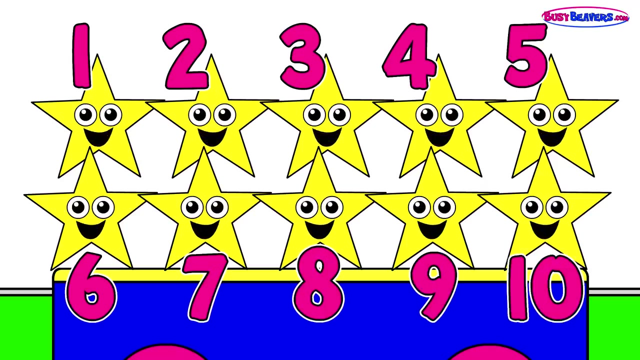 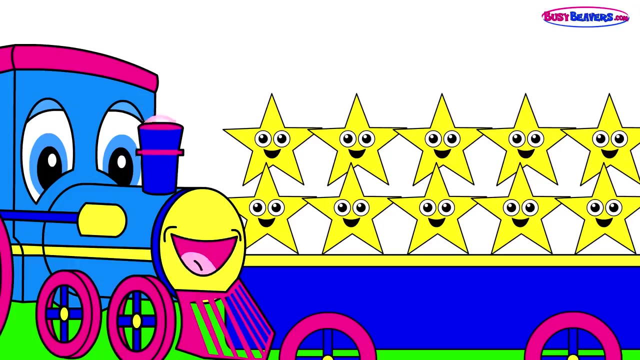 Hi Steamy Steamer, So round: Stars One, two, three, four, five, six, seven, eight, nine, ten, Ten stars Hi, stars Hi Steamy, Very sparkly, Very twinkly. 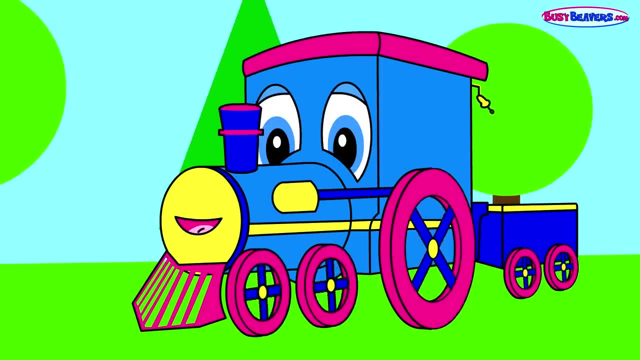 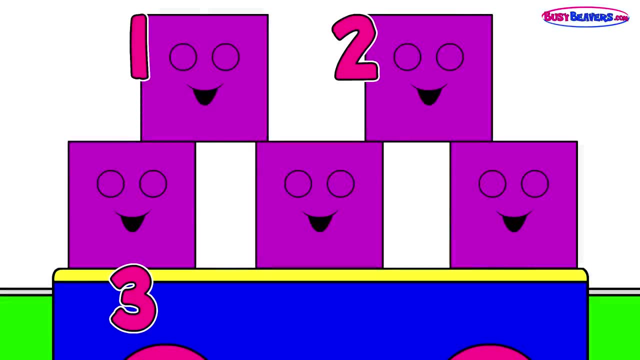 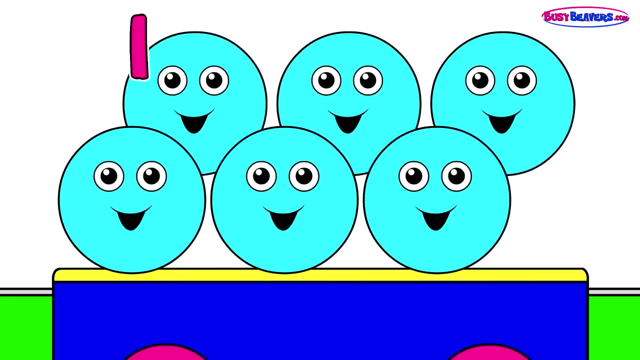 Well, that's all the shapes For today. let's count them one more time: One, two, three, four, five squares: One, two, three, four, five, six circles: One, two, three, four, five, six circles. 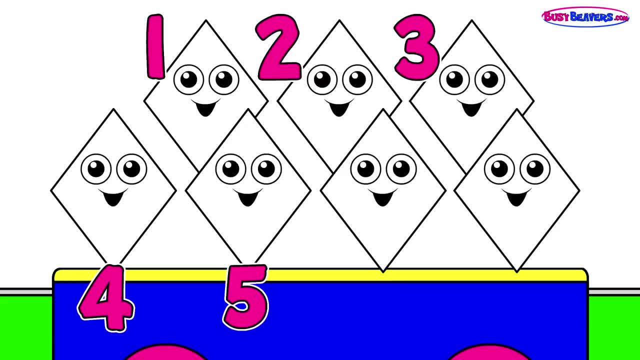 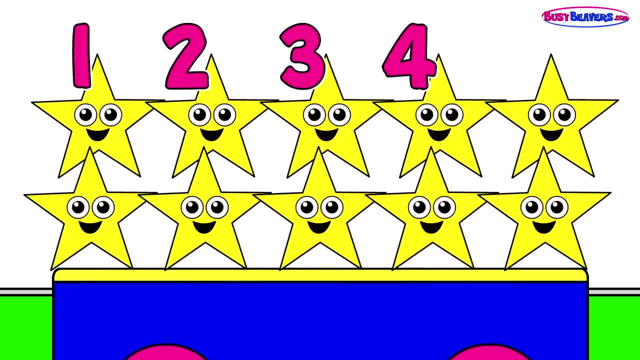 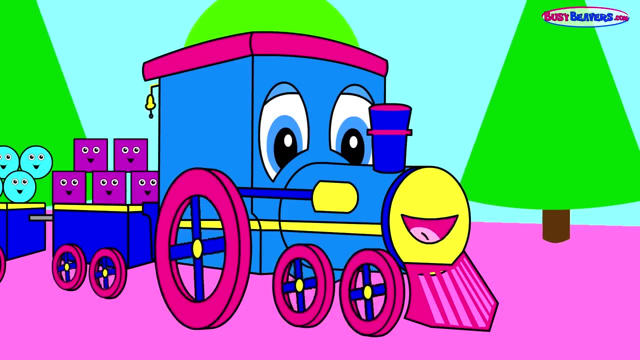 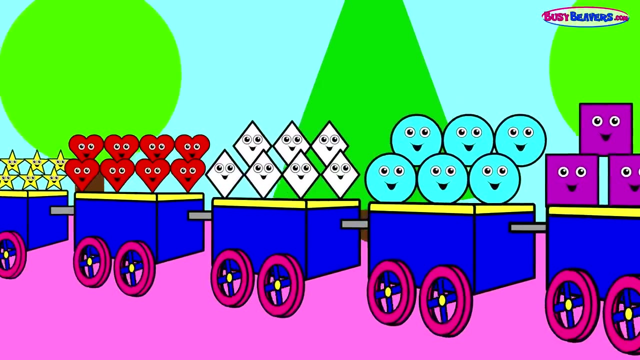 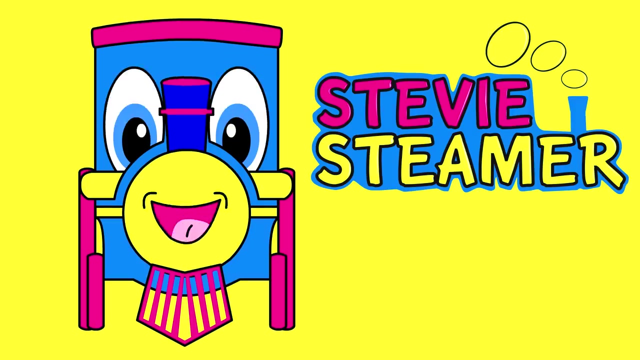 One, two, three, four, five, six, seven, eight, nine, 10 stars All aboard, Here we go. Steamy steamer, Steamy steamer, That's my name. Stevie Steamer, I'm a train. 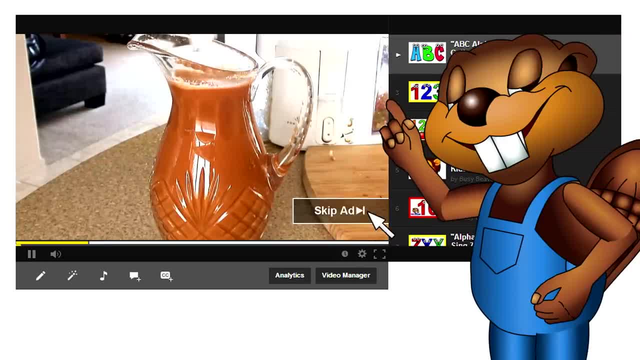 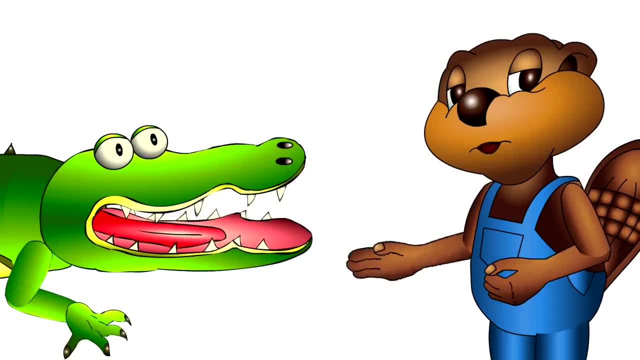 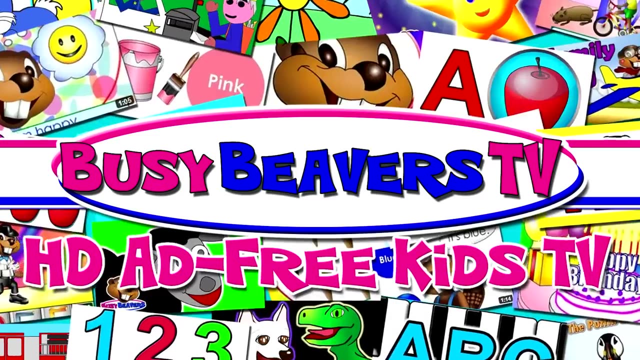 Skip ad, Skip ad, Are you tired of watching ads before every video on YouTube? Oh, they're very frustrating. I know Well, Busy Beavers have a new channel, Busy Beavers TV, Where all of our kids' learning videos are in HD and ad-free. 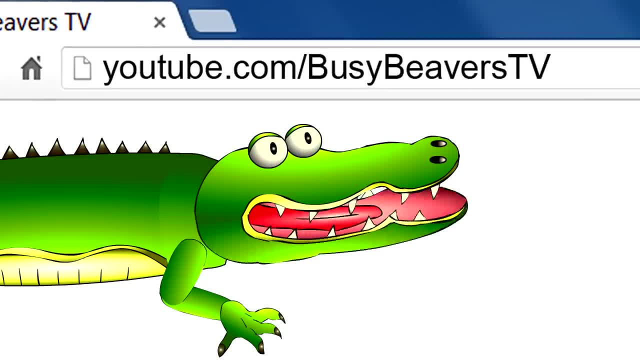 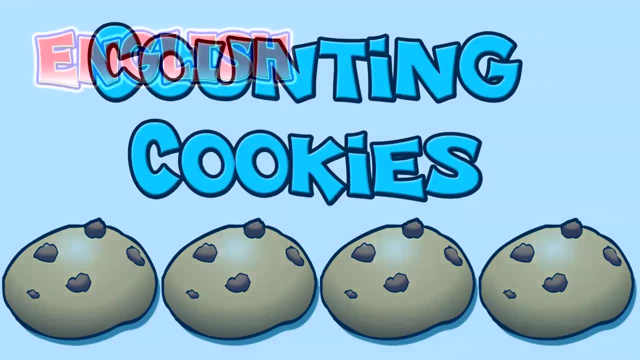 So let me get this straight. YouTubecom slash Busy Beavers TV has all of the Busy Beavers song videos, Yeah, And all of the kindy lesson videos. That's right, And I can learn to speak English, Chinese, Korean, Spanish and more. 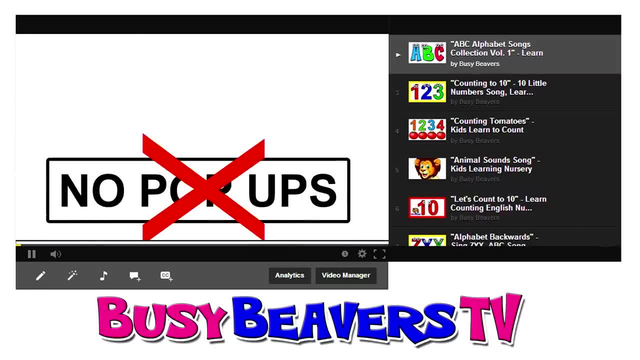 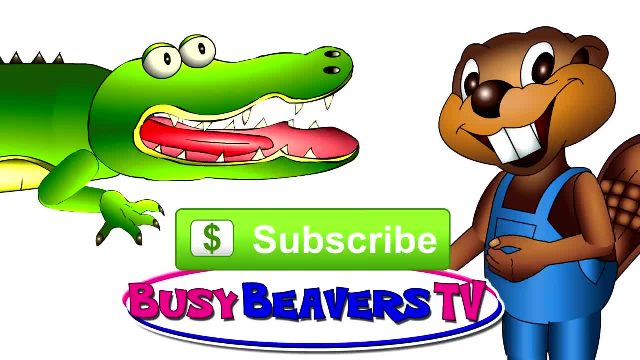 Yes, And there's no ads. No ads, No pop-ups, No pop-ups And no commercials. All of the great content from our free channel in HD and ad-free. That's it. I'm clicking on it. I'm clicking that button. 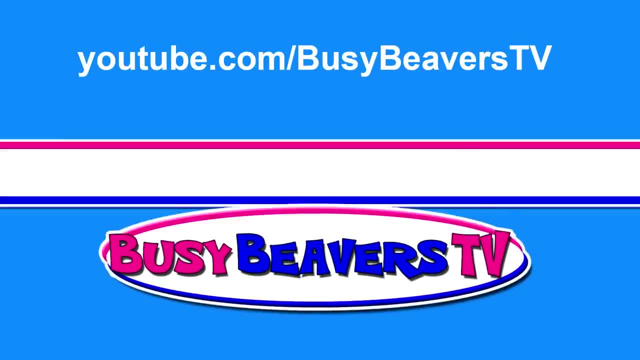 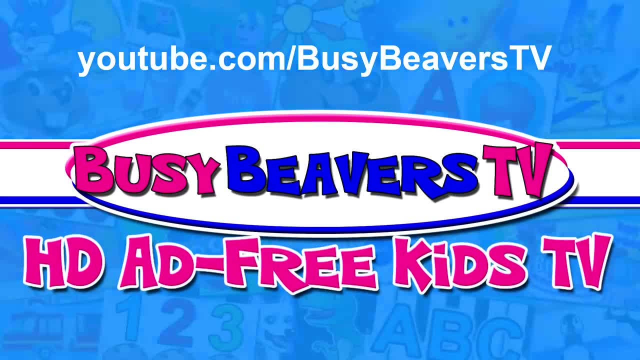 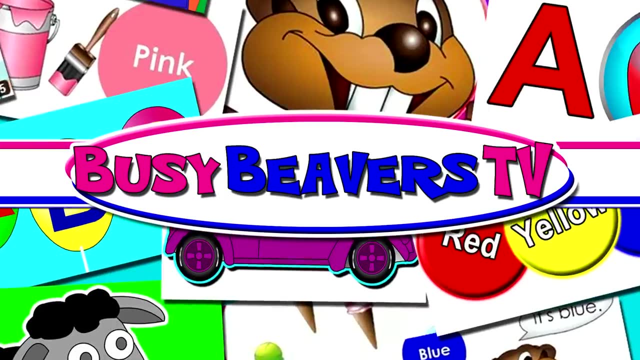 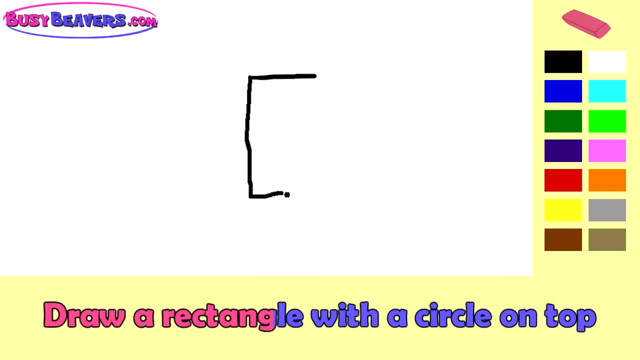 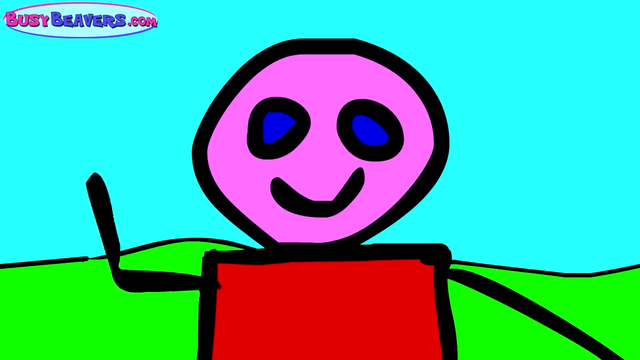 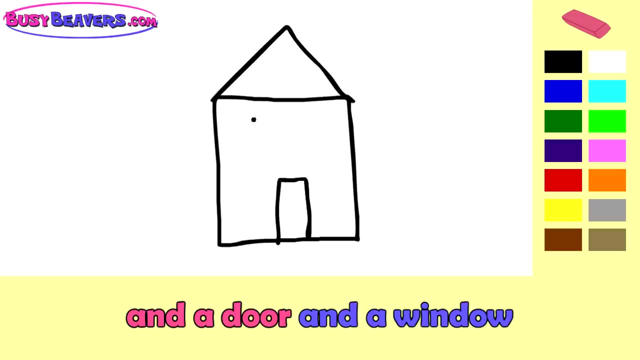 And I'm not kidding, Do it. YouTubecom slash Busy Beavers TV For kids' learning videos in HD and ad-free. And all of the kindy lesson videos- Yeah, And all of the kindy lesson videos in HD and ad-free. 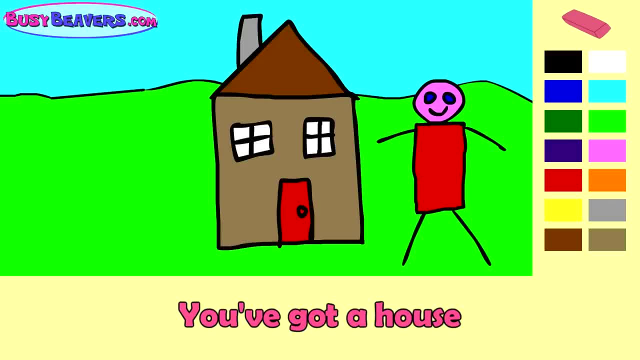 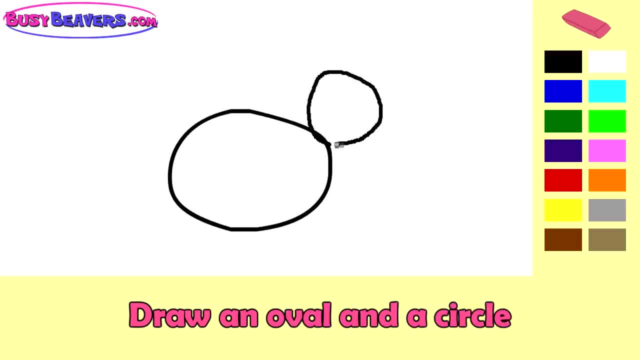 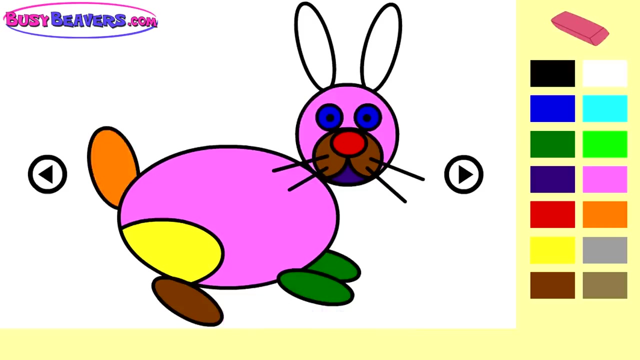 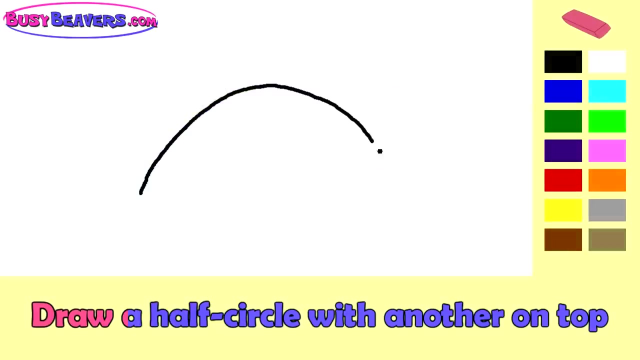 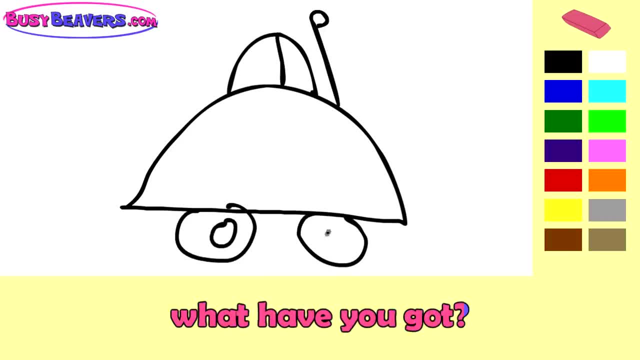 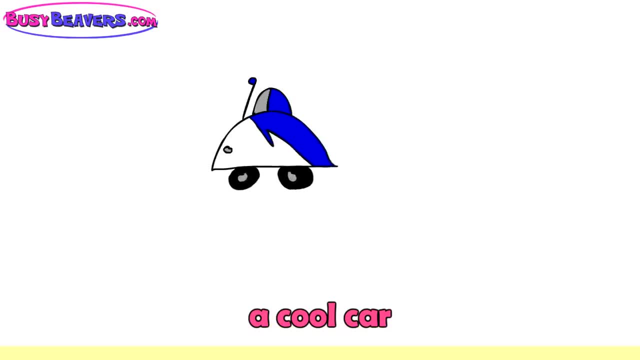 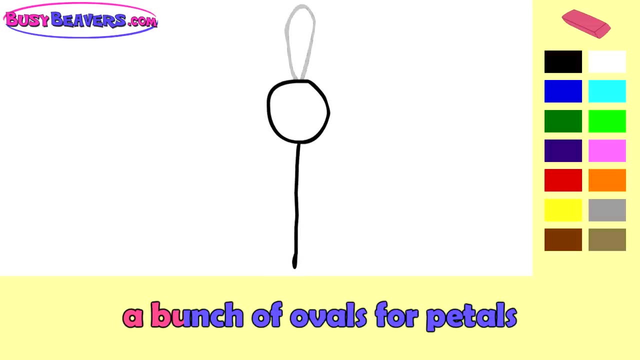 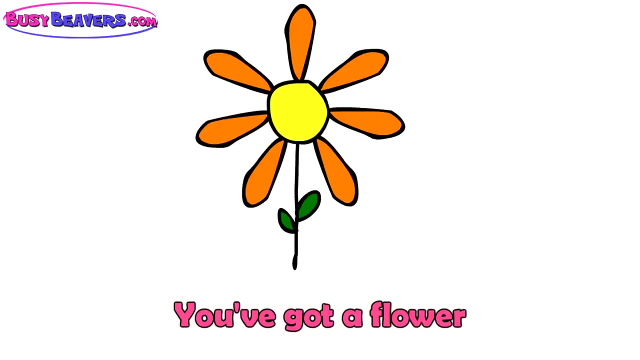 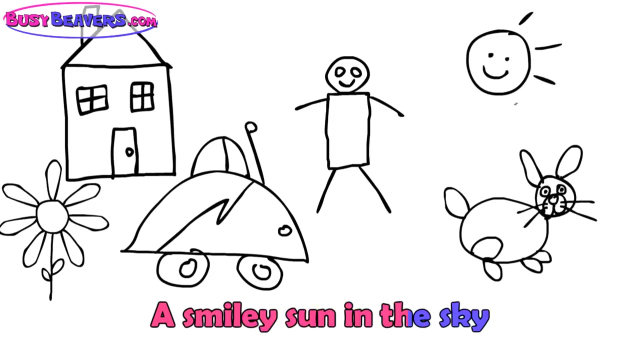 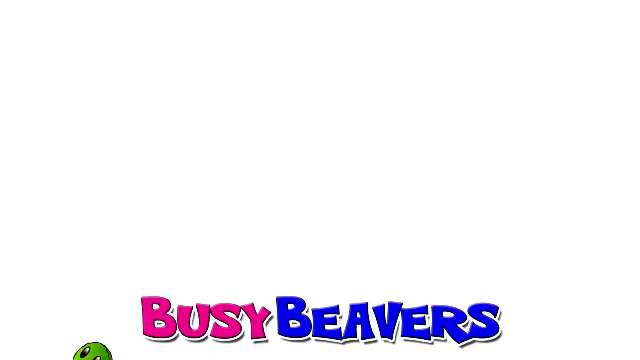 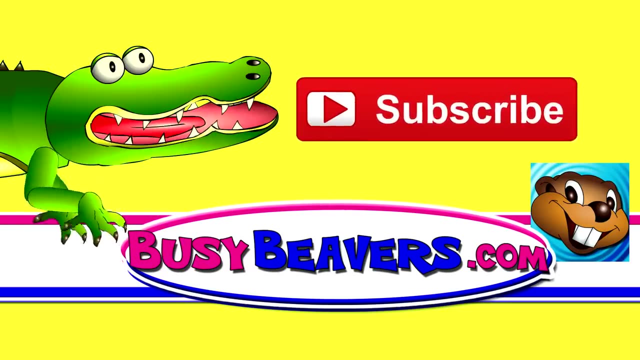 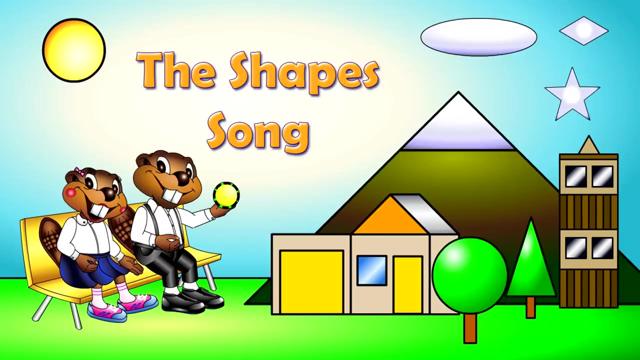 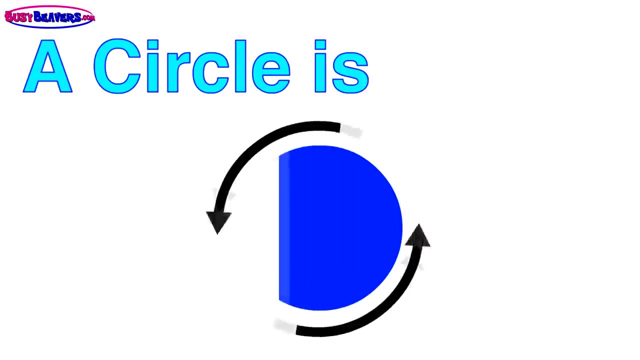 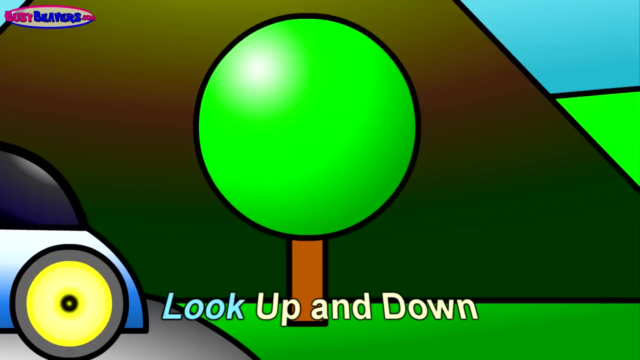 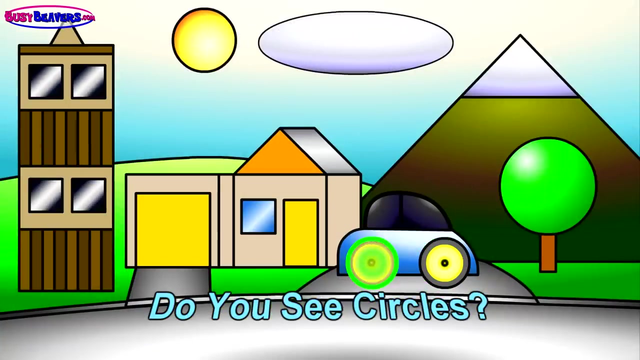 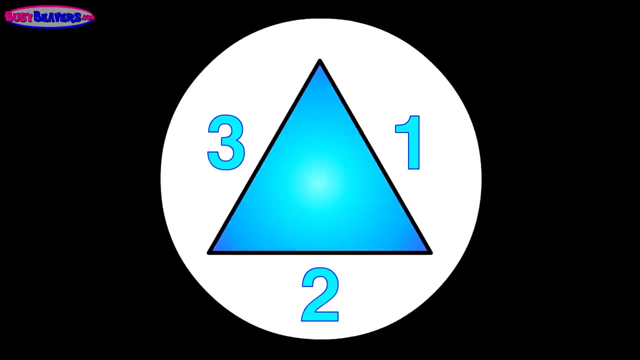 It's a circle, it's a circle. a circle is round. It's a circle, it's a circle, a circle is round. Look up and down, look all around. do you see circles? Triangle triangle one, two, three. Triangle triangle one, two, three. 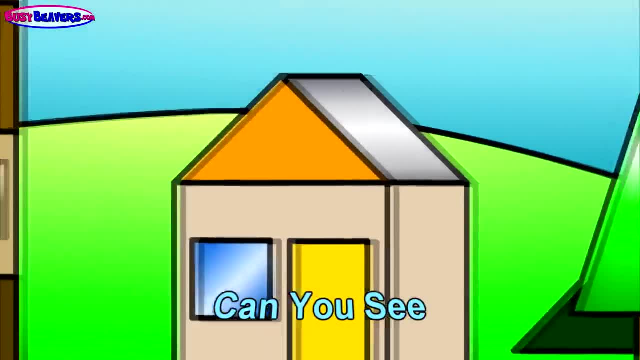 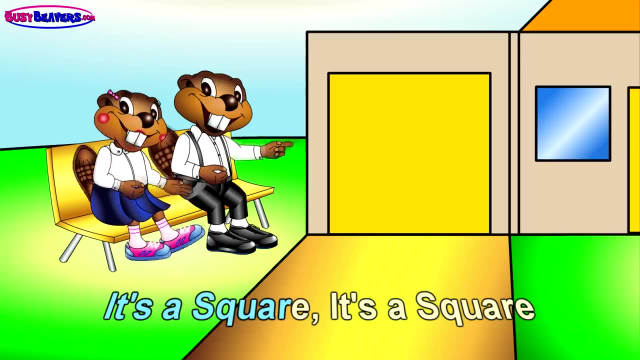 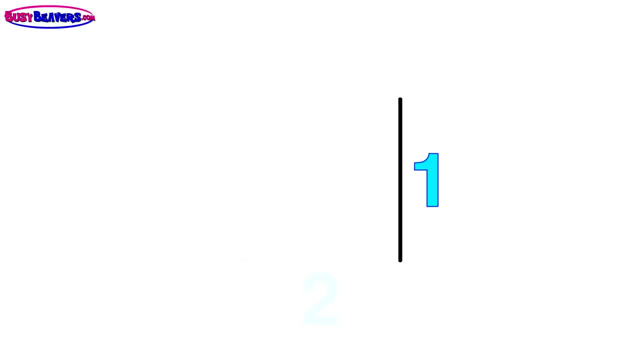 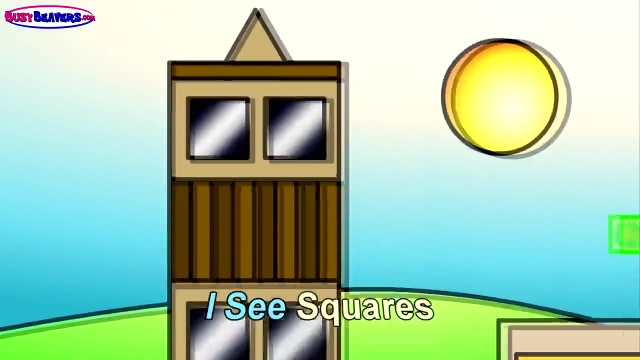 Look all around you, can you see triangles. It's a square. it's a square. one, two, three, four. It's a square. it's a square. one, two, three, four. Look over there, can you see squares? I see squares. 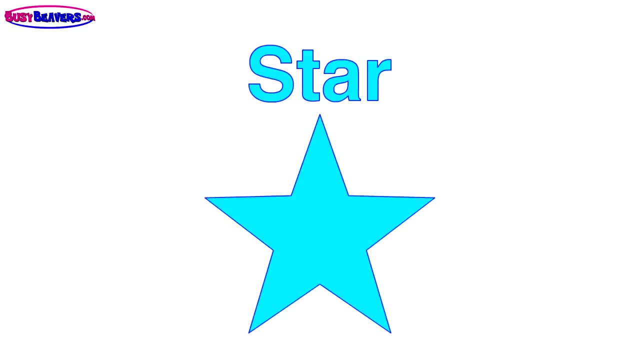 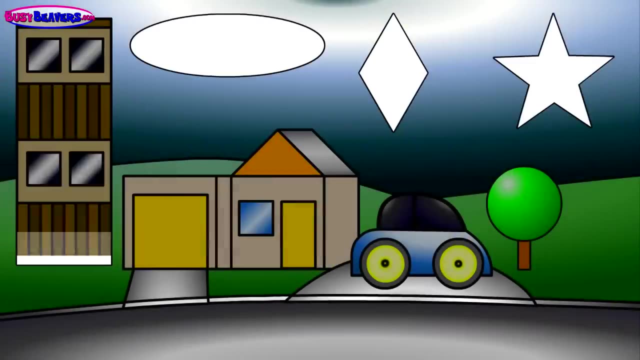 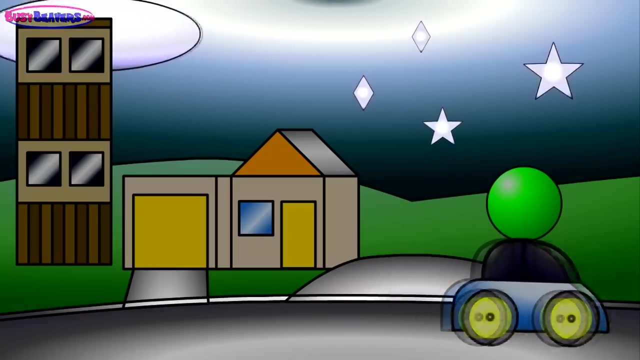 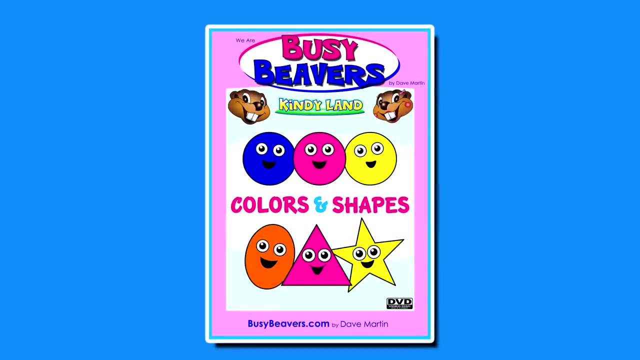 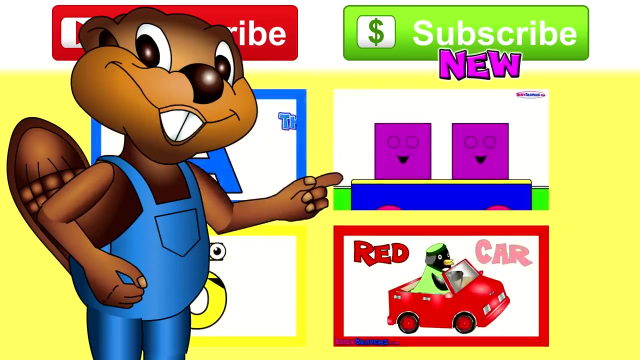 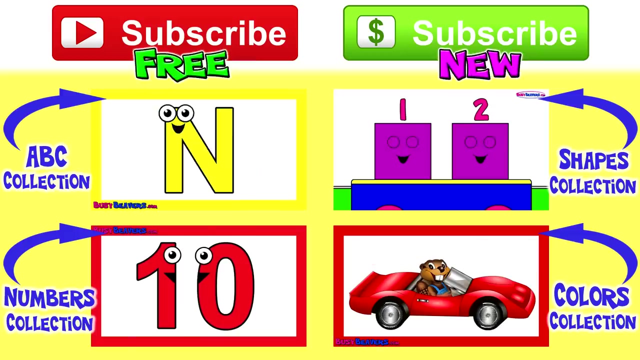 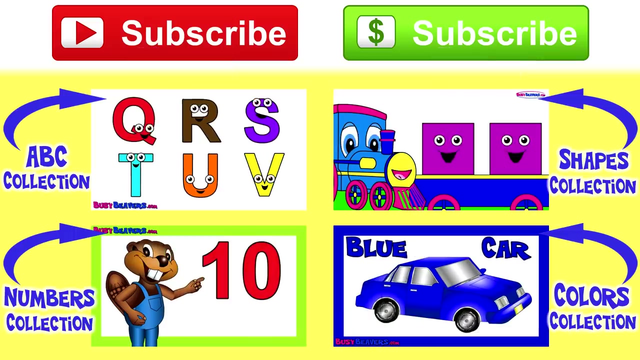 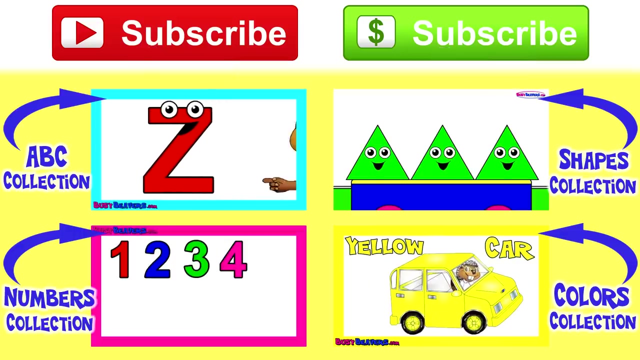 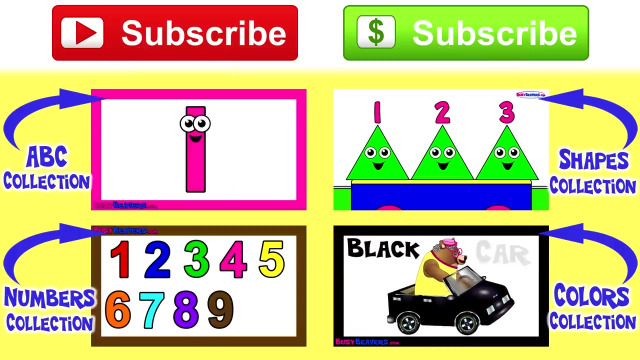 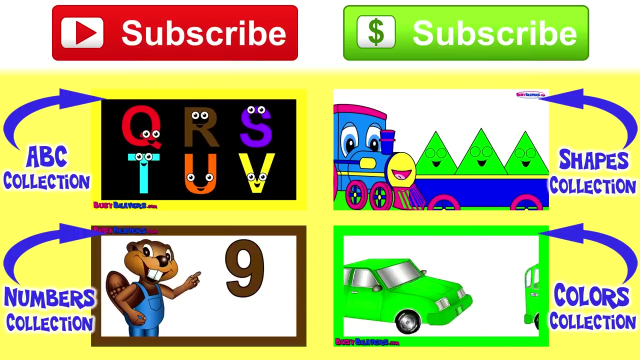 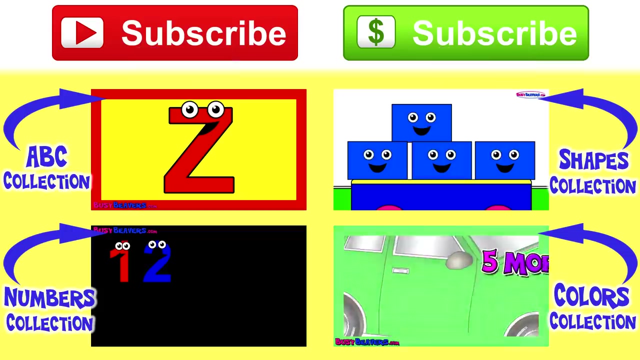 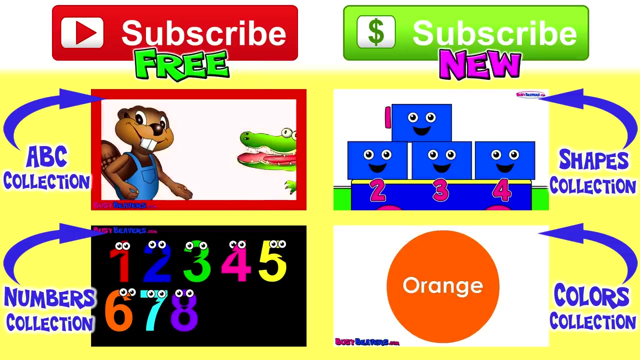 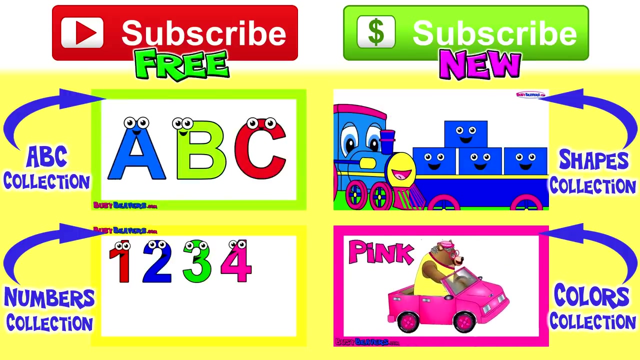 Rectangle over diamond star. Rectangle over diamond star. Rectangle over diamond star Rectangle. Subscribe to our channels to keep in touch And check out these other cool Busy Beavers videos. Thank you, You're welcome.